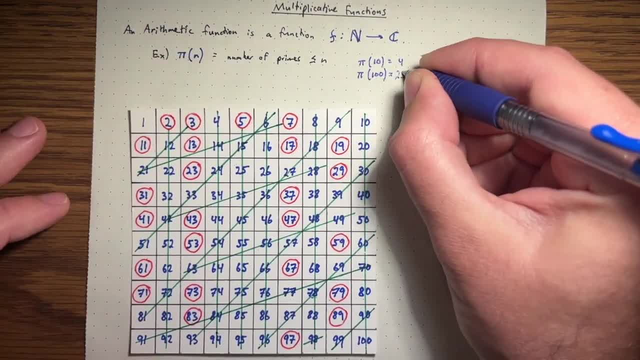 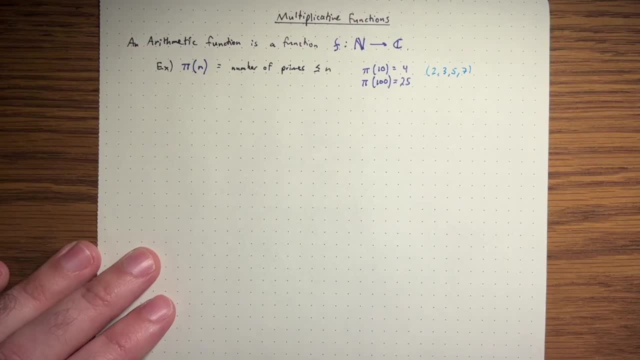 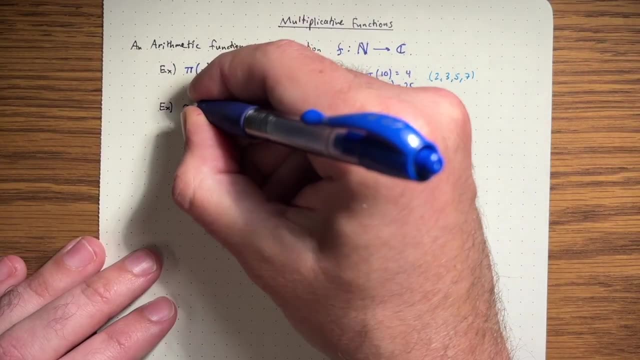 If you count them all, you should get 25.. So that's one example of an arithmetic function. Another example Is the function that counts the divisors of a number. So this is called tau of n. This is the Greek letter tau. 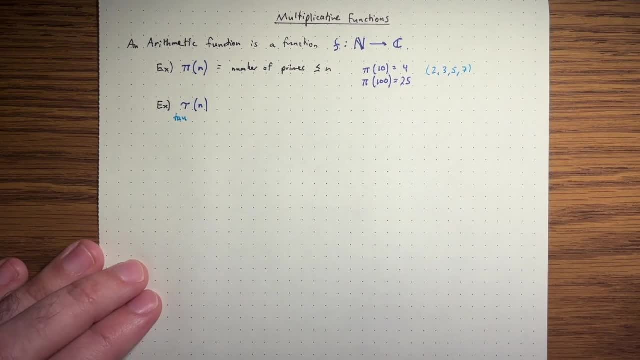 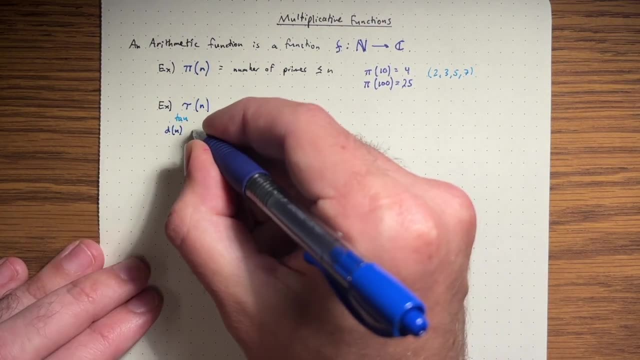 I'm pretty sure this comes from the German word for divisor, which starts with a T, But often this function also has some other names. So some people call it d of n, Some people call it sigma 0 of n. I'll explain that a bit more later. 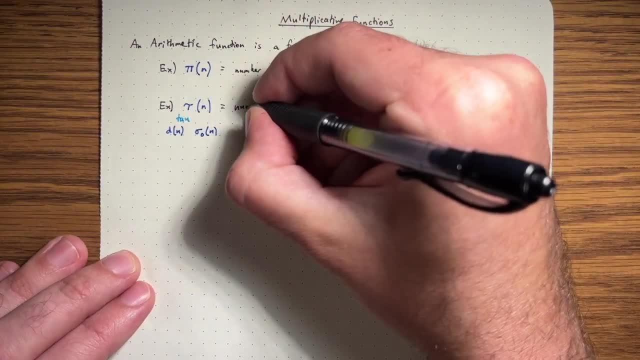 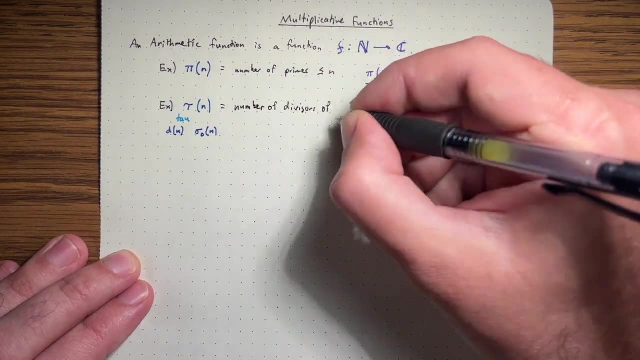 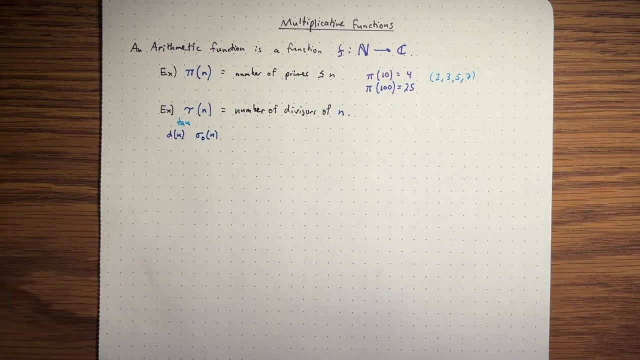 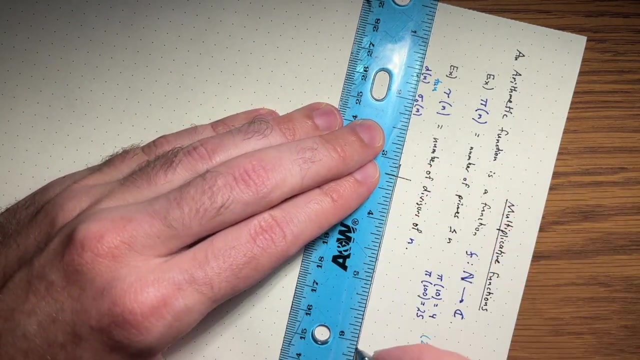 But yeah, what is this function? It just counts the number of divisors of n. So it's the number of divisors of this number, n, And I think this one's worth making a little table actually. So this one we're going to study a fair bit today. 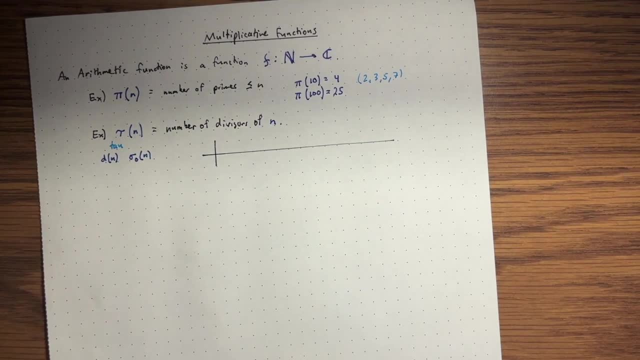 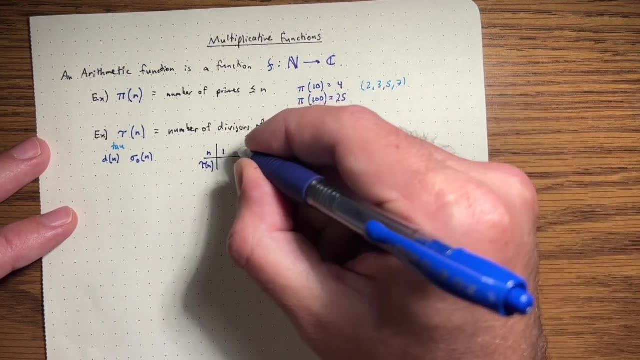 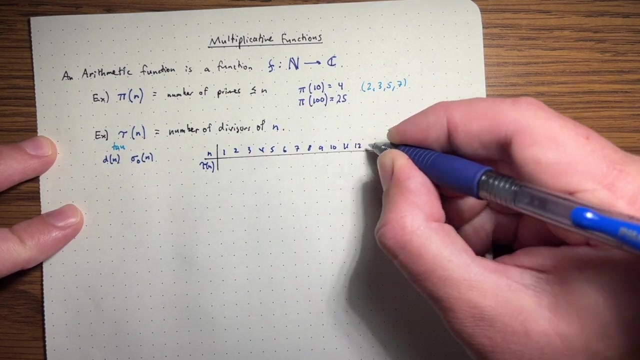 Because it turns out this function has some rather nice properties. So let's put n up here and then tau of n down here. So n is going to start at 1,, 2,, 3,, 4,, 5,, etc. 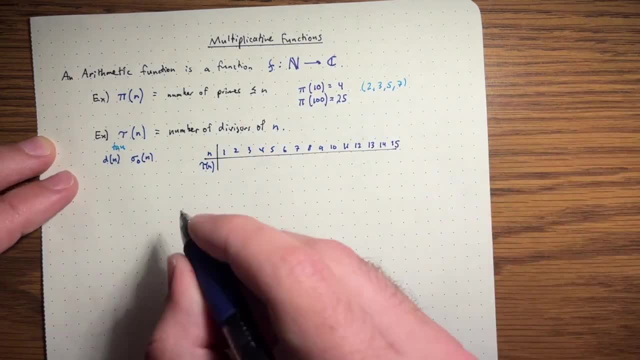 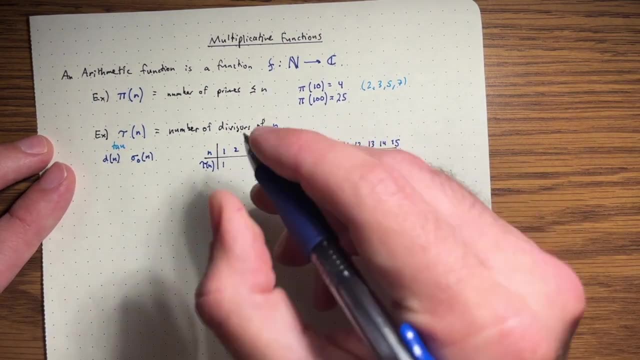 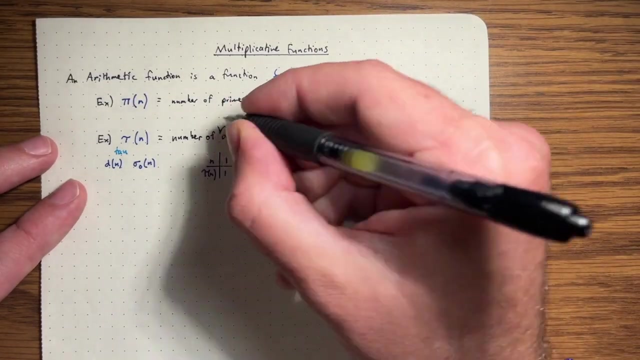 13,, 14,, 15.. Keep going. So 1 has one divisor, 2 has one divisor other than itself, But we're going to count all the divisors. So let me just emphasize that, Because I think we talked about divisors before. 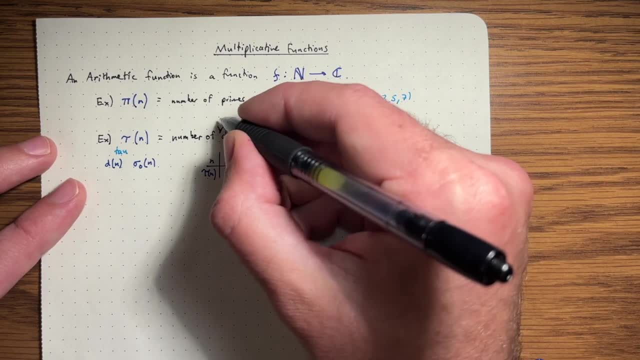 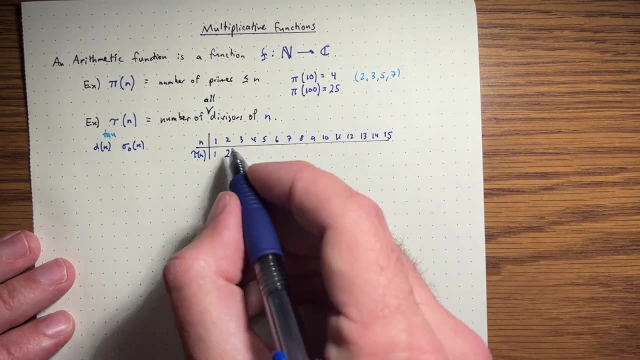 But we were talking about proper divisors, So we want all divisors of n, including the number itself. So 2 is a prime. So it has two divisors: 1 and itself. 3 also has two divisors: 5, 7.. 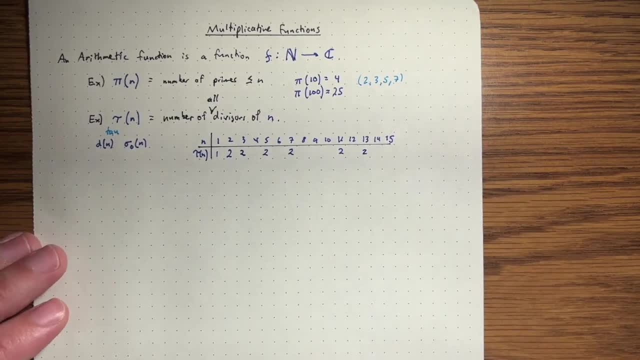 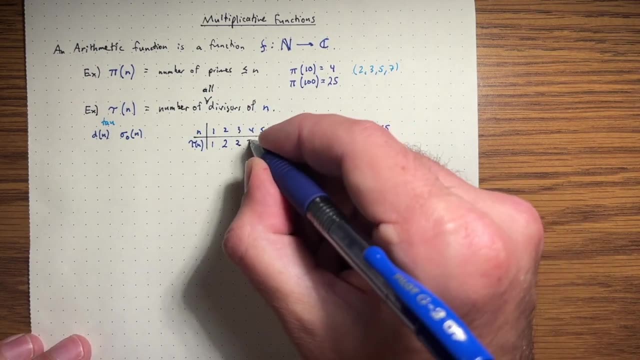 I'm going to just go to the primes and say those all have two divisors. How about 4?? 4 has 1,, 2, and 4.. So it's going to have three divisors. 6 has 1,, 2,, 3, and 6.. 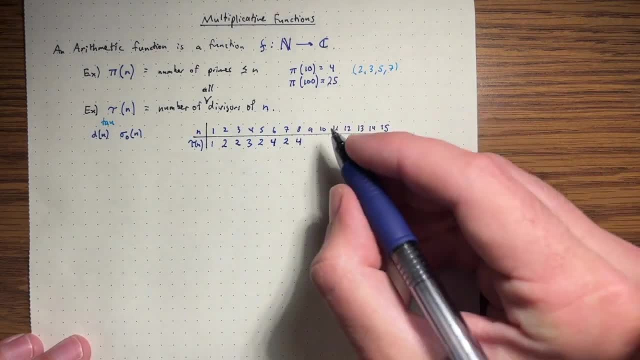 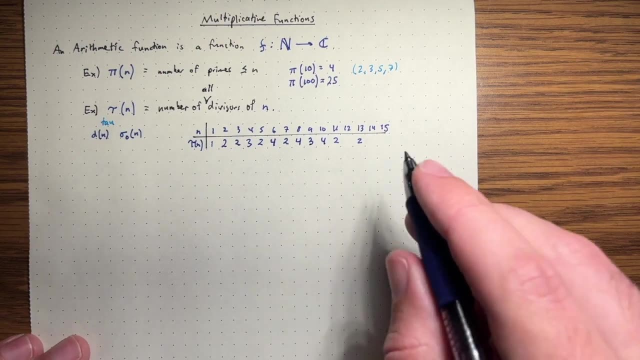 That's four divisors. 8 has four divisors. 9 has three divisors: 1,, 3, and 9.. 10 has four divisors. 12 has a lot of divisors: 1,, 2,, 3,, 4,, 6, and 12.. 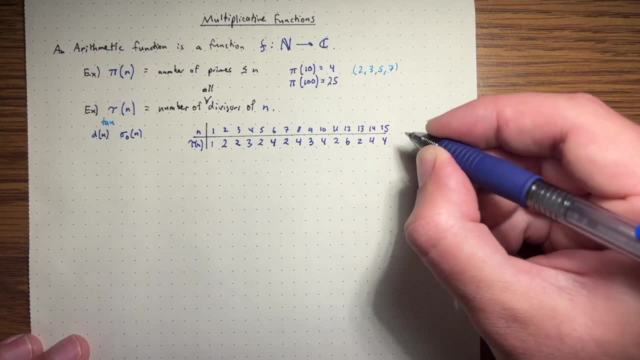 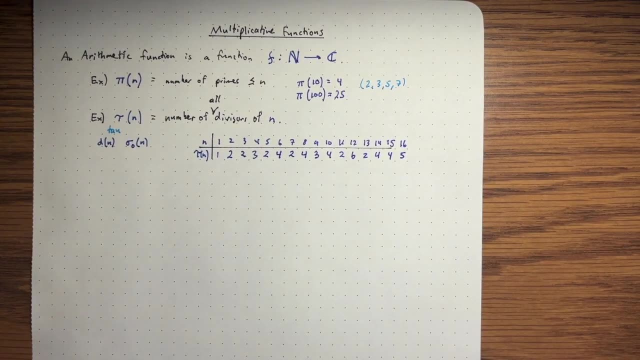 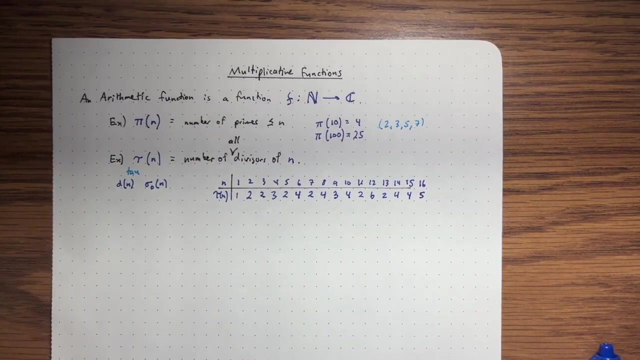 So it's going to be 6.. This one's going to be 4.. 4. Let's see if we go one more. 16 has five divisors, All right. So this is a function tau of n And, as you can see, it behaves a bit randomly. 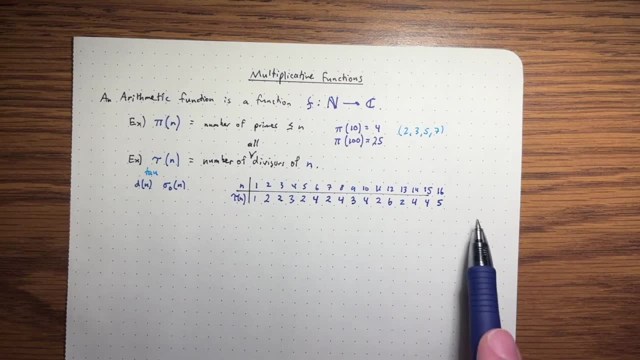 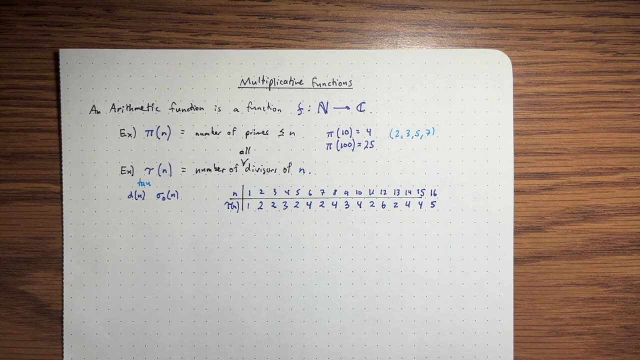 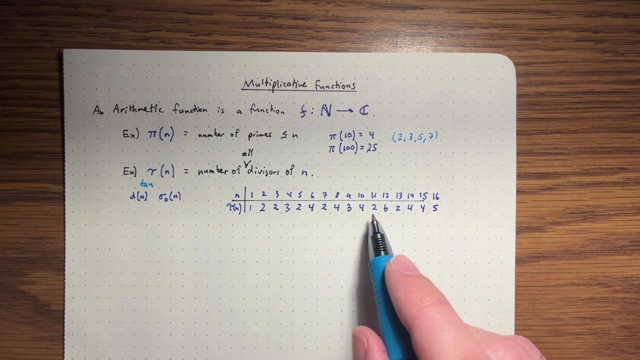 Got some big jumps. Can't often predict what's going to come next, But there is actually a fairly interesting pattern here. It's a bit tough to notice, But for example we could look at. let's look at the 12 here. 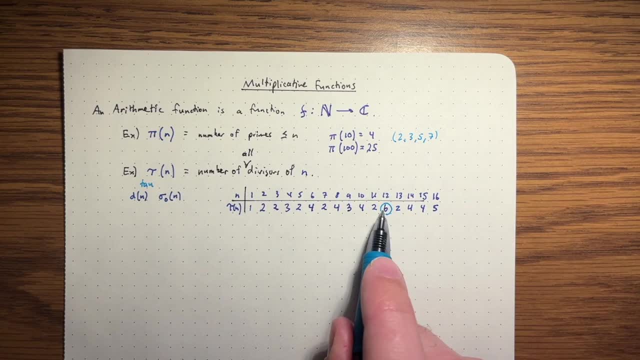 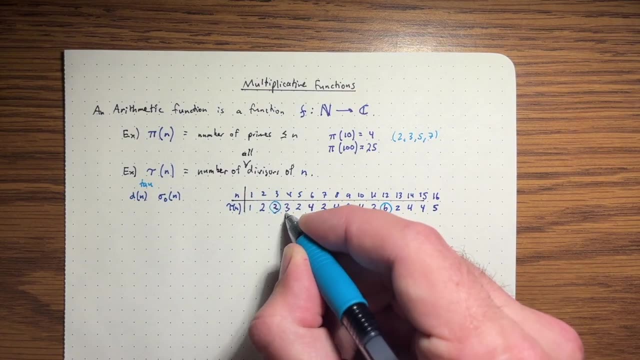 So 12 has six divisors. Well, 12 is 4 times 3.. And if you look at the number of divisors of 3 and the number of divisors of 4, it looks like the product, 2 times 3, is 6.. 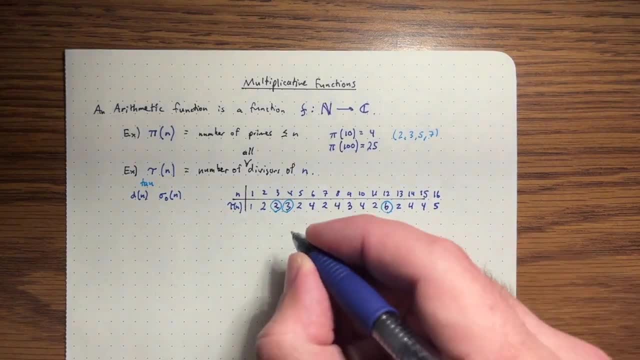 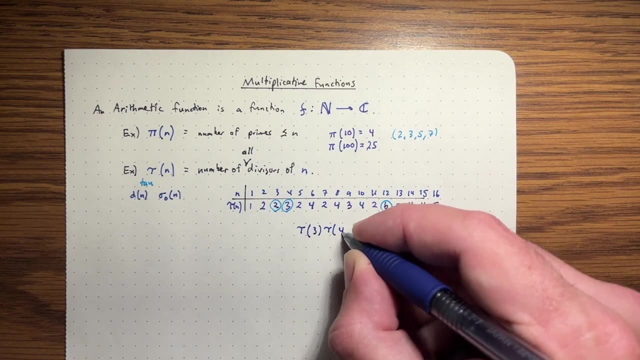 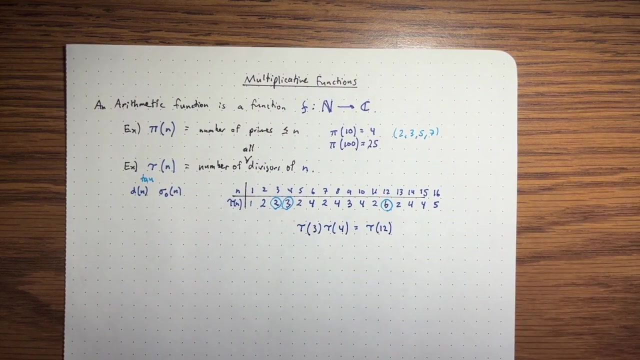 So, in other words, we have this relationship. So T of 3 times T of 4.. T of 4 is T of 12.. 12 is 3 times 4.. Well, you might say that this doesn't always seem to work. 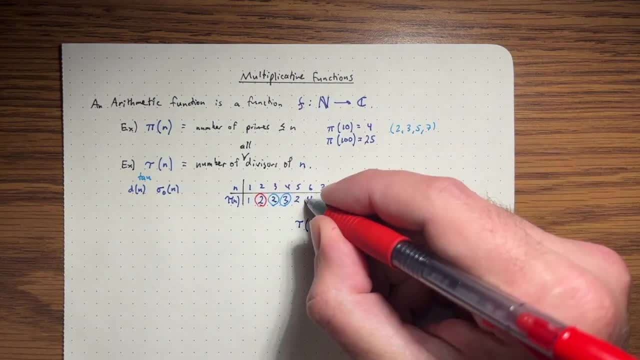 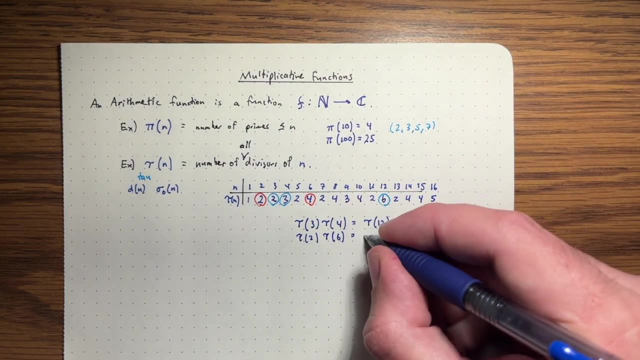 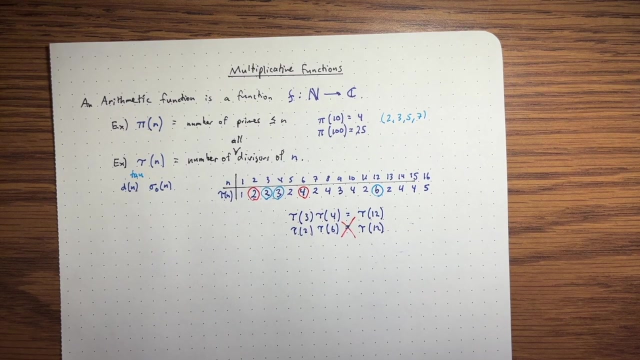 Because 12 is also 2 times 6. But tau of 2 times 2 is tau of 6.. Maybe we would expect that to be tau of 12.. But it's not. So this one does not work, But still, this is rather interesting. 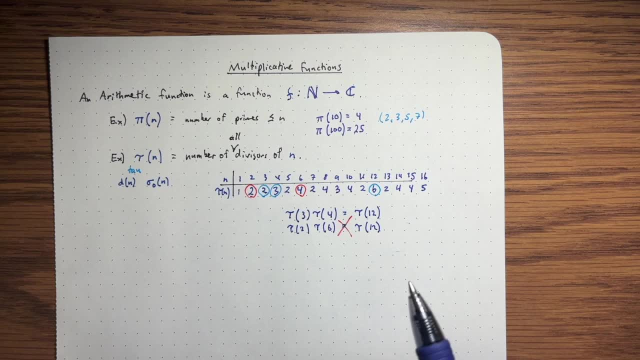 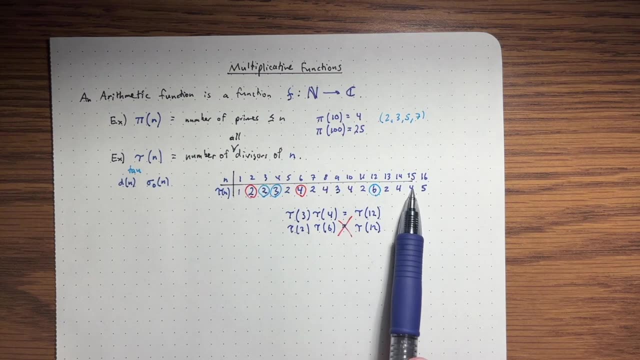 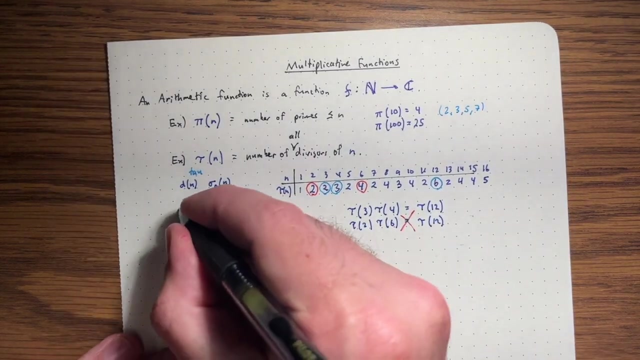 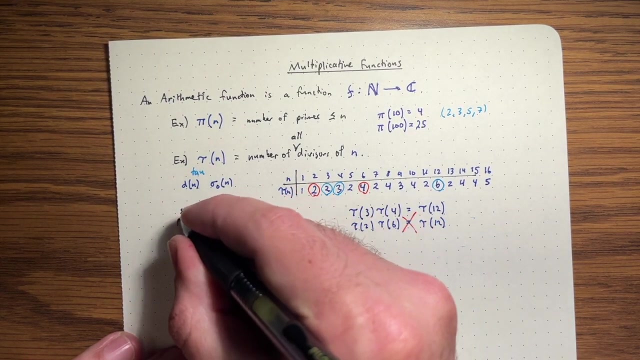 And you can actually see it happen a few more times here. So, for example, 15 has four divisors. 15 is 3 times 5.. 2 times 2 is 4.. And so the observation is that sometimes, so sometimes, it seems that 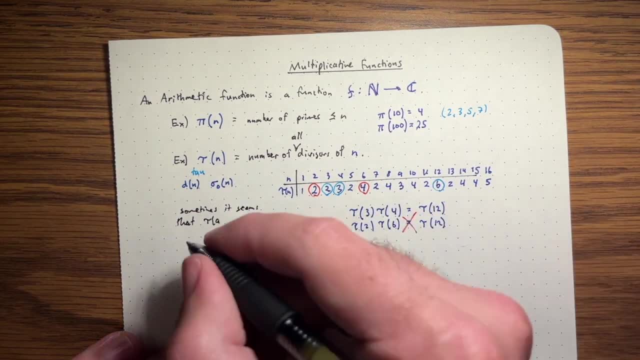 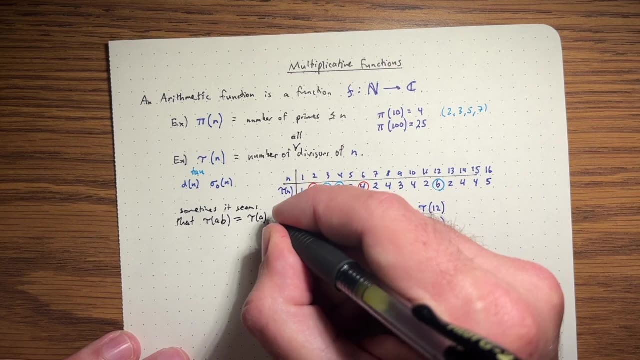 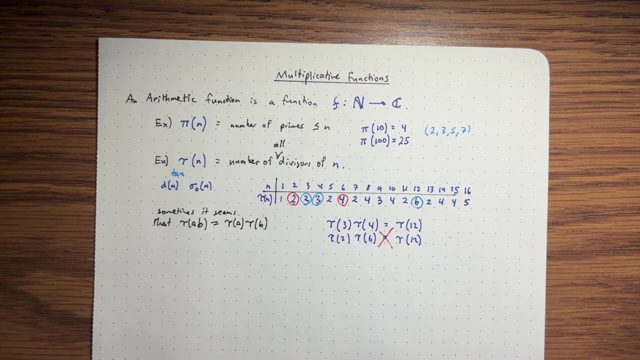 you can find many more examples if you write out this table further. It seems that tau of a product of two numbers is equal to tau of A times tau of B. So you can multiply the numbers of divisors together to get the number of divisors here. 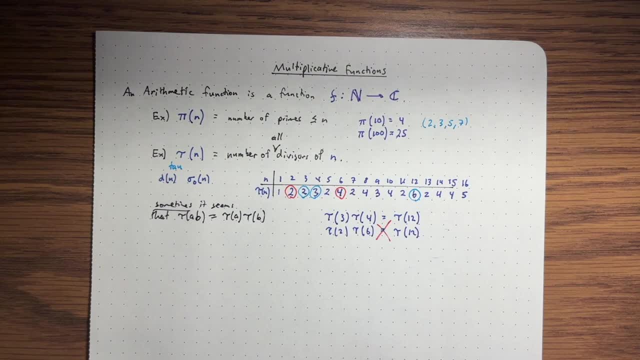 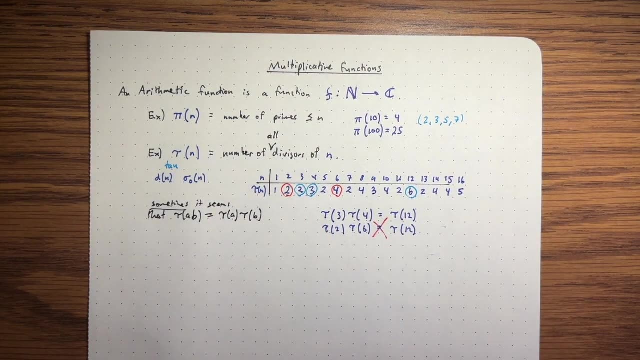 But it's only sometimes. This doesn't always work. Let's try to figure out exactly when this works. So we already know something about this function. We have a formula for it. We have a formula for tau of n based on the prime factorization of n. 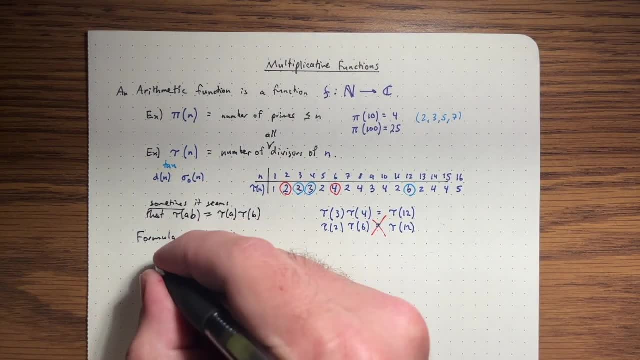 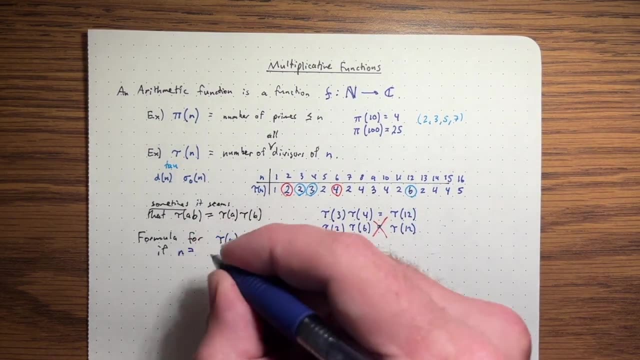 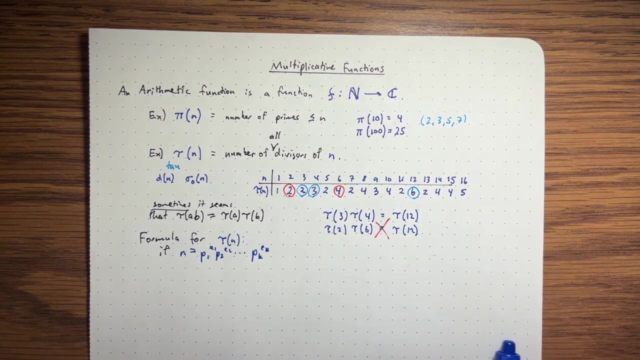 And here's that formula. So if n is this product of prime, so p1 to the e1,, p2 to the e2, etc. pk to the ek, Then tau of n is. So how do we find a number of divisors? 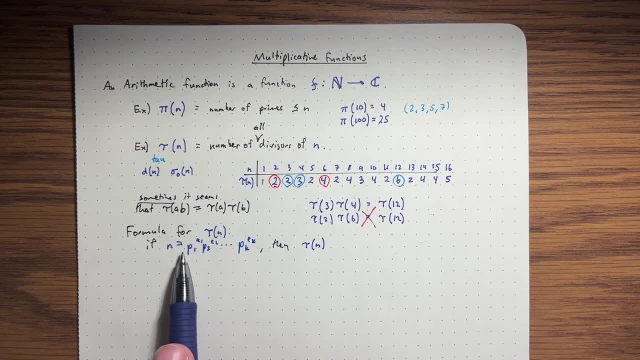 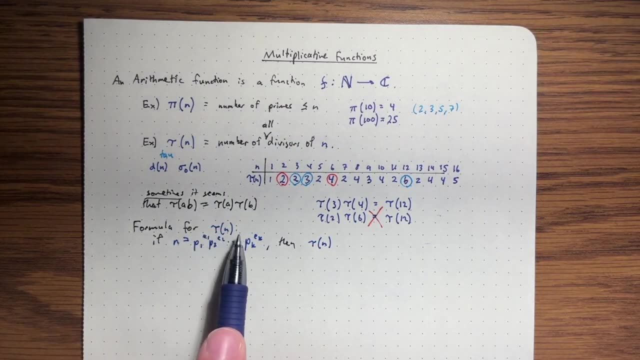 Let's just review this really quick. So essentially you can see all the divisors sitting here. You can just take any powers you want and you get a divisor of n. If you take 0 powers for all of them, you get a divisor of 1.. 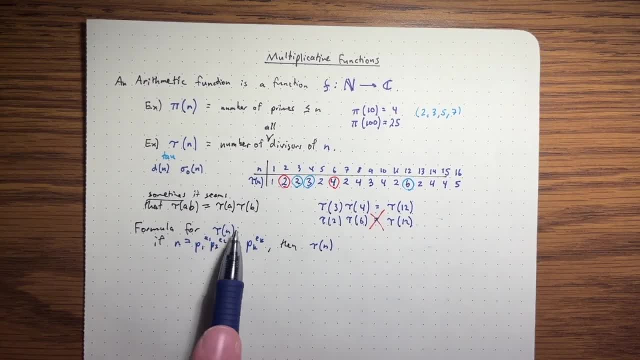 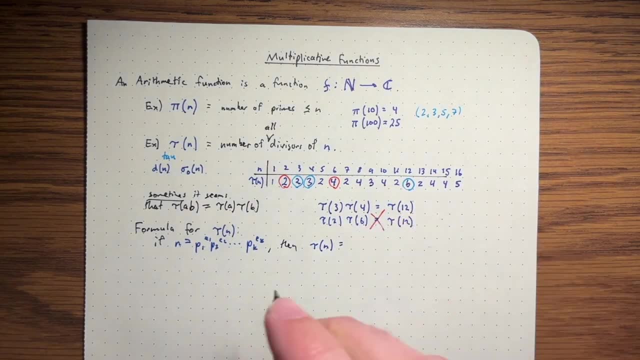 You can take any prime you want in the factorization of n to any power you want up to its exponent. You can't go over its exponent. So essentially, if I want to factor p1, I have e1 plus 1 choices for that. 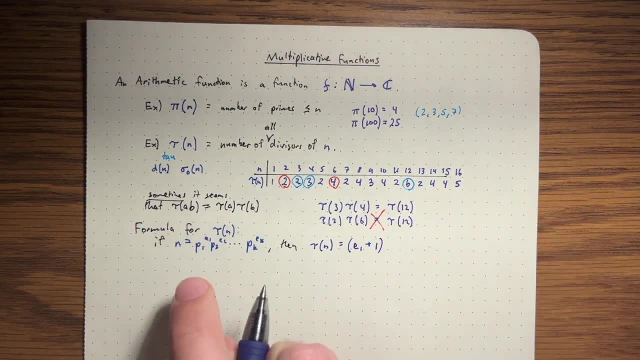 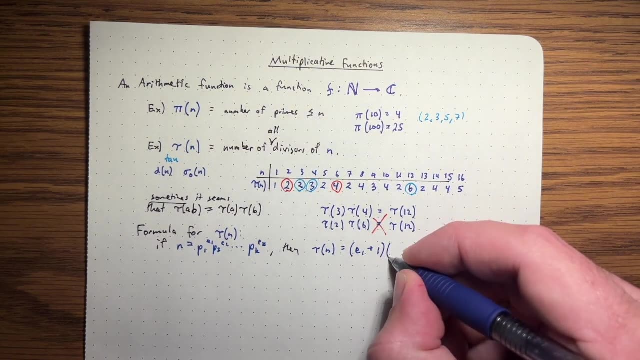 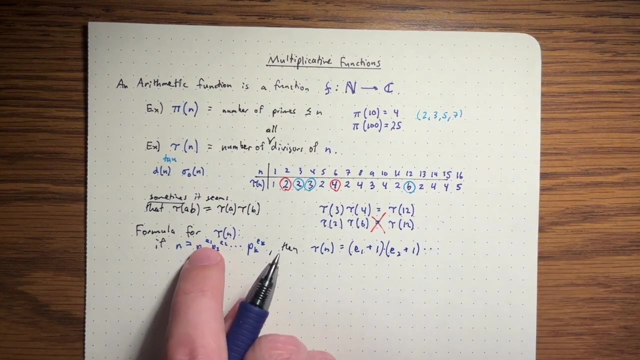 Plus 1, because I can choose to take 0 of this prime And then I can do the same for this prime, e2 plus 1 times. I'm multiplying right, Because for each choice of the exponent here I can take e2 plus 1 choices of the next one, etc. 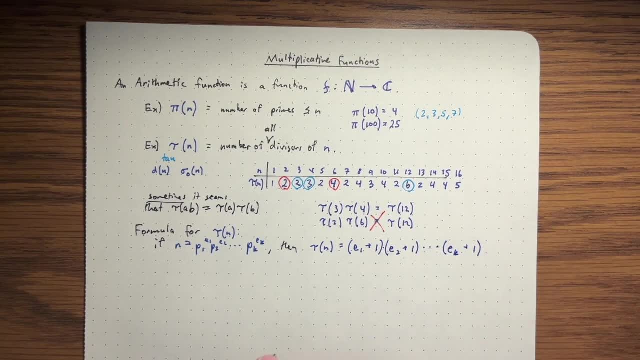 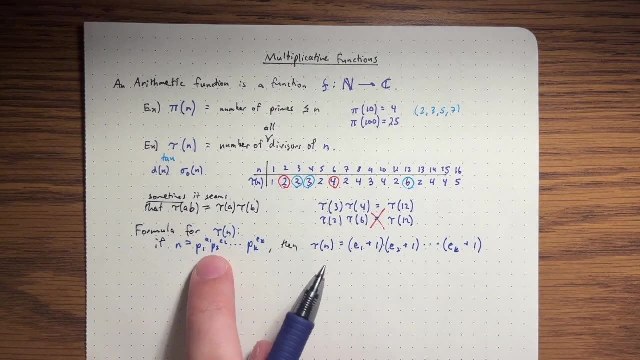 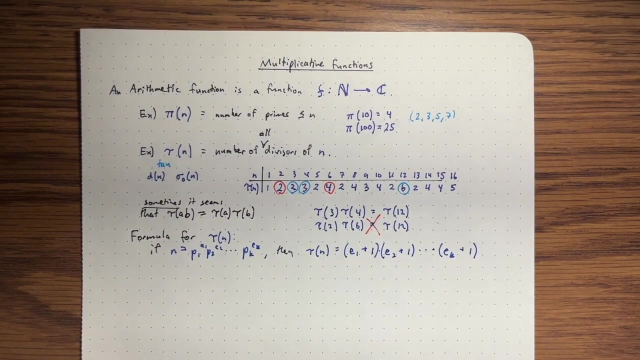 Until we get to this last term here. The nice thing about this formula is it doesn't actually care about what our primes are, So it just sort of cares about the exponents in the prime factorization. So that's rather interesting, And so let's try to figure out what's going on here. 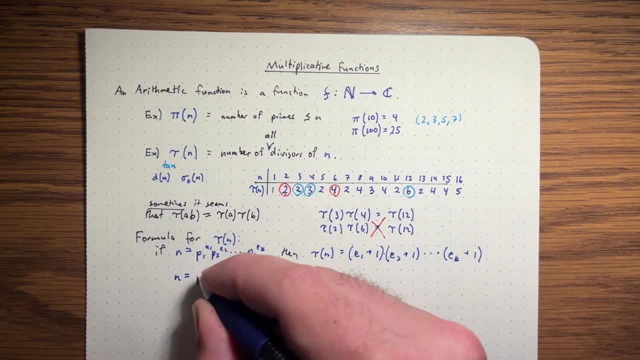 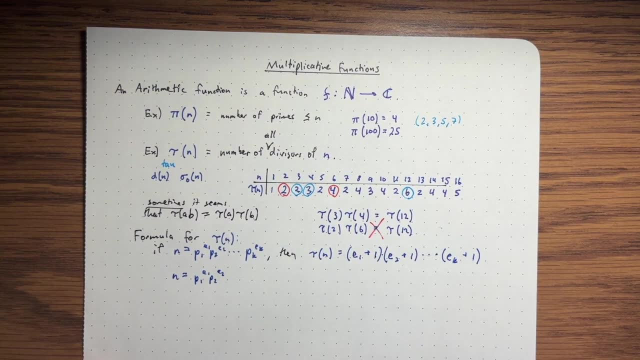 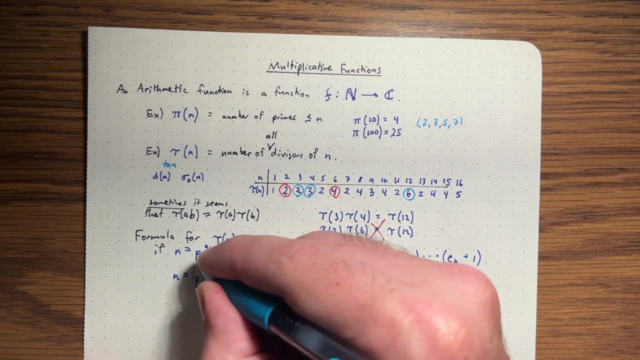 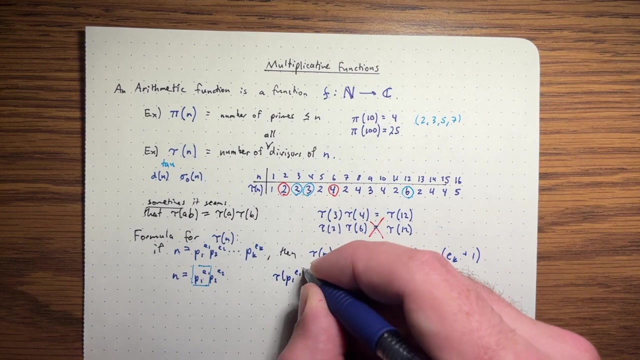 So, let's say, our number just had two prime factors Like this. Well, let's say we said, let's say we split it up like this: So we'll take this prime and tau of p1 to the e1. Well, what's that going to be? 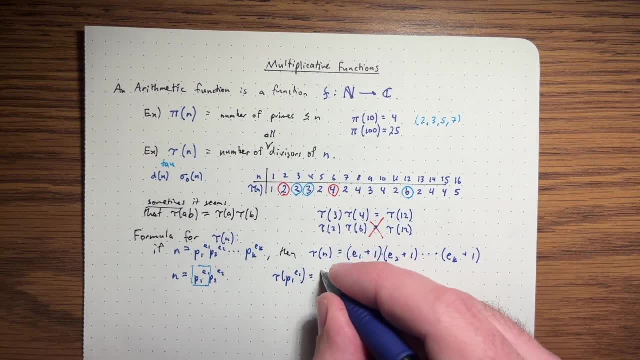 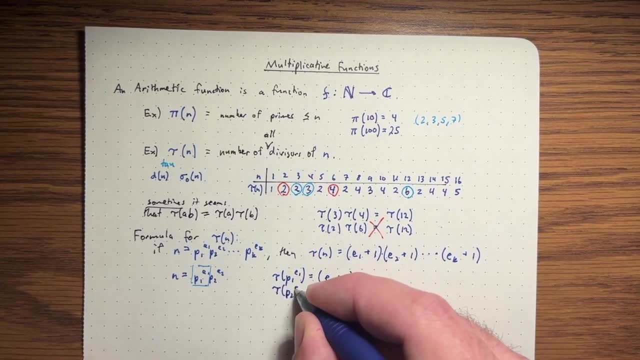 I mean this is just going to have e1 plus 1 divisors. We can take any power of this prime we want And then if we do the same with the second prime power, we get that that's going to have e2 plus 1 divisors. 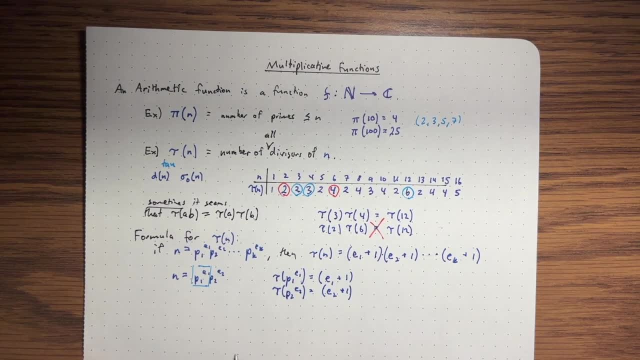 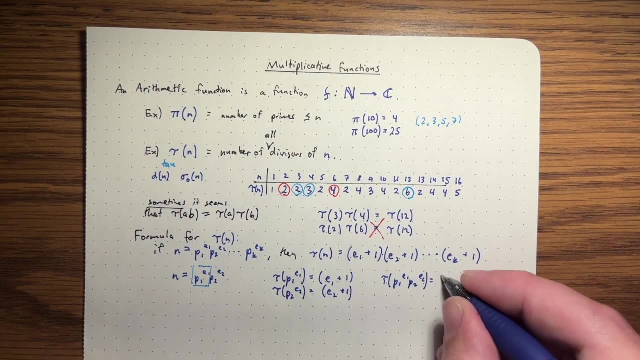 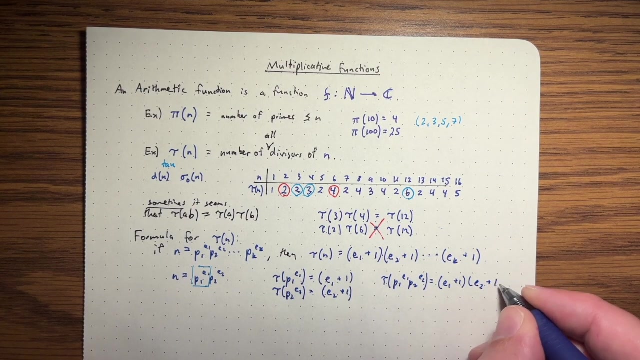 But now tau of this entire number. that's going to be sort of independent choices here because they're different primes. So it's going to be e1 plus 1 times e2 plus 1 by our formula. But you'll notice this is just the same as 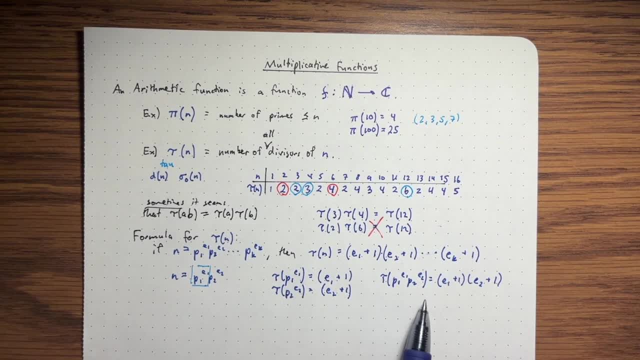 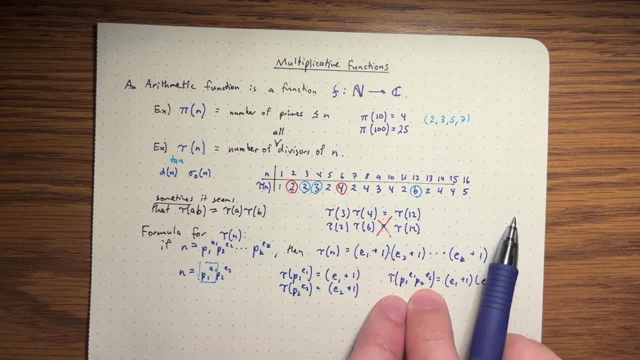 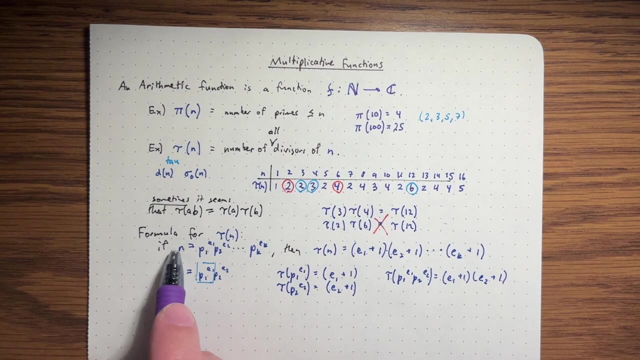 tau of p1 to e1 times tau of p2 to the e2.. So essentially when you have different primes you can split apart the product into two parts and then do it separately. So in general what you can do is if you write n as a product of relatively prime numbers. 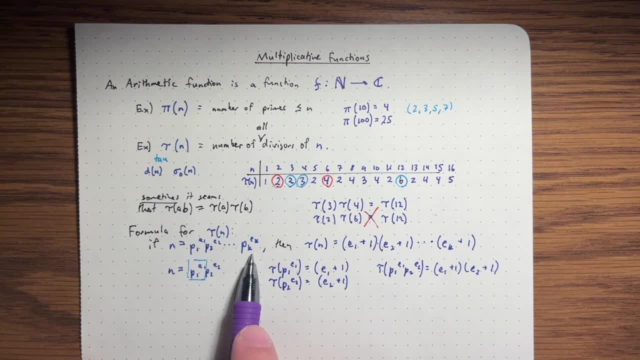 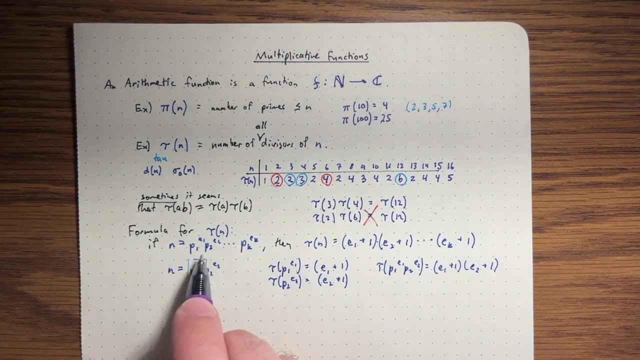 so what would that mean in terms of the factorization, Two numbers will be relatively prime if they don't share any prime factors in common. So, for example, if I split these p1 and p2 off and write n as this product times the rest of it. 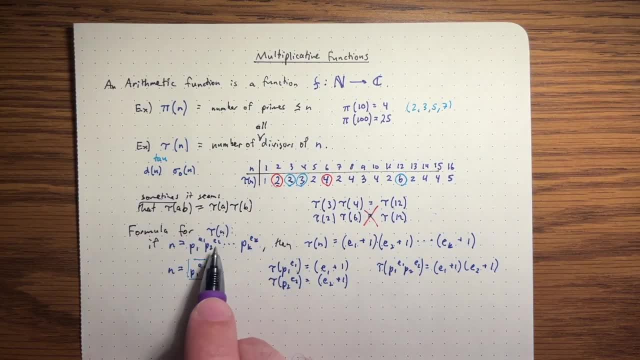 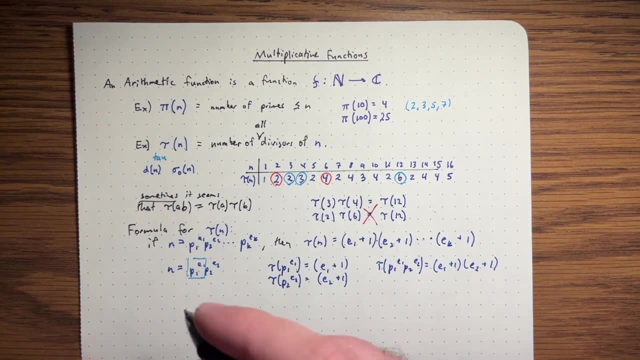 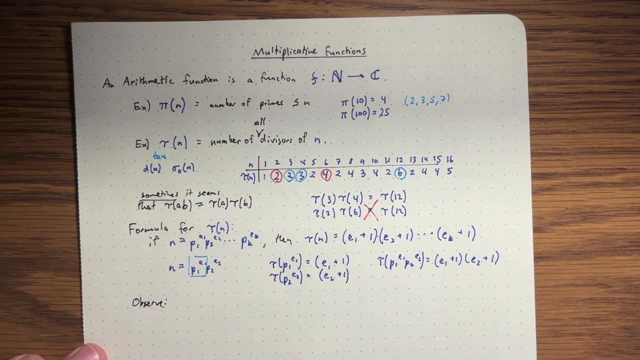 I can sort of do this part separately, multiply it together, find the number of divisors and then multiply them both together. So sorry, I said a lot of words there, but let's record what we just observed. So observe in general. 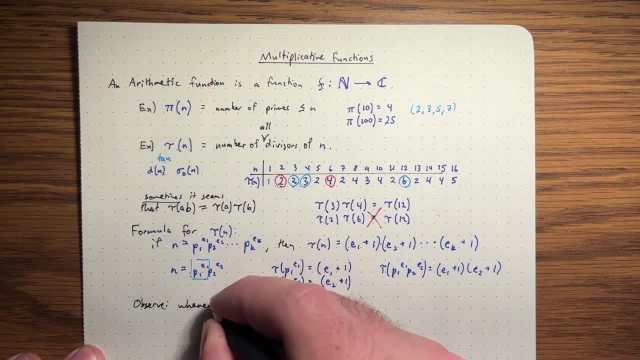 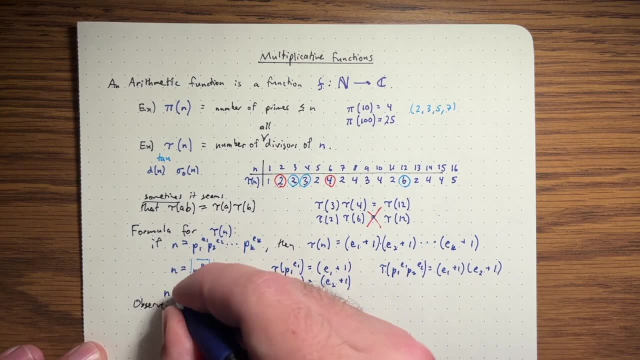 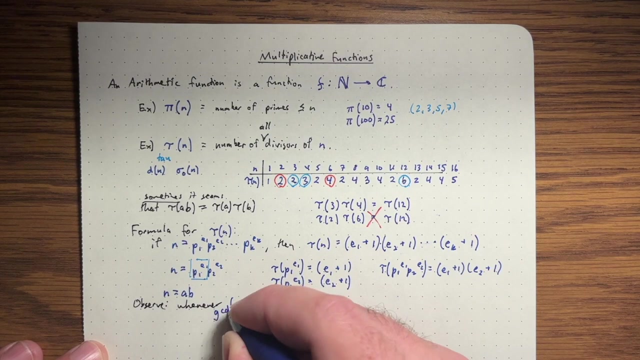 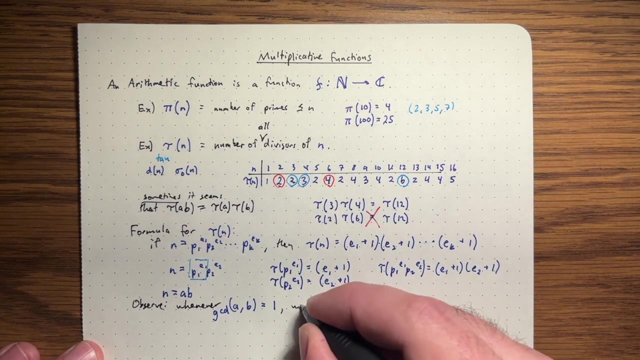 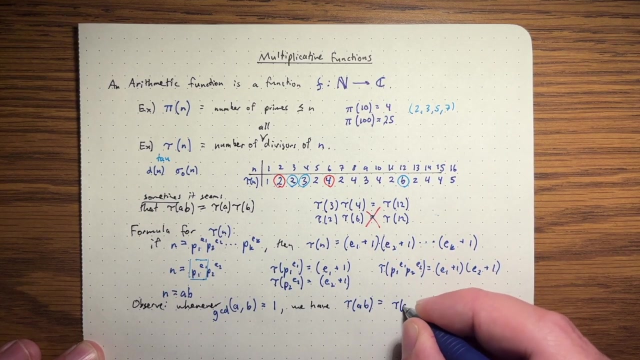 So whenever let's write n as a product of, let's write n as a product. So whenever a and b are relatively prime, so whenever the GCD is 1, we have, tau of ab is equal to tau of a times tau of b. 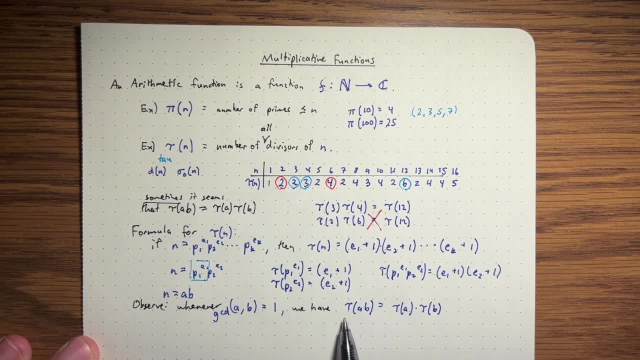 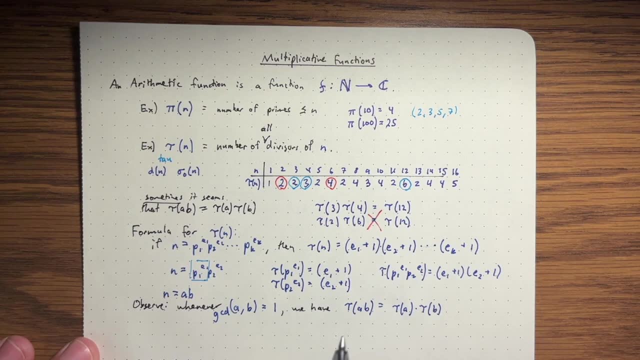 Essentially that's just from our observation here, because a and b are relatively prime, so they'll involve different primes in the prime factorization. but our formula just involves multiplying all these factors together in the end anyway. So this is a really interesting property here. 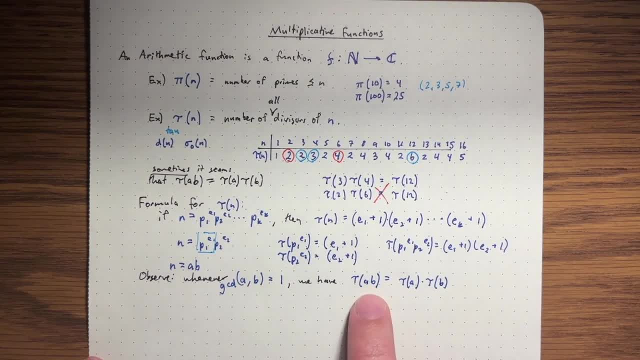 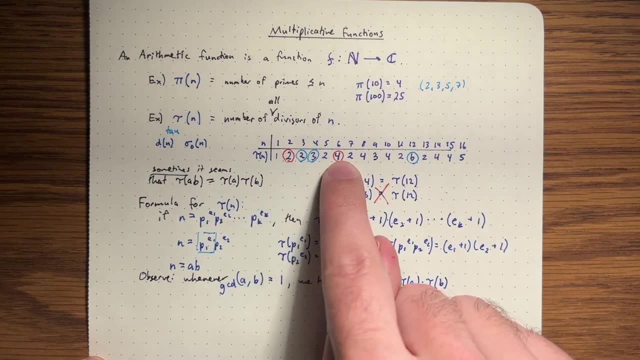 It only works if a and b are relatively prime. So if you pick a and b to be not relatively prime, this can easily fail, as we've seen here with tau of 2 times tau of 6. That's not equal to tau of 12.. 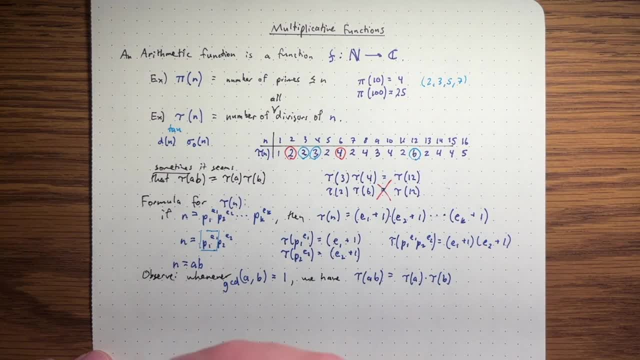 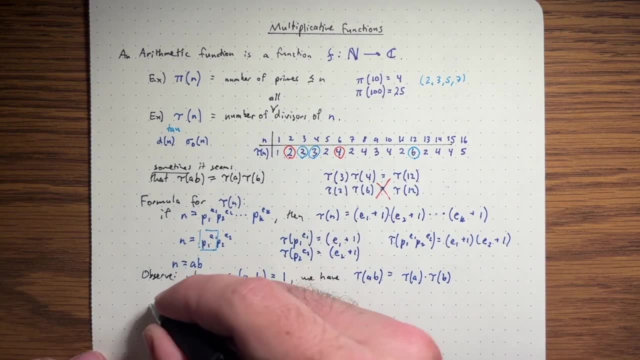 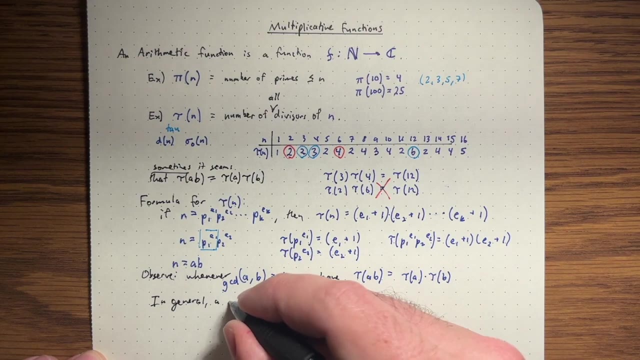 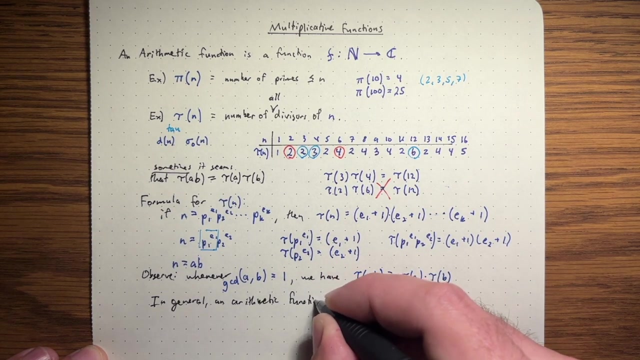 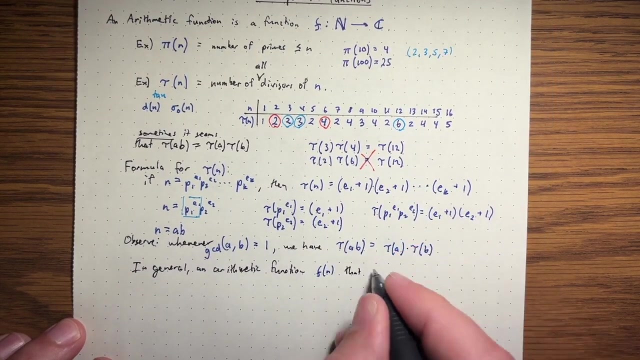 But let's subtract this definition. as a definition, This turns out to be a really useful observation. So in general, an arithmetic function, let's call it f of n- that satisfies essentially this same property that tau does. that satisfies essentially this same property that tau does. 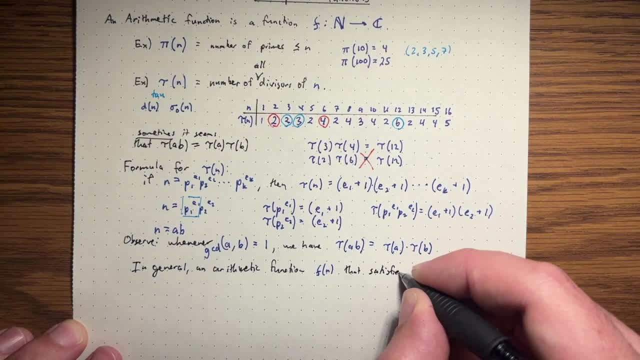 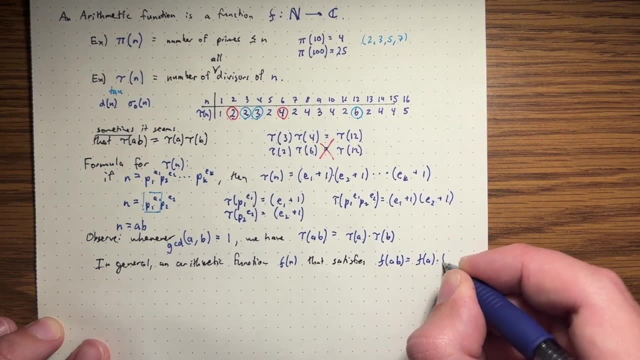 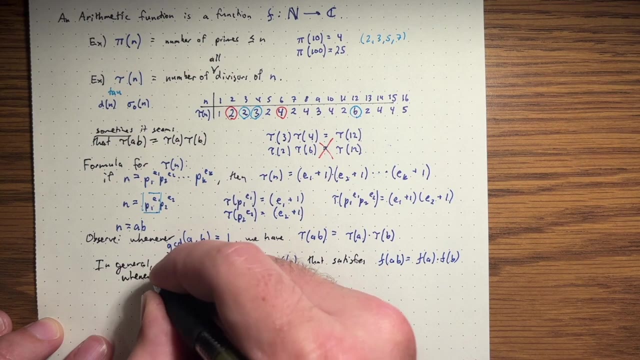 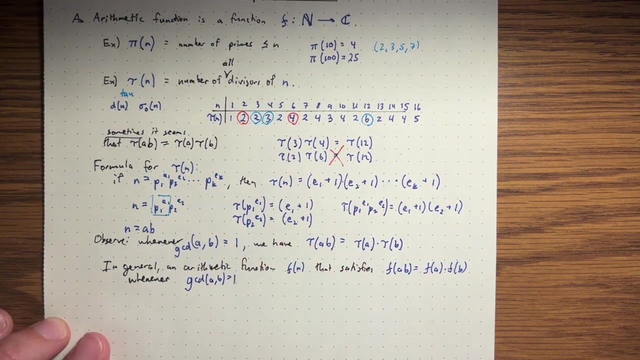 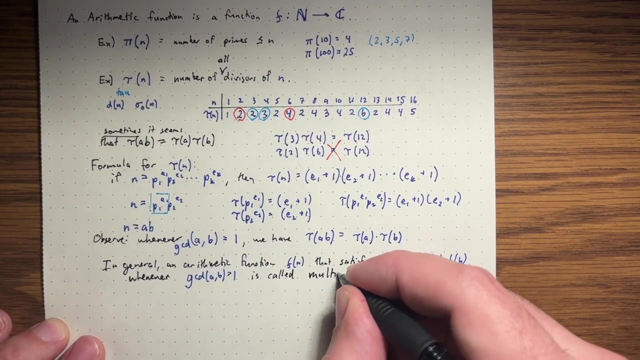 So that satisfies f of a product equals f of a times f of b. whenever a and b are relatively prime is called multiplicative. So multiplicative means this very precise property. It doesn't mean you can always do this, It just means that when you have two relatively prime numbers 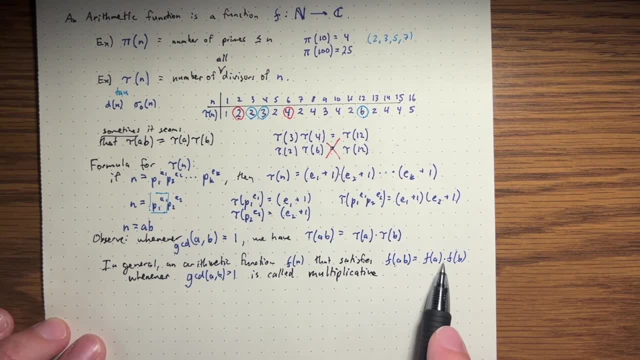 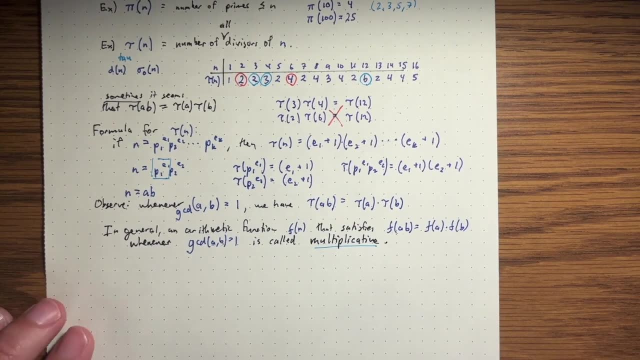 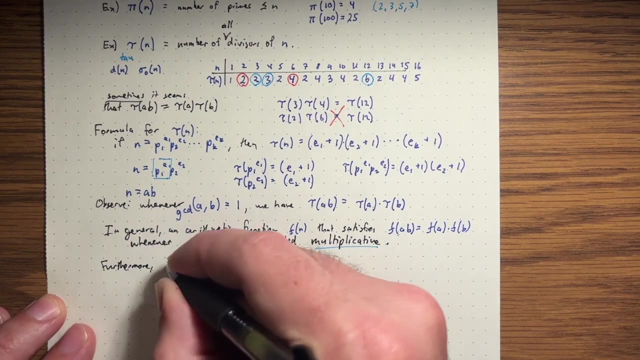 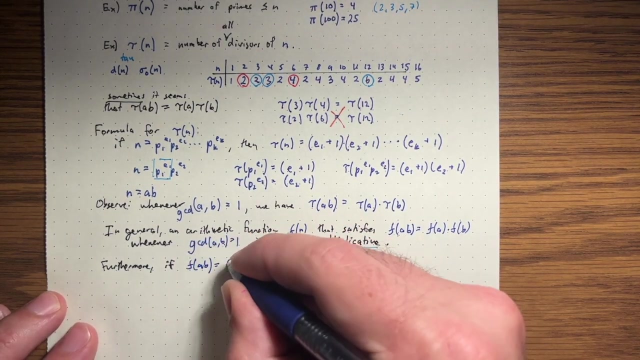 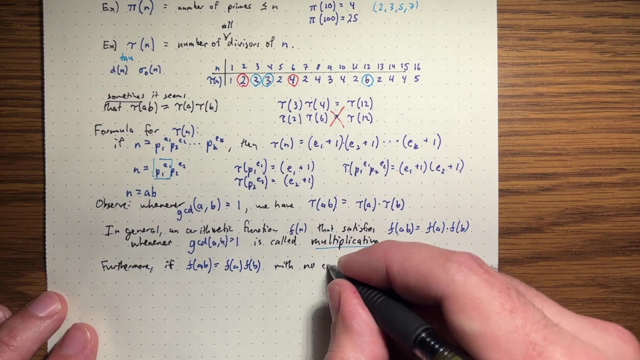 two numbers with no factors in common, then f of a- b equals f of a times f of b. So this is multiplicative, Okay, furthermore. so, furthermore, if f of a- b equals f, f of a times f of b, with no conditions on a and b, 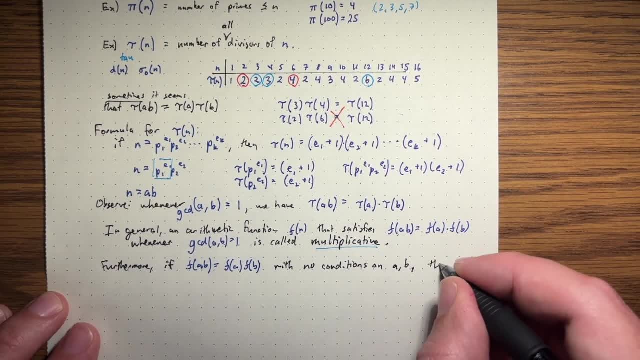 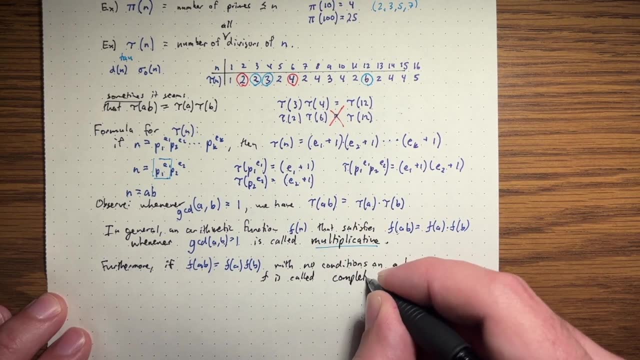 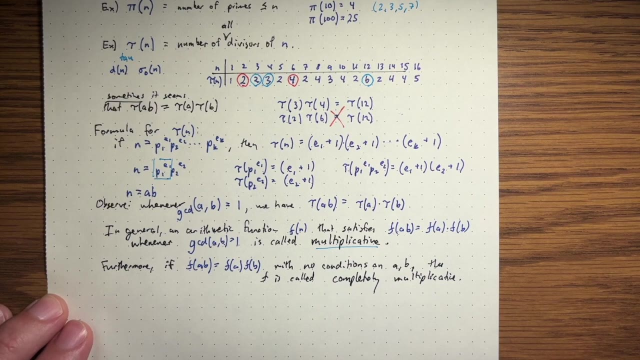 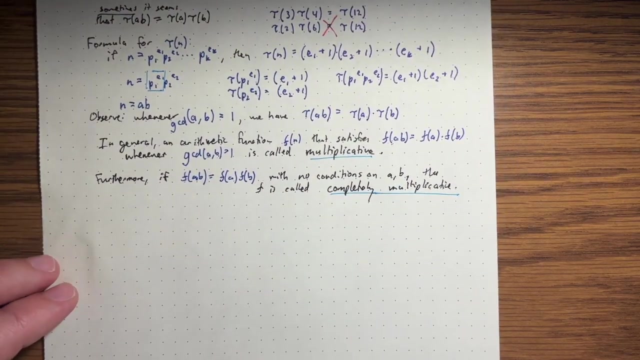 with no conditions on a and b. then f is called completely multiplicative. Okay, so even when two numbers are not relatively prime, you still have this property. That's actually rather hard to do, But here's an example. So just this function. 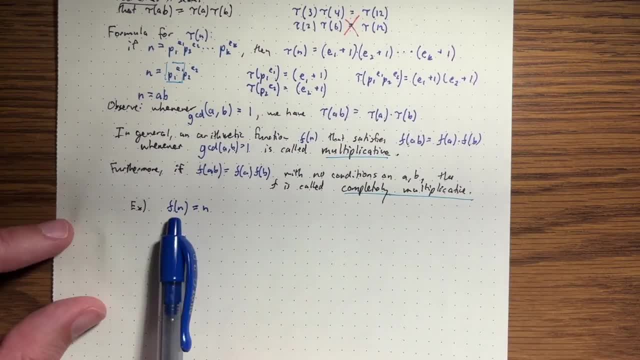 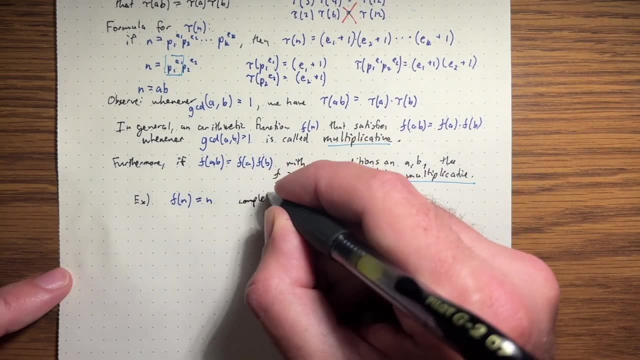 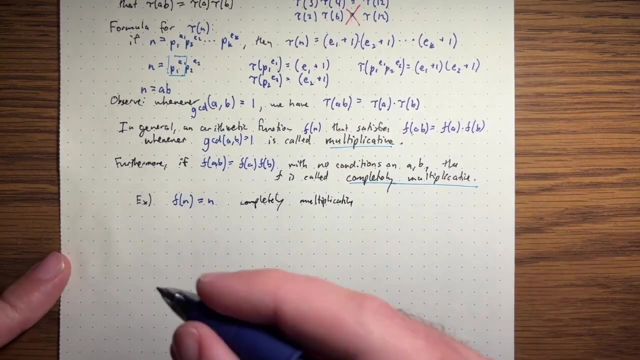 So f of n equals n, the identity function. So f of 6 would just be 6 itself. This function is completely multiplicative. You can also, you can even raise n to any fixed power you want. So f of n equals n to some fixed power. 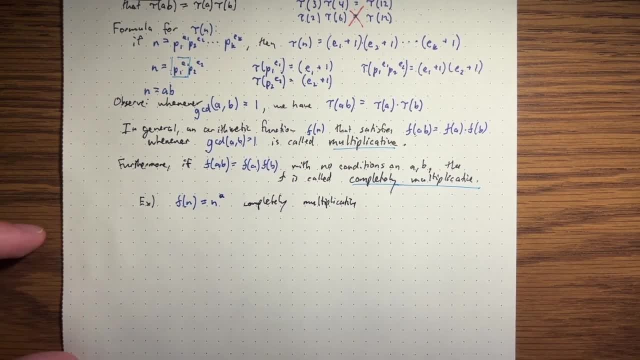 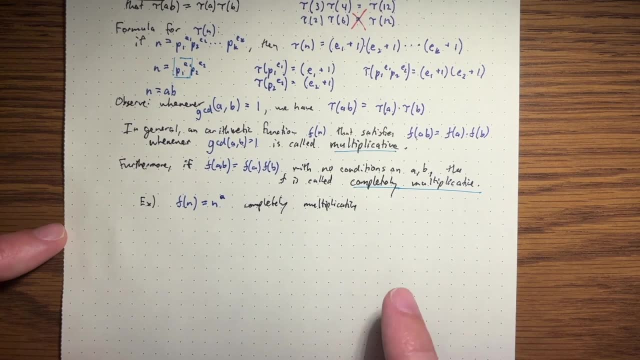 That's also going to be completely multiplicative. And, by the way, that even includes a 0 power. So f of n equals 1.. The function just always gives you 1.. I mean, that's definitely going to be completely multiplicative. 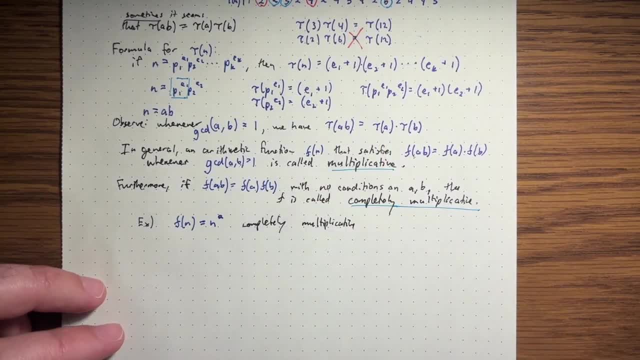 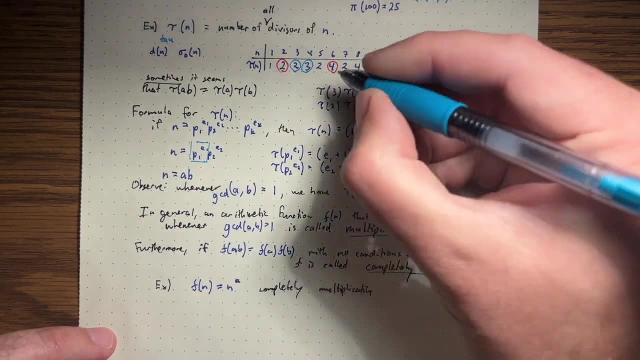 Okay, we saw today, okay, we saw tau is multiplicative, but not completely multiplicative. It's not completely multiplicative because this property doesn't always work. So it only worked with the 3 and the 4, because 3 and 4 are relatively prime. 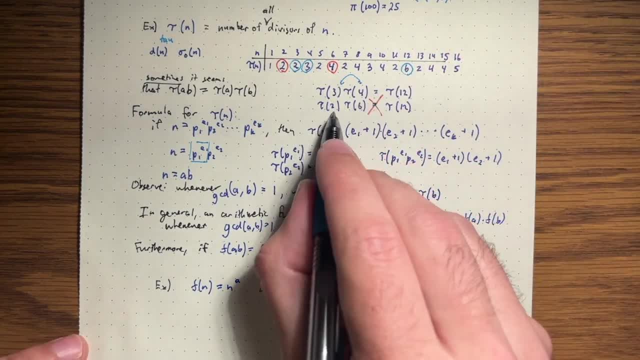 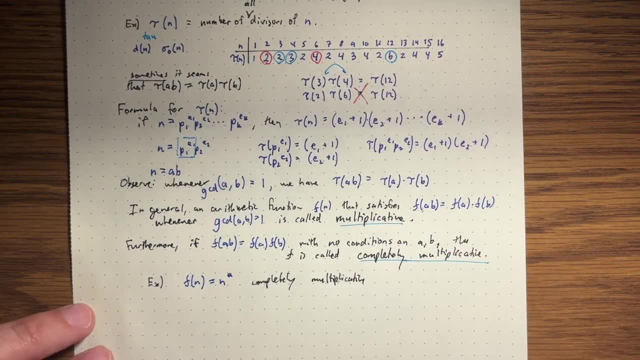 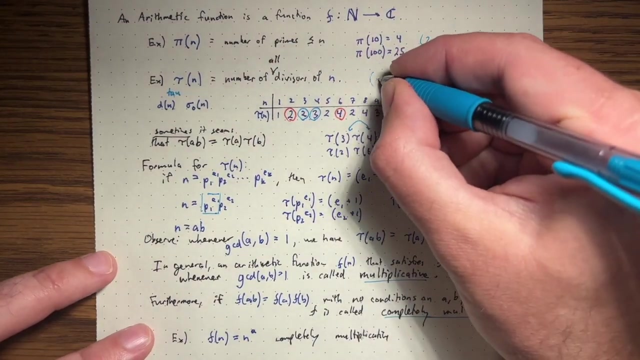 2 and 6 are not relatively prime. They share a factor of 2. So this doesn't apply. But tau is multiplicative. What's the example that's not multiplicative, So let's just try this. So this is a multiplicative function. 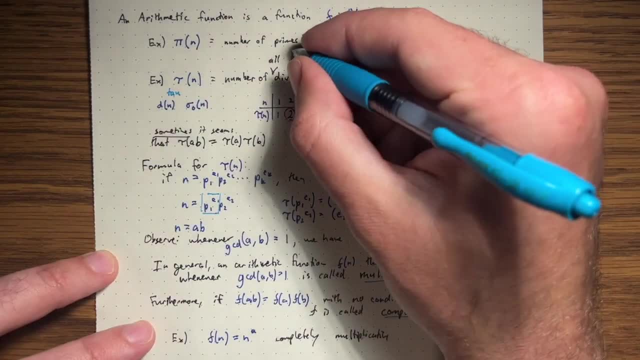 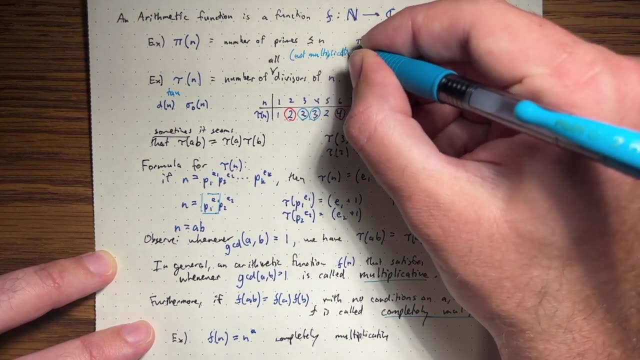 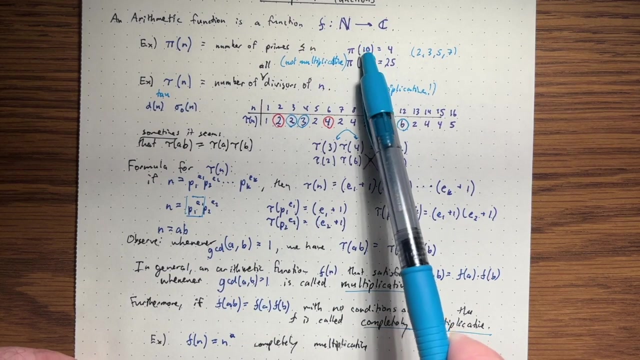 An example above is not multiplicative. It's an arithmetic function but it's not multiplicative And you can check that probably just by trying any two numbers. For example, pi of 100 is not pi of 10 times pi of 10.. 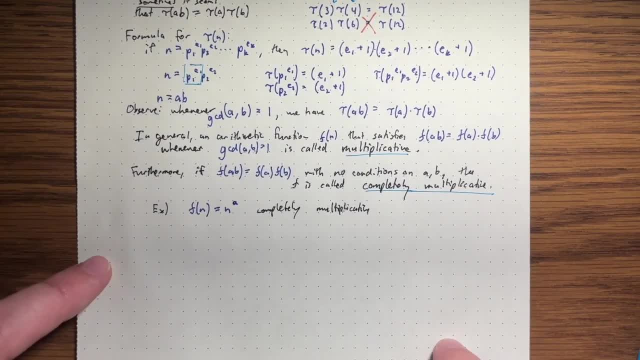 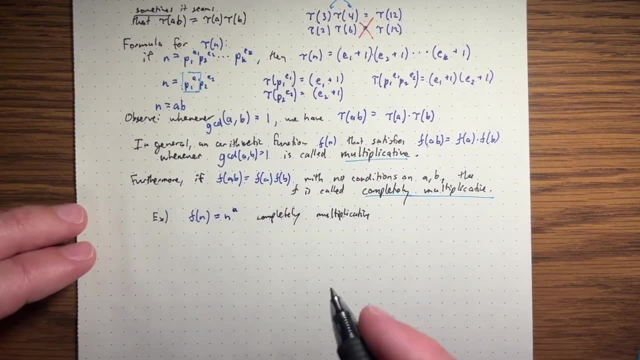 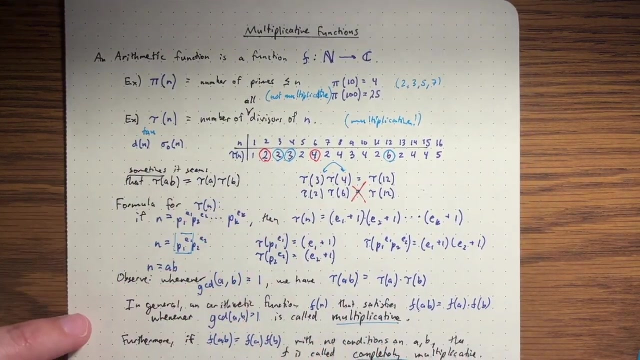 Okay, let's investigate this function, tau, a little bit closer. It's a really important function in number theory. Some people even say number theory is really the study of these arithmetic functions, because they just encapsulate so much of what we want to study in number theory. 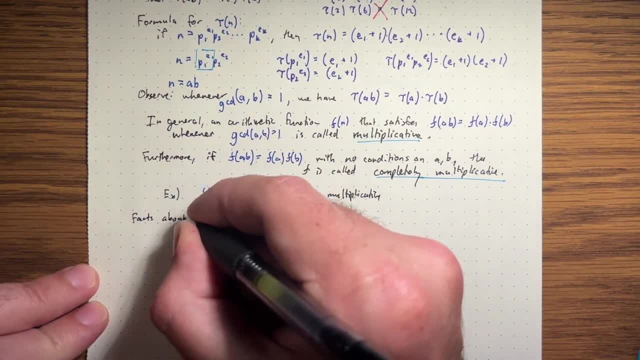 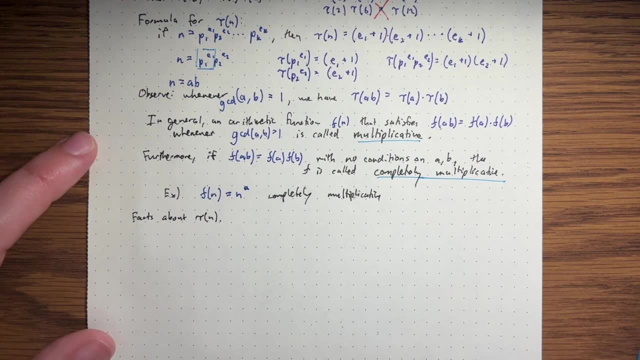 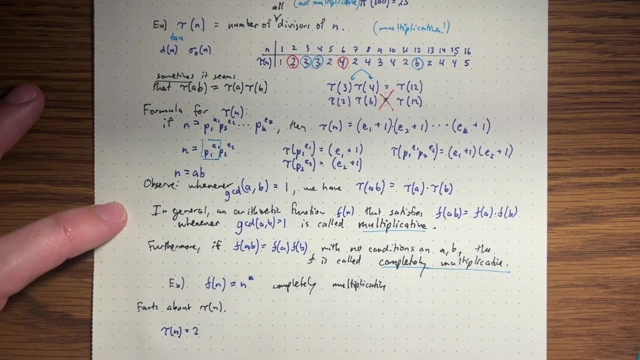 Let's look at some facts about this function: tau. Facts about tau. Let's start with maybe some more obvious ones. So tau- sometimes tau is 2.. That happens exactly when So tau is 2 if, and only if, n is prime. 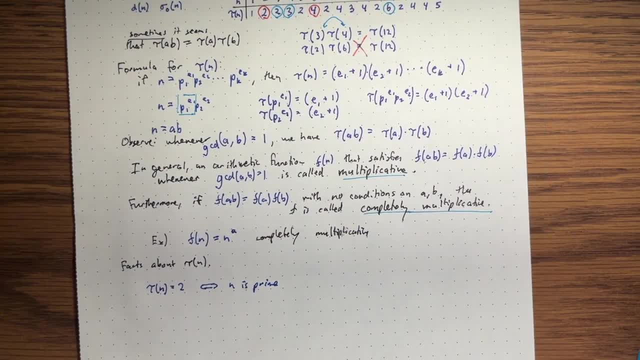 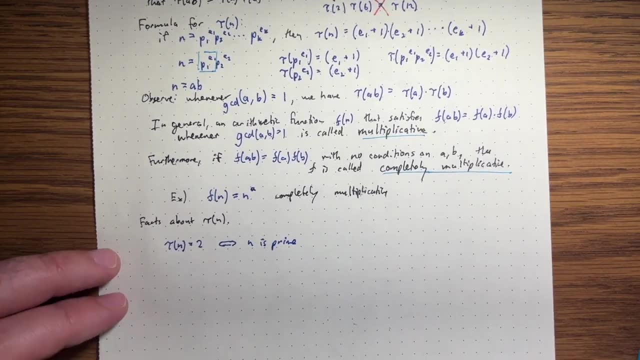 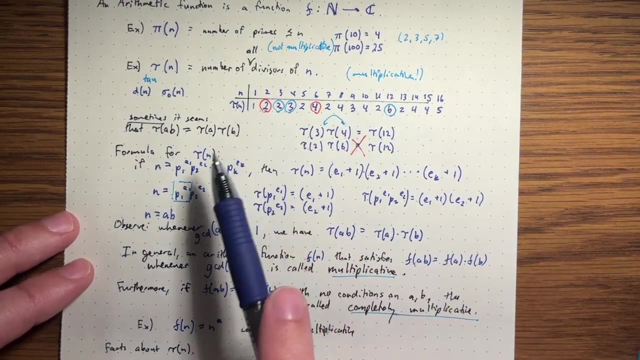 just essentially by definition of prime Prime numbers are ones with exactly two positive divisors. I'm always talking about positive divisors here, by the way. Here's a more interesting one. Can you spot the pattern? So sometimes n is odd. 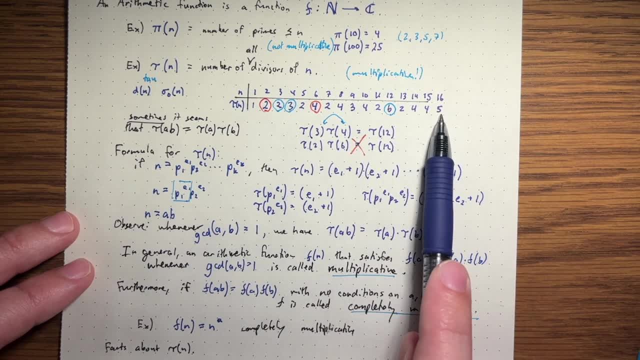 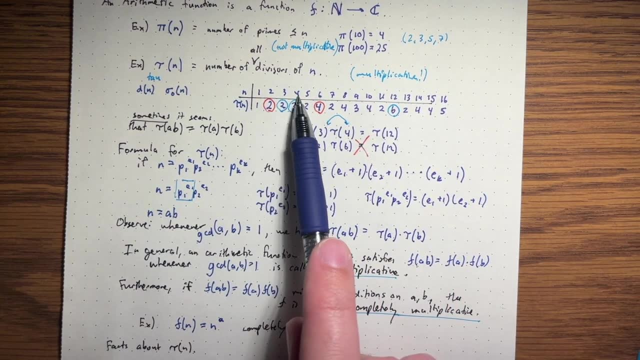 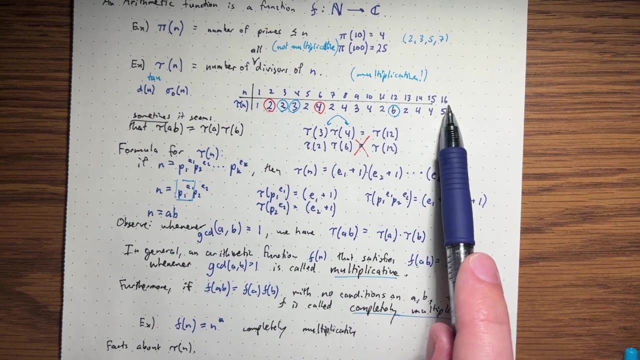 For example here And here. So can you spot the pattern there, When n is 4 and 9.. Yeah, sometimes tau of n is odd. So when n equals 4,, 9, or 16,, also 1 itself. 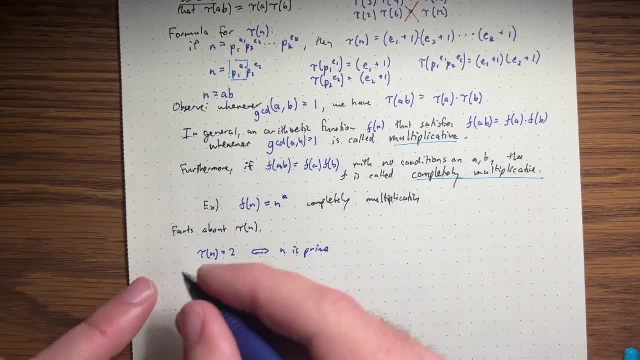 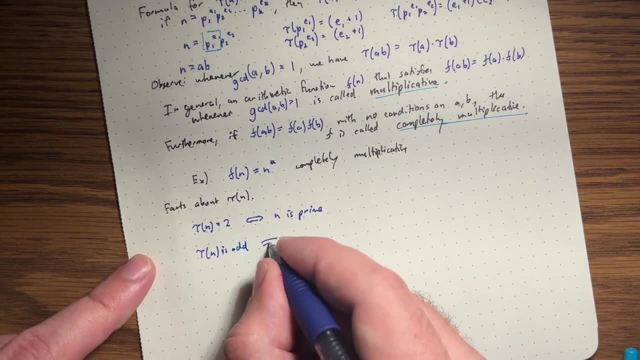 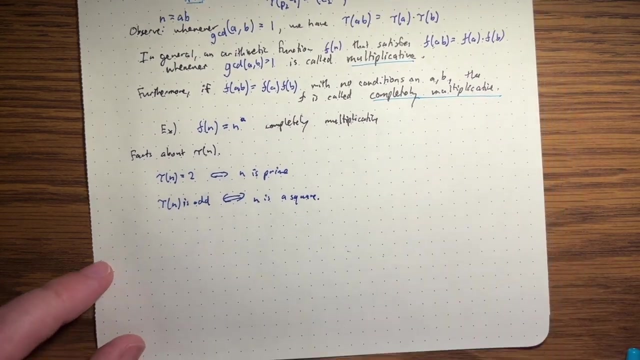 So it appears that when n is a square number, So let's record that. So tau of n is odd. This is what we want to prove, maybe. So if, and only if, n is a square, Let's see if we can understand why that's true. 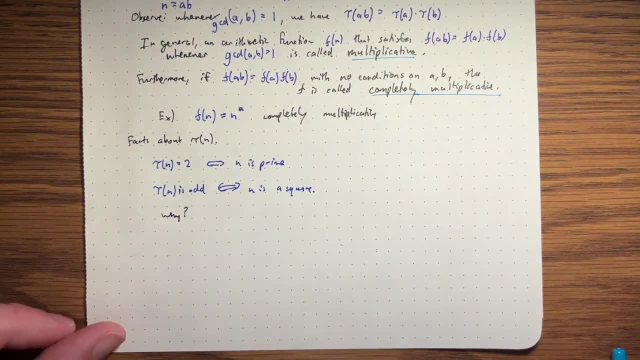 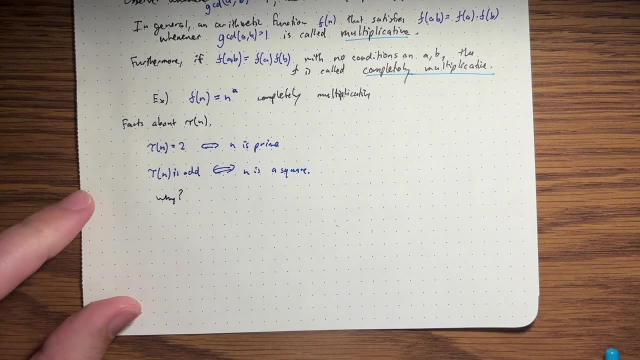 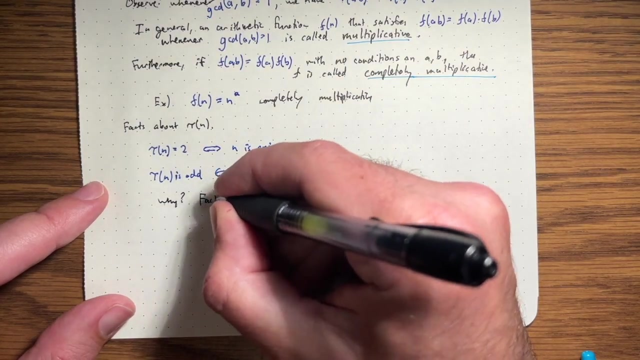 So why is this true? Well, there are a couple reasons for it, But let's try to prove it from the prime factorization. So, first of all, how do you identify something as a square from the prime factorization? It's actually fairly easy to do. 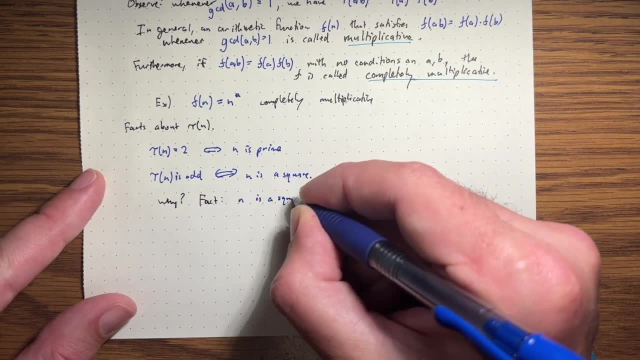 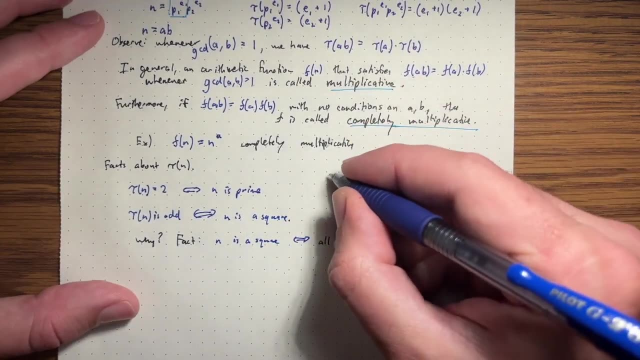 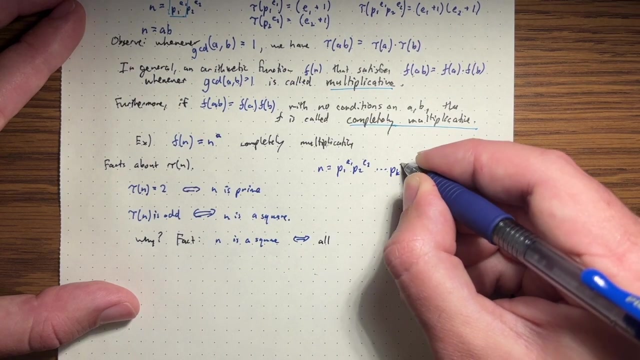 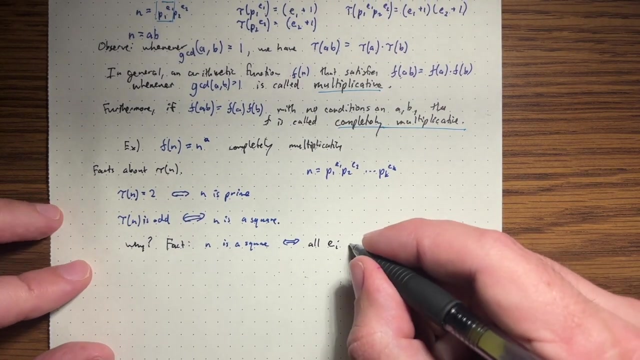 So n is a square If, and only if. So I'm just always going to assume that n is going to have some prime factorization. So n is a square if, and only if, all of the exponents in the prime factorization are even. 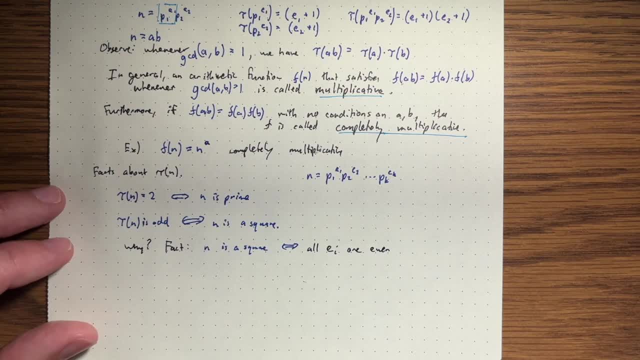 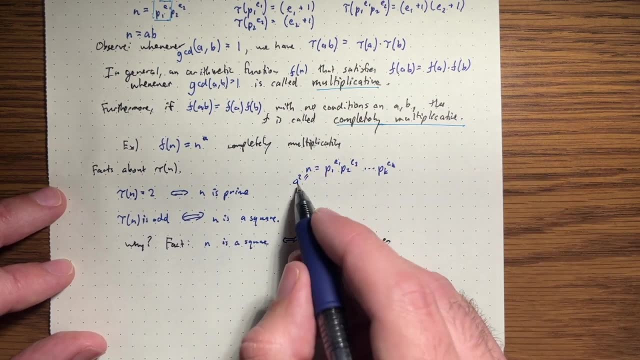 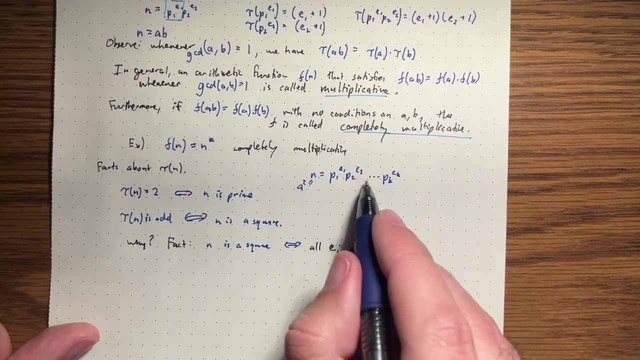 Okay, so all of these EI's are even. Why is that? Well, if n equals the square of some number, a squared a itself has some prime factorization. But then when you square that prime factorization, you have to get this prime factorization by unique factorization. 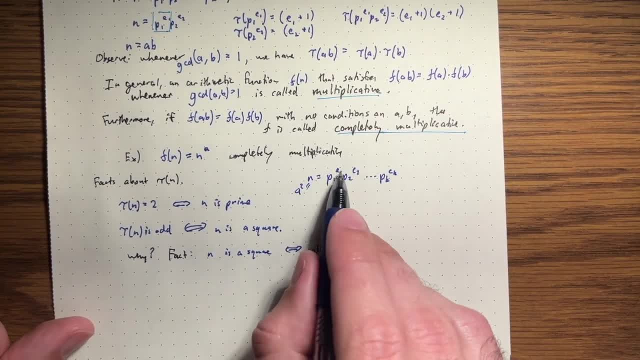 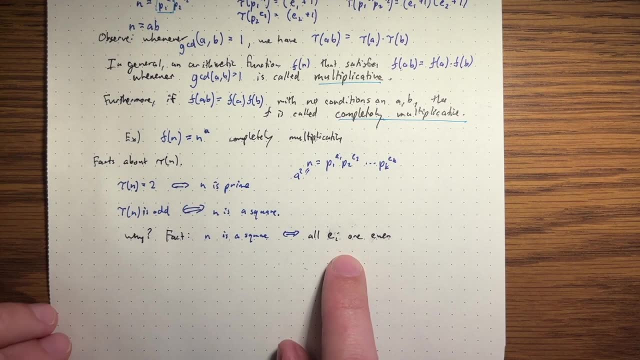 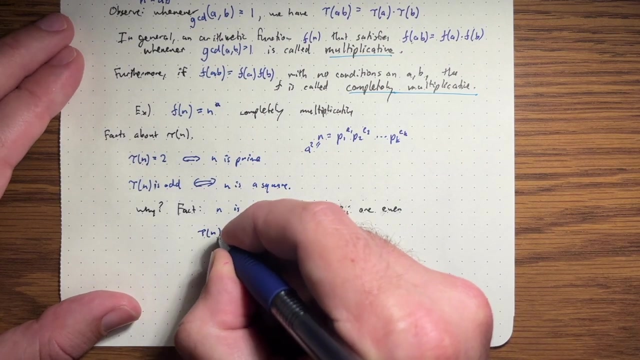 But I'm squaring it, So I'm essentially multiplying all the exponents by 2.. So these all are going to end up being even Okay. well, What does that have to do with tau of n being odd? Well, let's just look at a formula for tau of n. 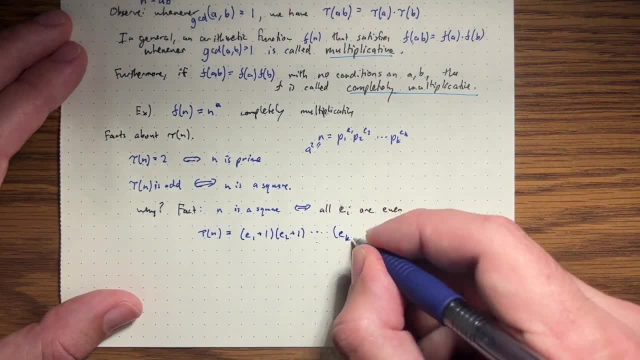 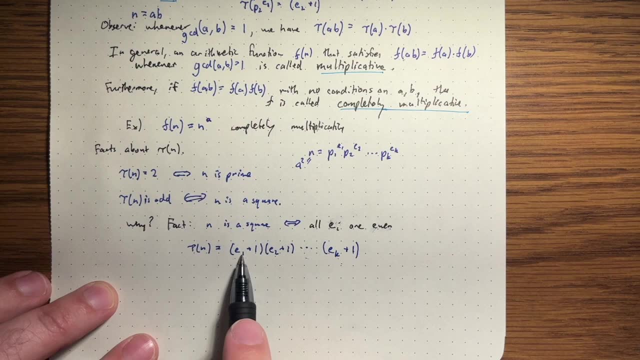 e to the plus 1.. You add 1 to all the exponents. multiply them together. Well, if all the EI are even, certainly this is going to be odd. We're going to get a product of a bunch of odd numbers, which is odd. 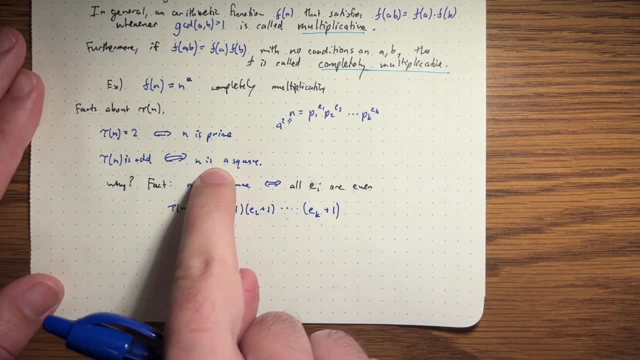 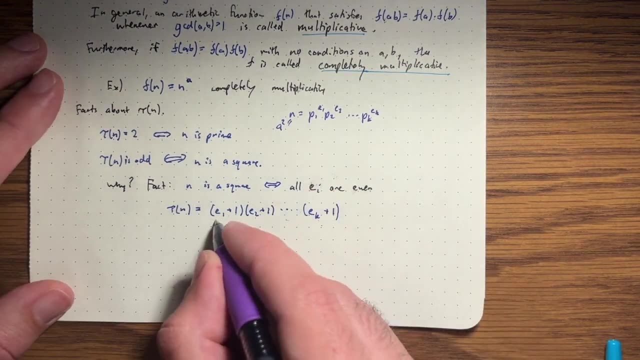 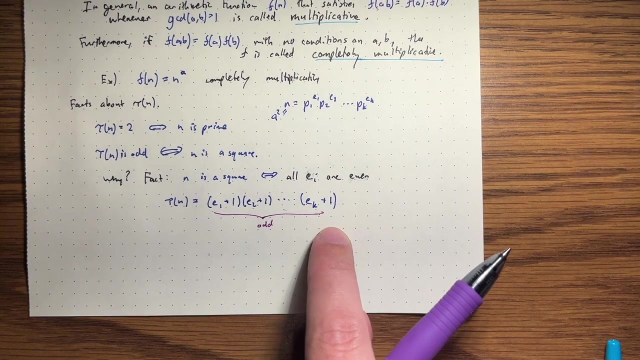 Okay, so that's this direction. Let's suppose tau of n is odd. So what if this whole thing is odd? This whole thing is odd. What can we conclude? Well, you know, if any one of these factors See, we've written tau of n as a product. 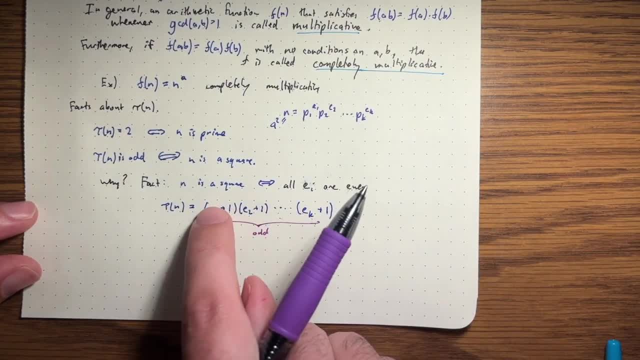 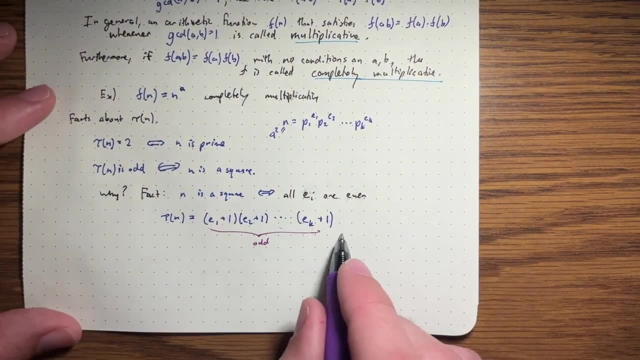 That's a very useful thing to do- a product of integers, And if any one of these factors were even, that would mean the whole thing is even right. So if this whole thing is odd, that actually means every single one of these has to be odd. 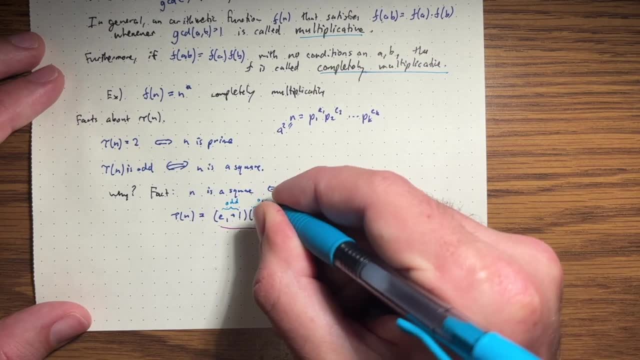 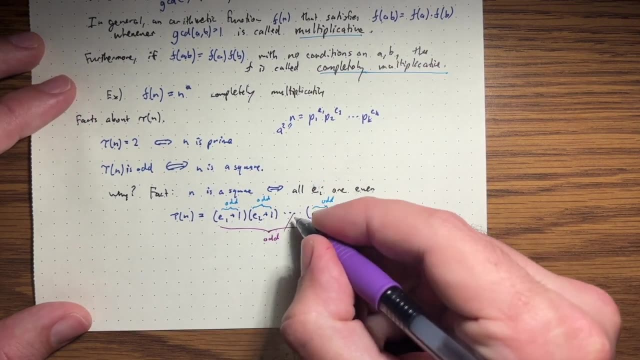 So this has to be odd, This has to be odd, Everything has to be odd, And that means: So see, the whole thing. being odd implies all these are odd. Now, if all these are odd, that means all the EI are even right. 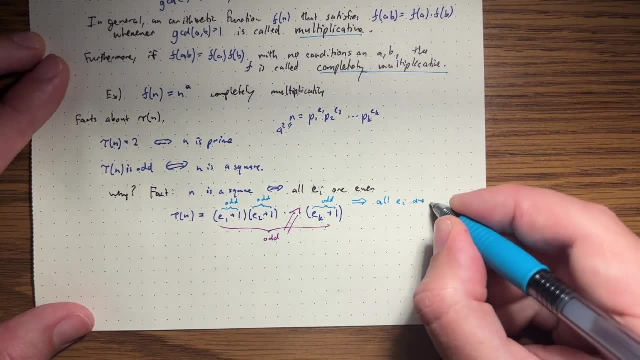 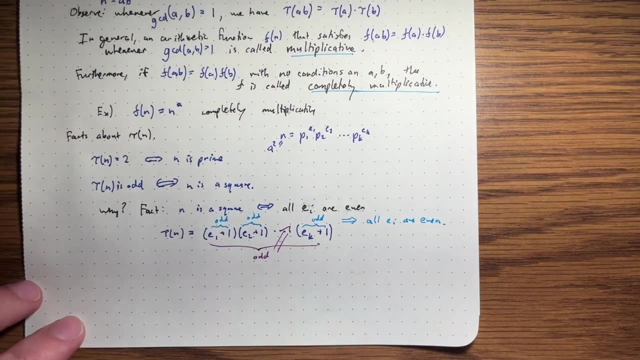 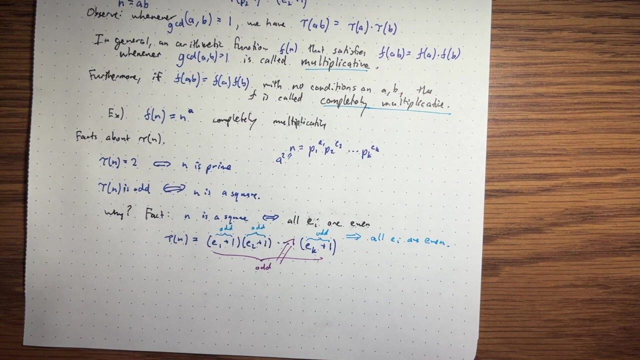 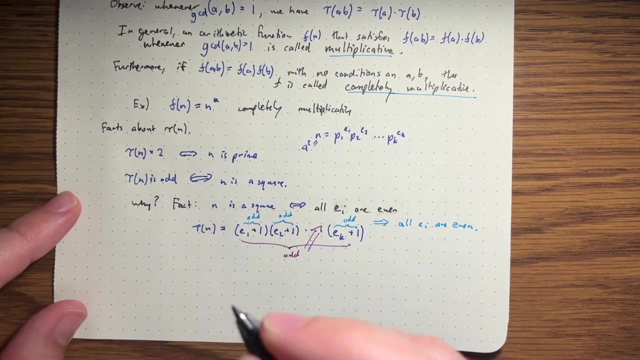 Because EI plus 1 is an odd number. But by our fact right, that's going to be a square, So we've proven this. So tn is odd exactly when n is a square. Okay, let's do a quick computation. 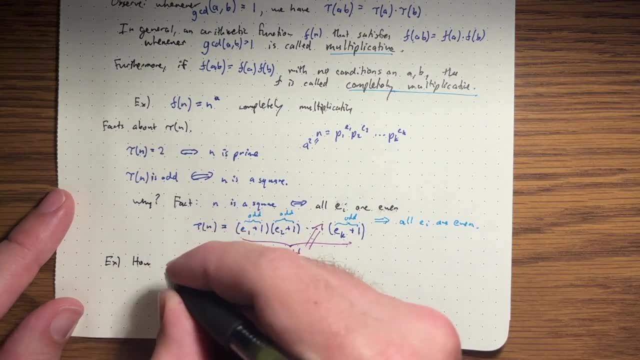 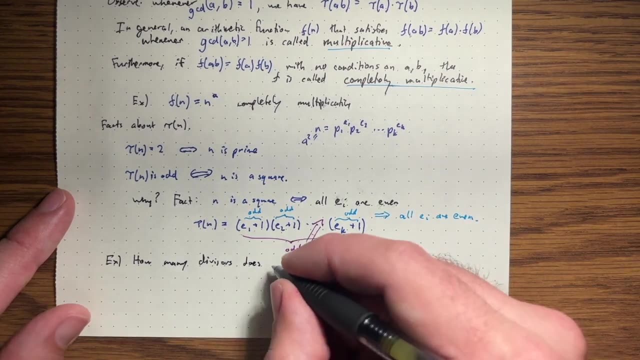 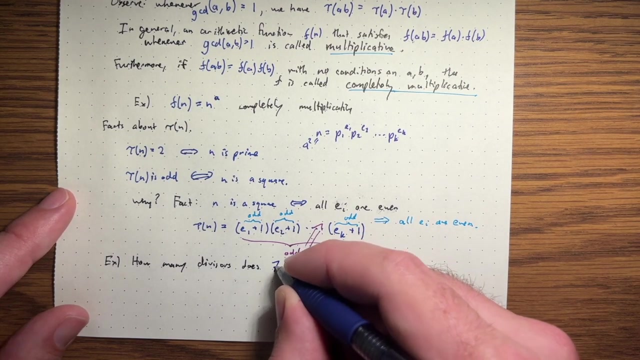 So here's a good example. So how many? Let's just show how useful this is. So how many divisors does the number? Let's pick something with a lot of divisors, A factorial maybe. Let's do 720.. 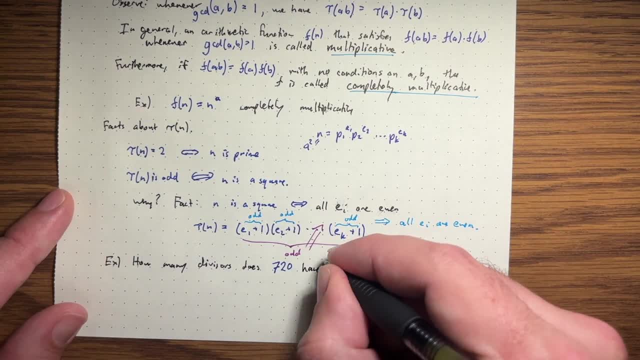 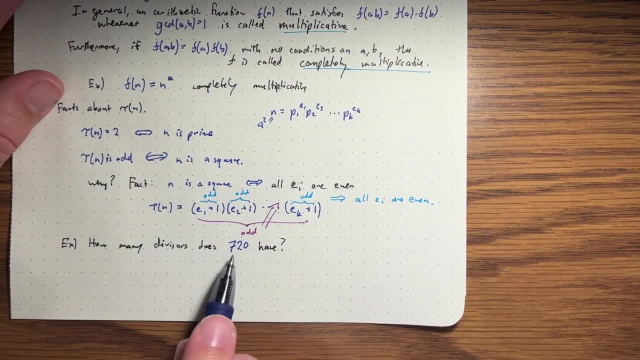 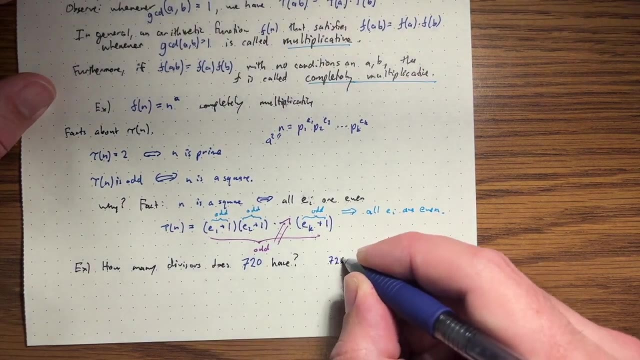 That's 6 factorial. How many divisors does the 720 have? Okay, well, let's find the prime factorization first. That's definitely going to be the right approach here. So 720 is Let's see. there are a bunch of 2s that we can pull out. 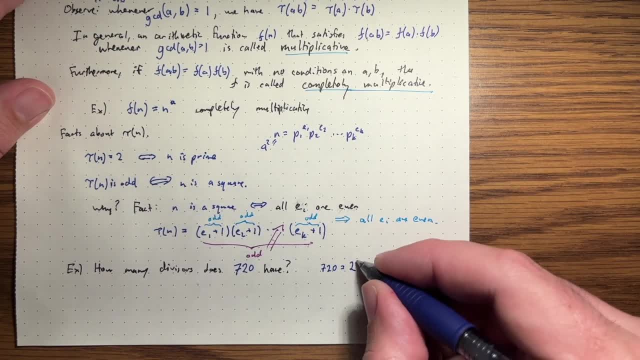 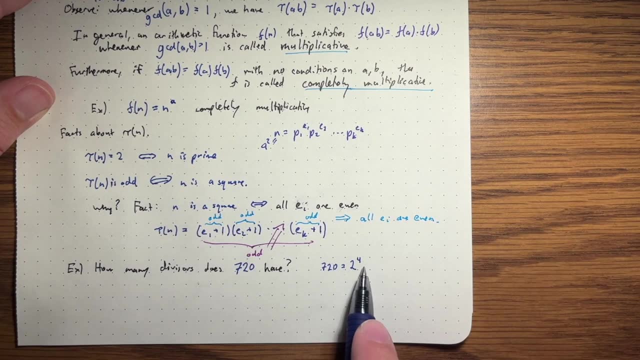 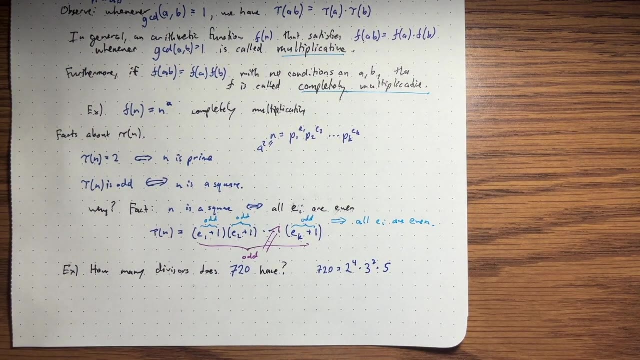 Let me think. So we're going to get 4- 2s and we're left with a 45. And so we're going to get 2, 3s and 1, 5.. So there's my prime factorization for 720.. 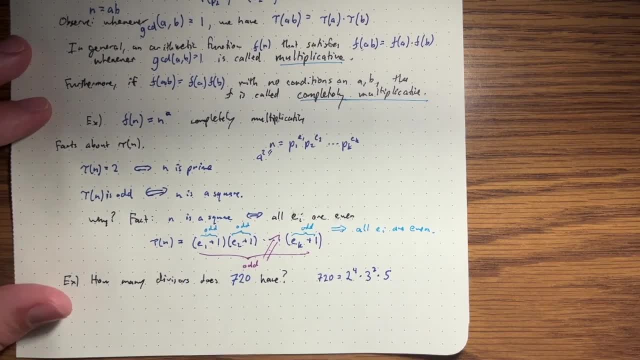 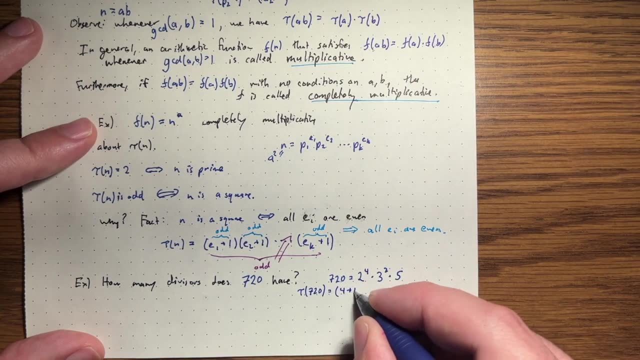 How do we count the number of divisors? Let's use this formula, All right, so the number of divisors, So tau, of 720, is going to be: I add 1 to all the exponents, 4 plus 1.. 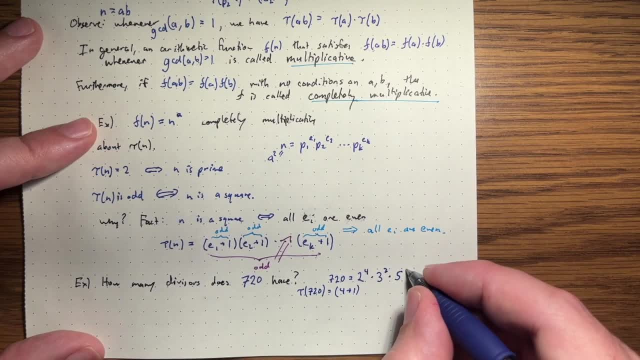 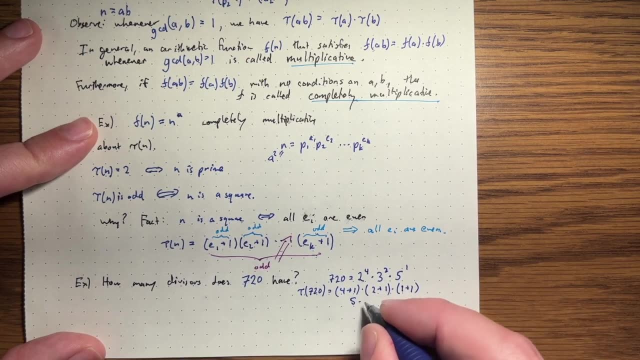 I don't even care what the primes are, I'm just looking at the exponents here and the prime factorization 1 plus 1.. So this is what 5 times 3 times 2, which is 30. So 720 has 30 divisors. 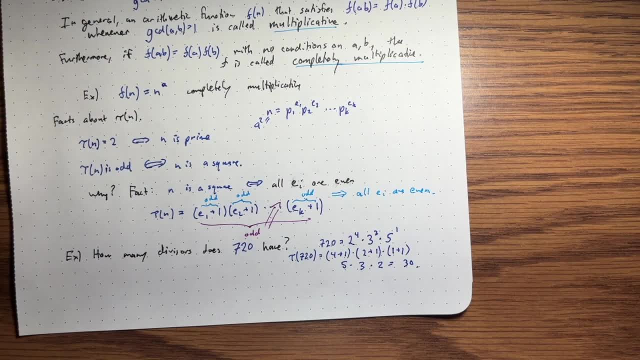 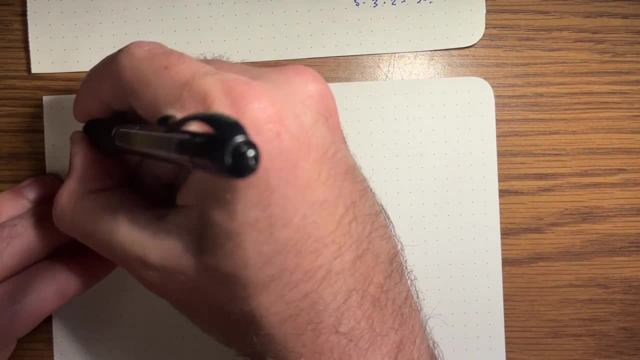 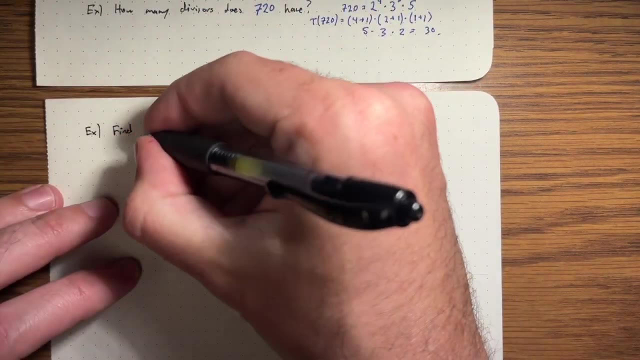 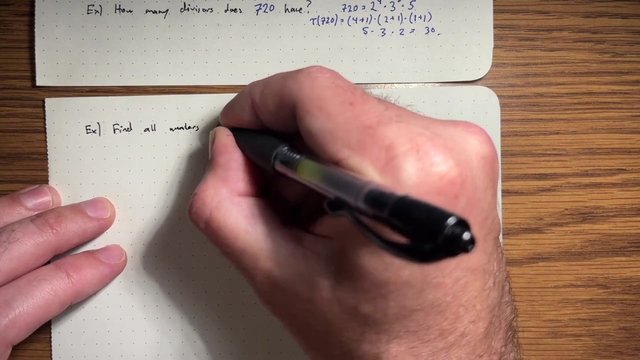 That's quite a lot of divisors. Okay, let's go to another page. Here's a really fun kind of problem. So let's try to find- And it shows you how useful this formula is also. So let's try to find- all numbers less than or equal to, let's say, 100,. 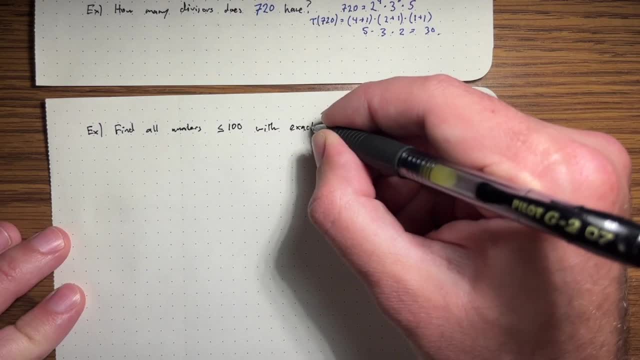 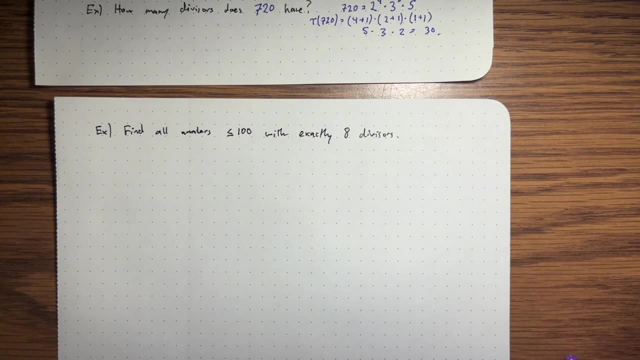 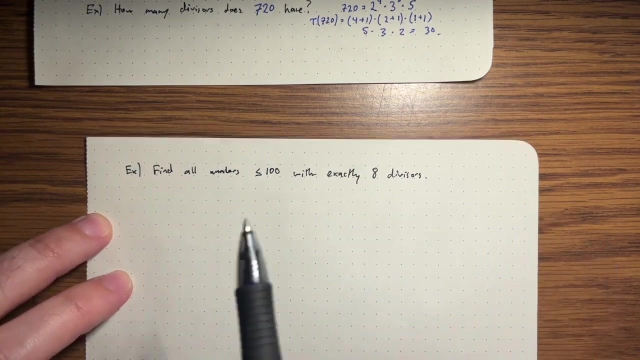 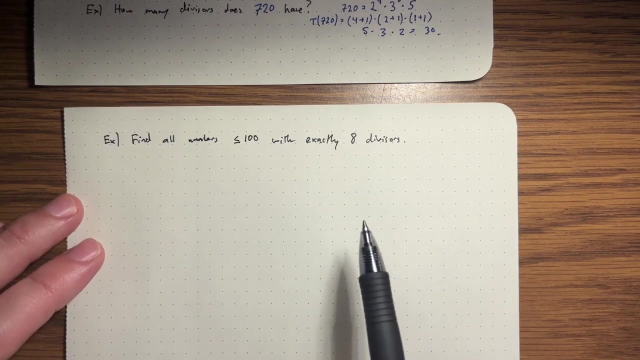 with exactly 8 divisors. Okay, Let's come up with a strategy first. So one strategy would just be to write down all the numbers. count the number of divisors, look at which ones have 8. That doesn't seem too efficient. 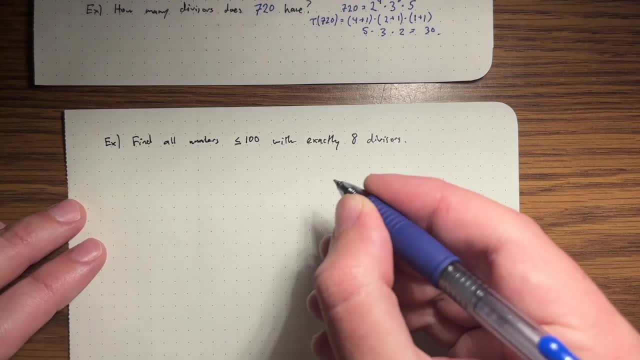 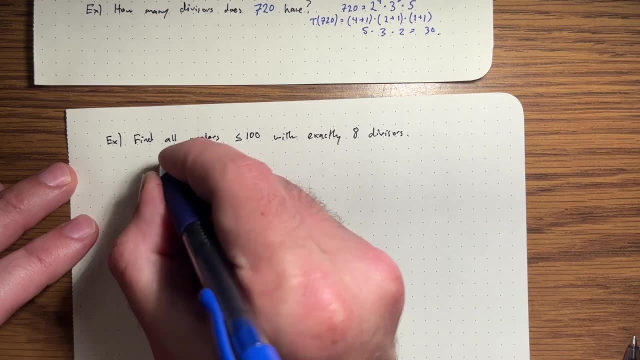 So what we can do instead is we can try to write down this formula. So tau of n- n is the number I'm trying to find. I want this to be 8, by the way. I want tau of n to be 8.. 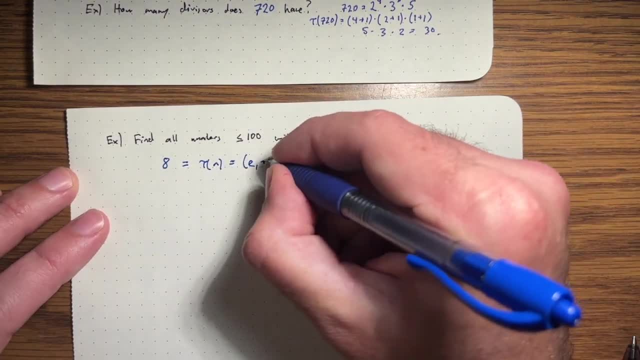 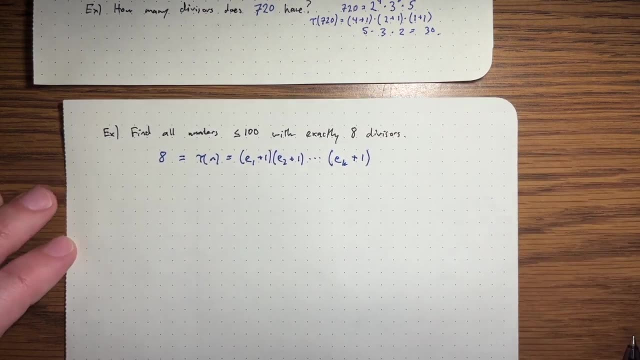 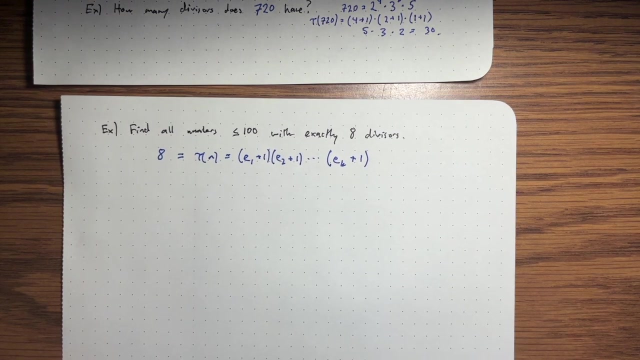 But we have a formula for this. But we have a formula for tau of n. It's just this product. But now we have a product of integers equaling 8. The positive integer is equaling 8. When you think about it, there aren't that many ways to do that. 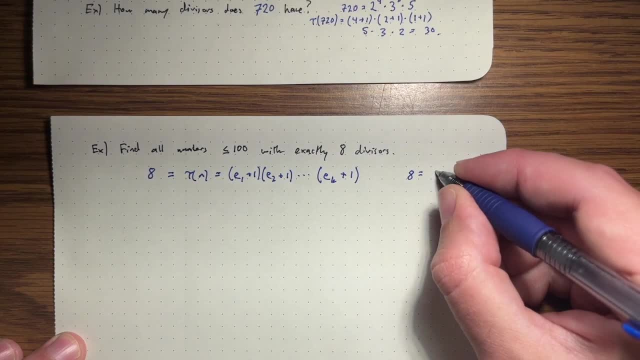 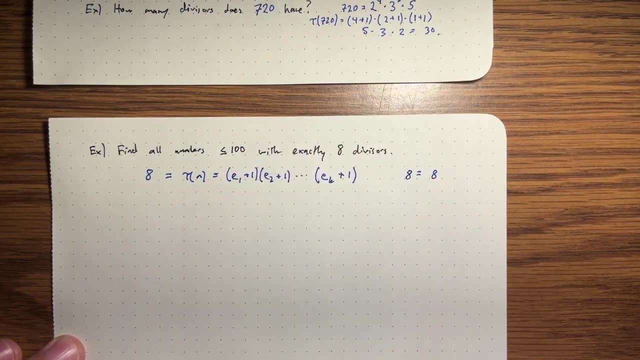 So we can have. 8 is Well, it could just be 8 itself. You can see one term here, The e1, I guess would be 7. Plus 1 is 8.. That could be all that we have. 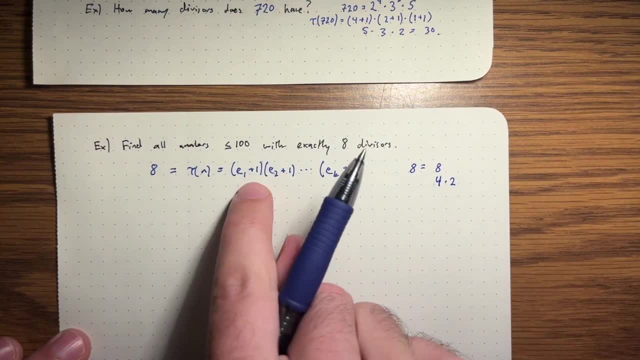 Or we could have a 4 times 2.. So one of these could be a 4.. One of these could be 2. And then we don't have anything else. Or we could have 2 times 2 times 2.. 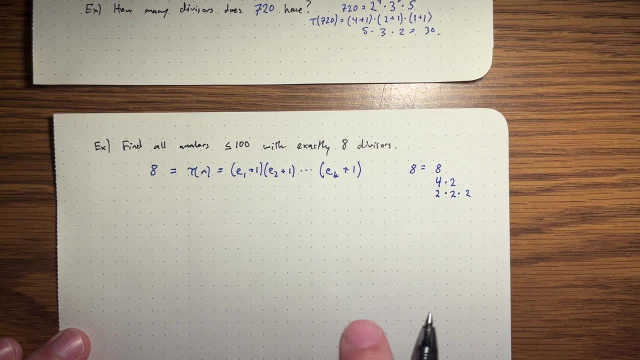 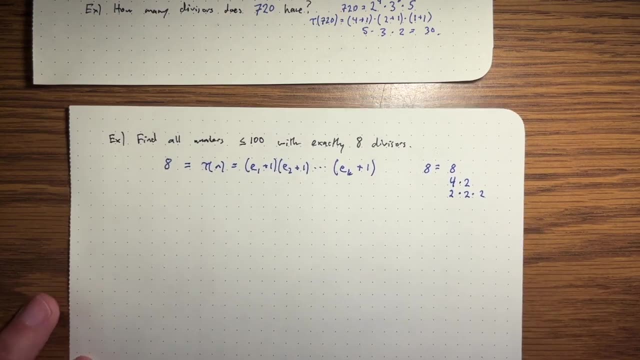 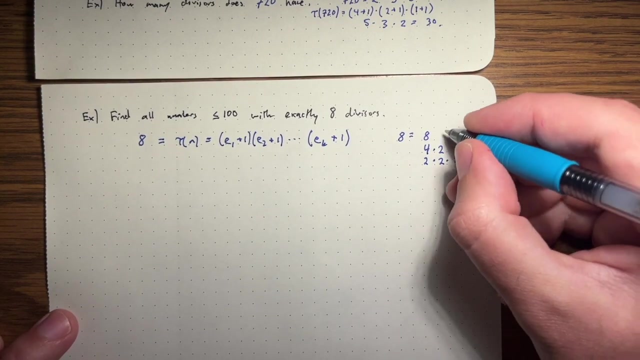 We could have three terms in this product, With each one giving me a 2.. So there are only a few cases that we have to consider here, So let's call this one case 1., Call this one case 2.. And this one case 3.. 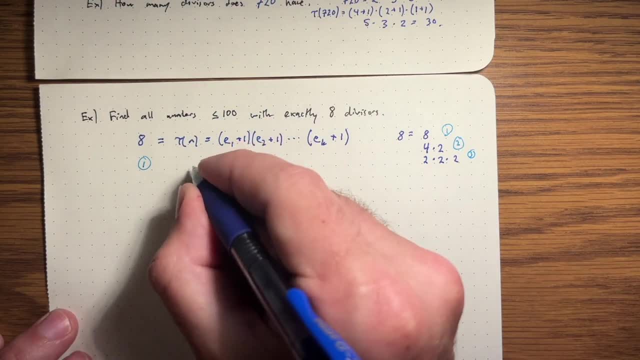 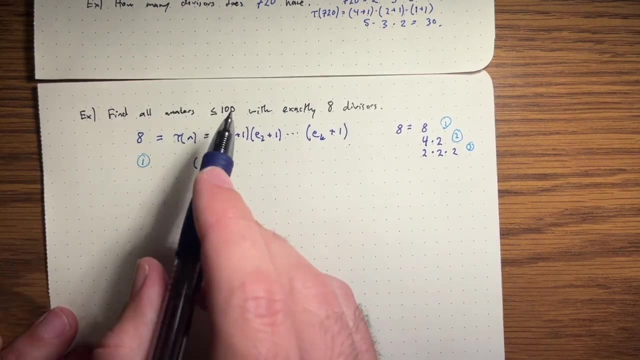 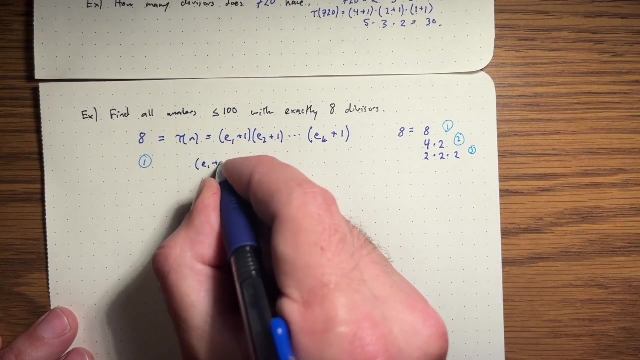 So case 1 first. Let's say, our factorization looks like this Of this side. here I'm not factoring any number in particular, I'm just looking at this formula. So we have e1 plus 1 equals 8.. 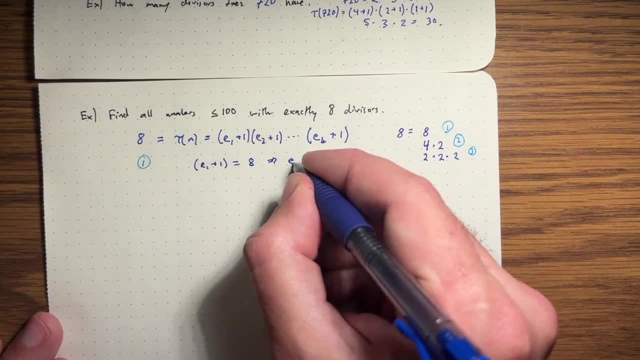 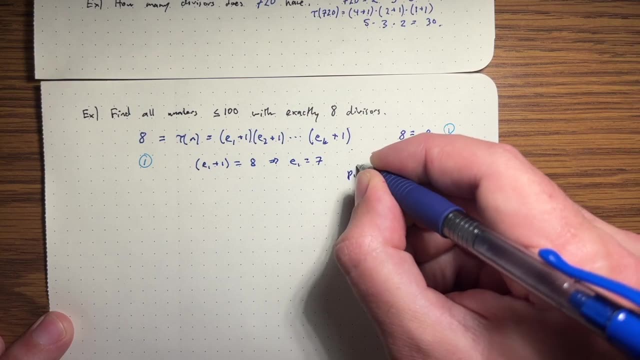 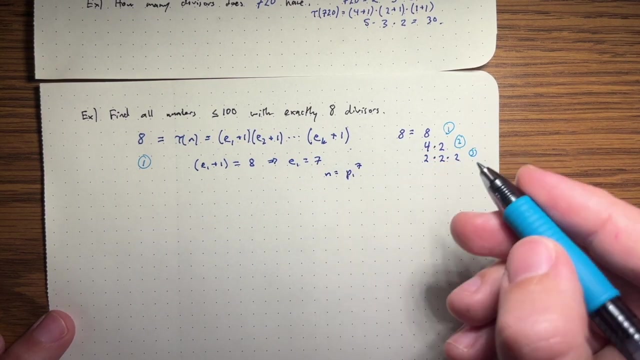 We just have one term equaling 8. That implies e1 has to be 7. So we could have 1 prime p1 to the 7. And that could be my number. n Well, is that possible? What if p1 is 2?? 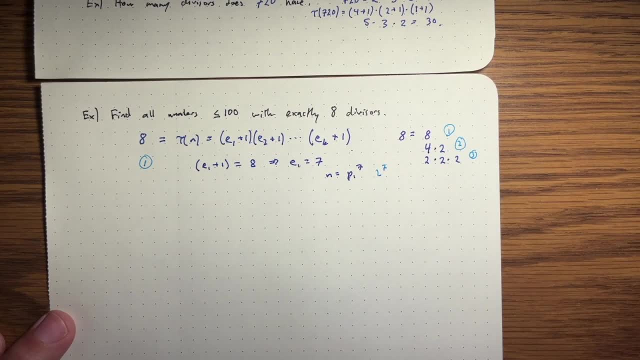 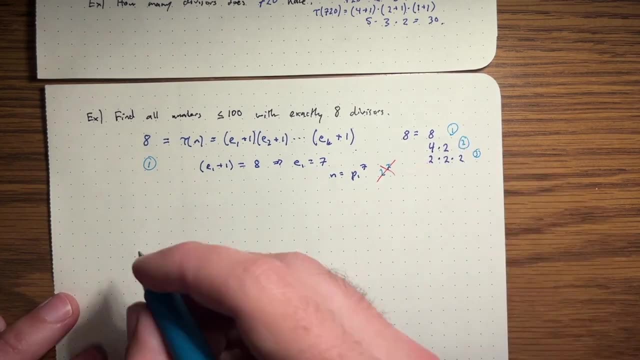 And we have 2 to the 7. I feel like that's over 100.. That's 128. So that's already too large. So 1 is not possible in this case. We could have another case. What if tau n? 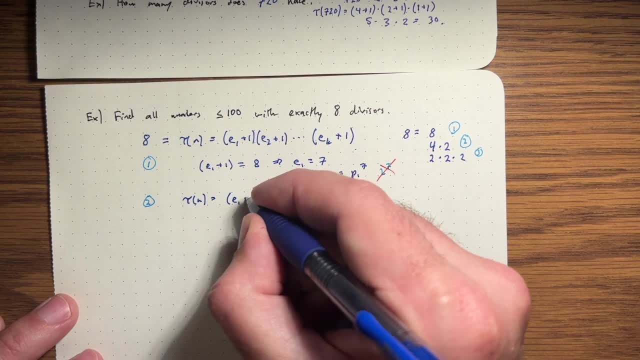 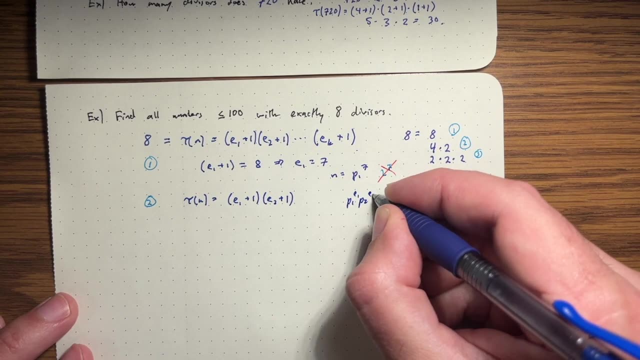 So we know it's equal to 8.. But what if it were equal to 8?? And this way, Where we have exactly 2 terms here, So we have 2 primes now: p1 to the e1.. p2 to the e2.. 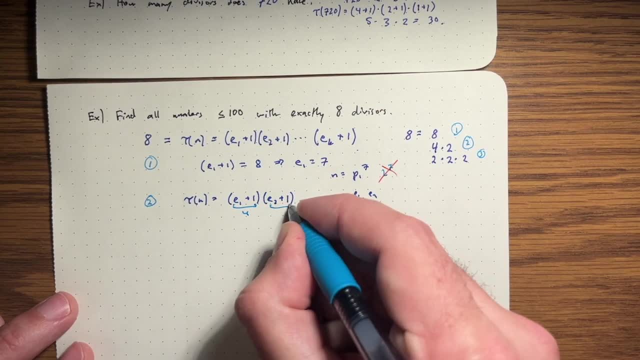 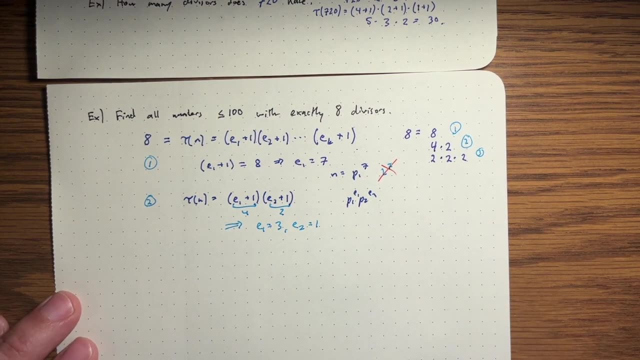 And let's say: this one equals 4. And this one equals 2.. Well, that implies e1 has to be 3. And e2 has to be 1.. So actually we're looking for factorizations of this shape. So we want p1 to the 3.. 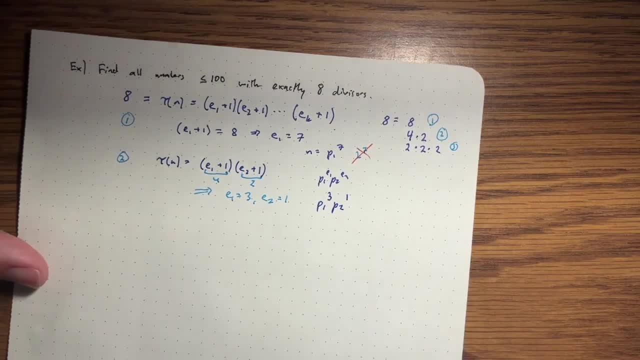 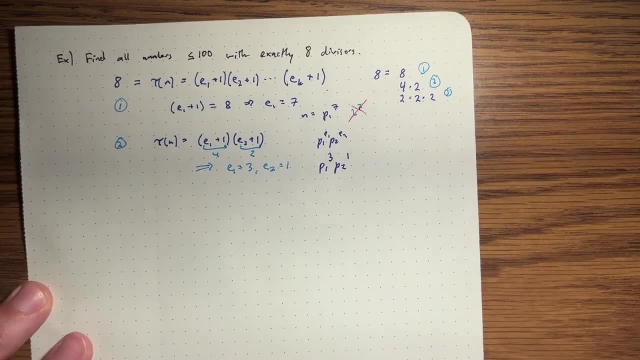 p2 to the 1.. So we're kind of working backwards, We're figuring out what the shape of the factorization is, Then we're generating the numbers really quick from that. OK, Well, let's just look at all the possibilities here. 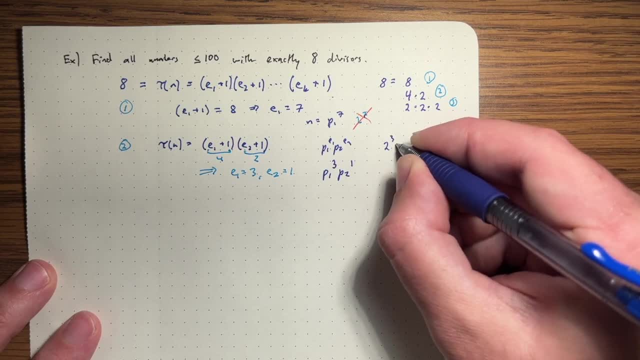 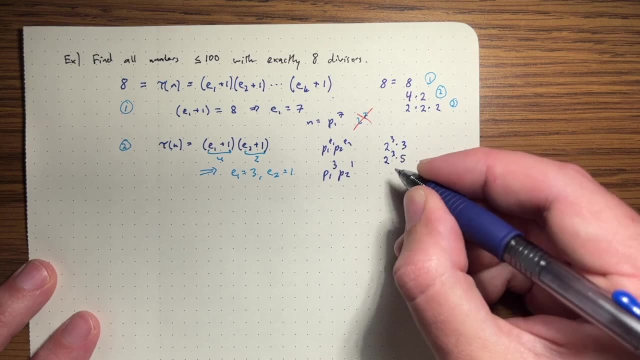 So p1 could be 2.. So I could have 2 to the 3 times. My next prime has to be to the first power, So I could have this. I could have this. I could have 2 to the 3 times 7.. 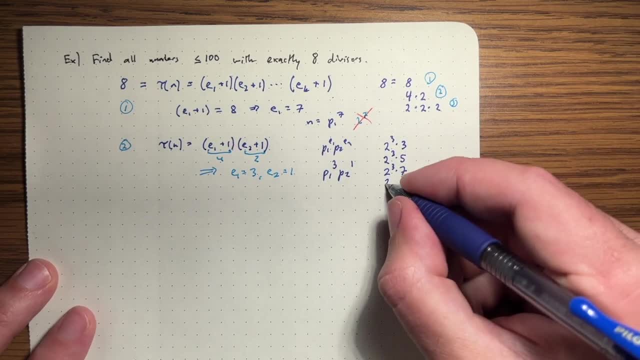 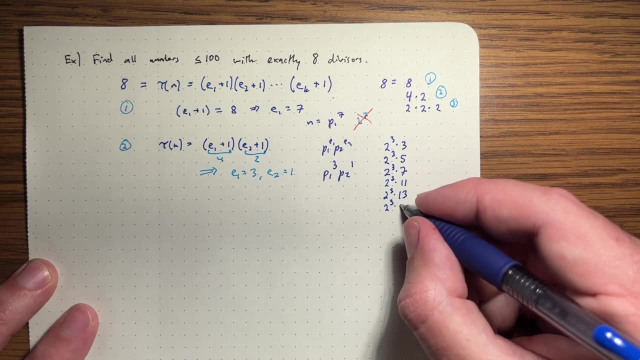 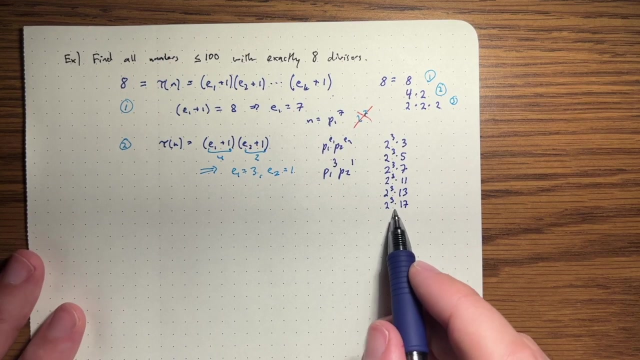 2 to the 3 is 8.. So these are all below 100.. We can keep going. 2 to the 3 times 13.. 2 to the 3 times 17.. Have I gone too high? Yeah, I think this one is actually 102.. 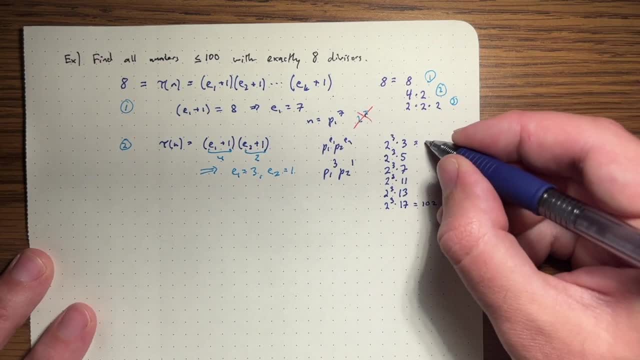 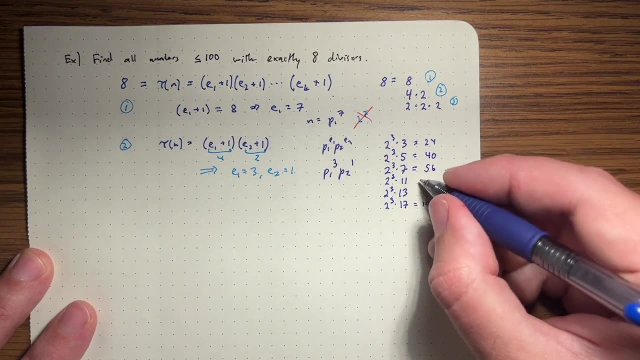 So that's too high. But what are these numbers? So 2 to the 3. So 8 times 3 is 24.. This one is 40.. This one is 56.. This one is 88.. Sorry about that. 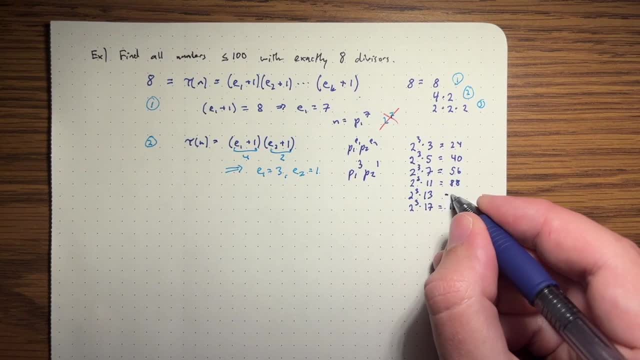 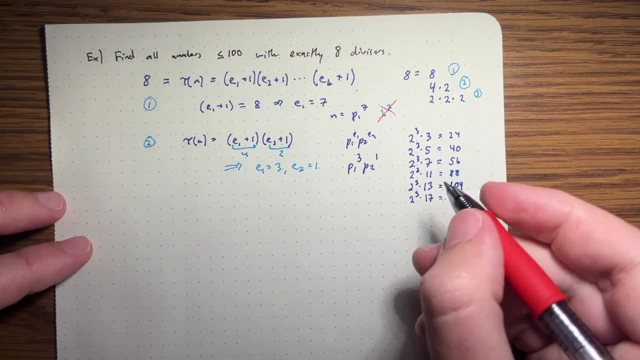 I think I got this one wrong. It should be 136.. And then this one here: 2 to the 3 times 13,, that's 104.. That's already over 100. So I don't need these last two. 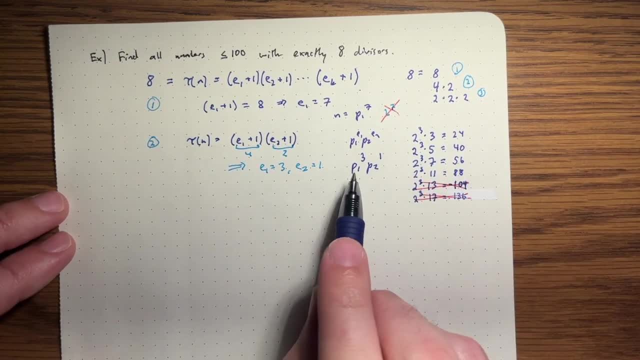 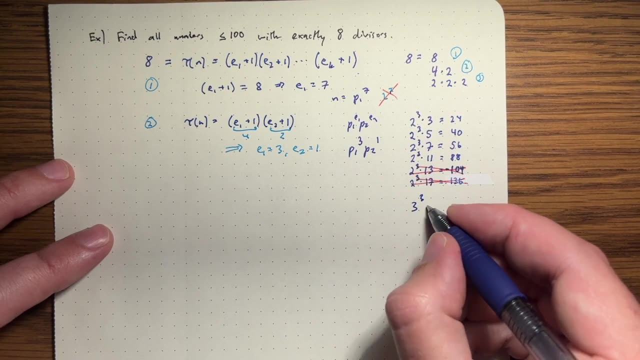 But I've produced four numbers here And I can actually keep going, because we don't have to take 2 for p1.. We could take 3.. So we could do 3 to the 3.. p1 is 3 now. 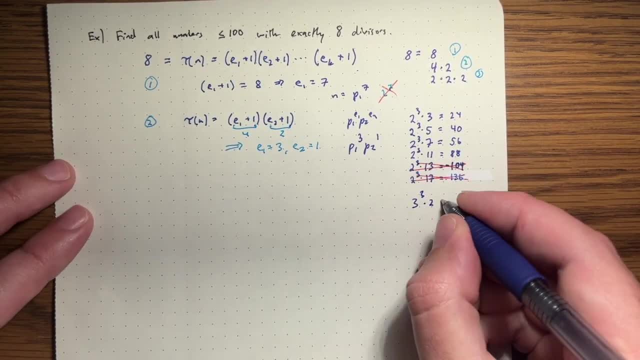 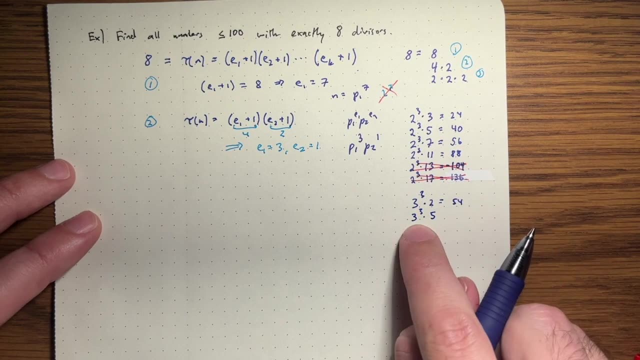 p2 can be 2.. That's not anything that we've done so far. So 3 to the 3 is 27 times 2 is 54. Then we could do 3 to the 3 times 5.. Notice, I'm not allowed to do 3 to the 3 times 3, because that would be 3 to the 4.. 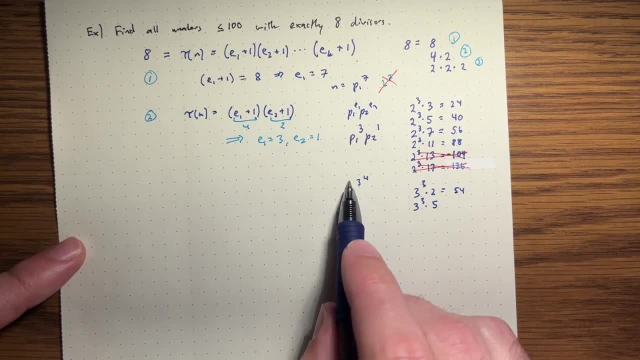 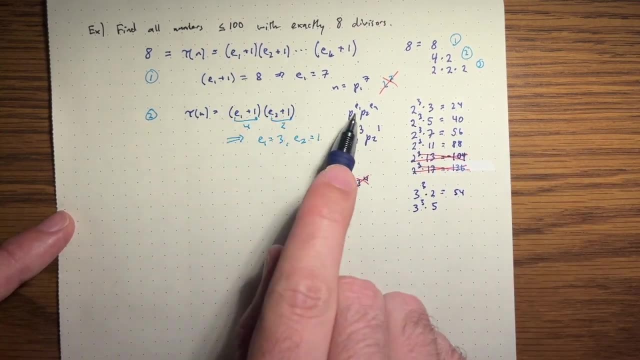 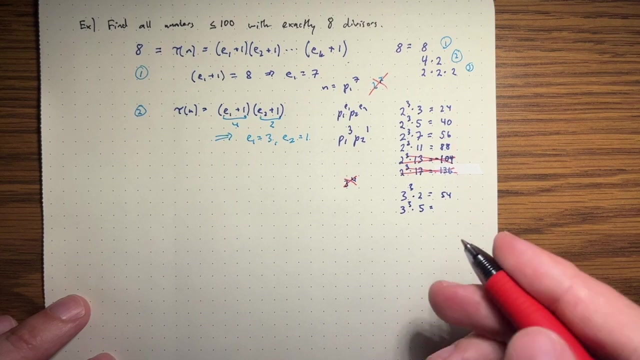 That would be a factorization of a different shape. This would actually have five divisors, not eight. I need distinct primes if I want to have a factorization like this. OK, Well, this one is already well over 100.. But I can do 54.. 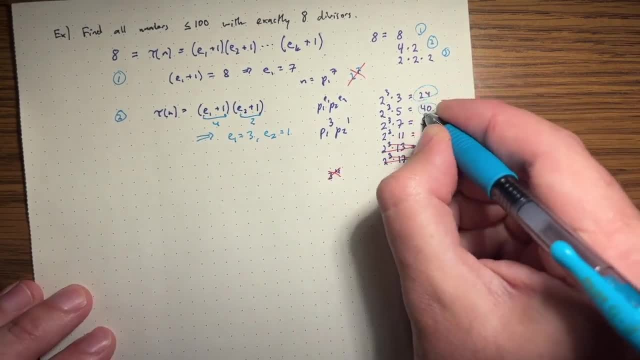 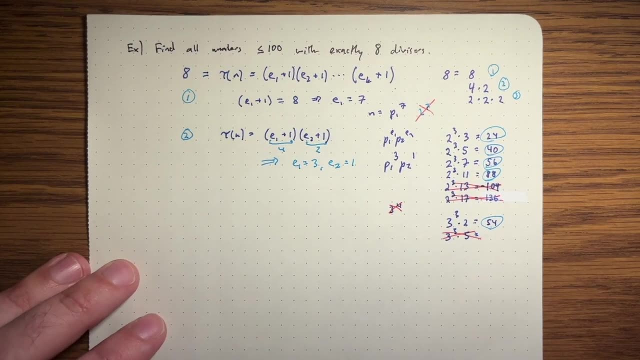 I'll circle the numbers that we're getting. If I do 5 to the 3, that's already over 100.. So I'm done with all the factorizations of this shape. Now we can look at the third case. What if tau van? so it's equal to 8 again. 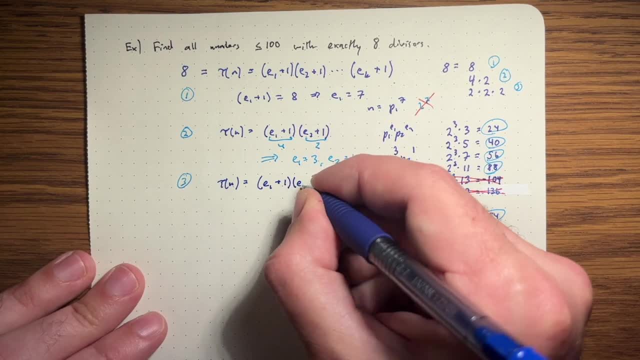 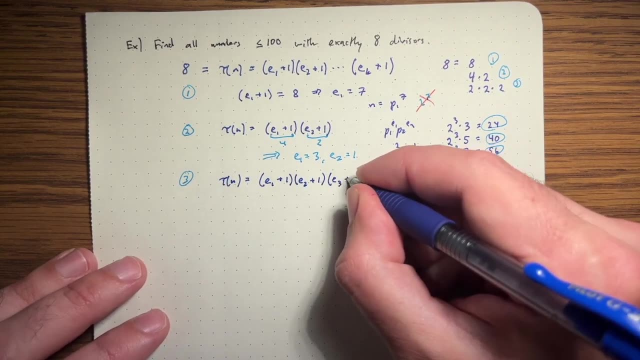 But what if it were equal to 8? in this way, I have three factors of 2.. These are the only three cases, because I have a product of things equaling 8.. Um, You might also say, well, why can't I add like a times 1 onto one of these? 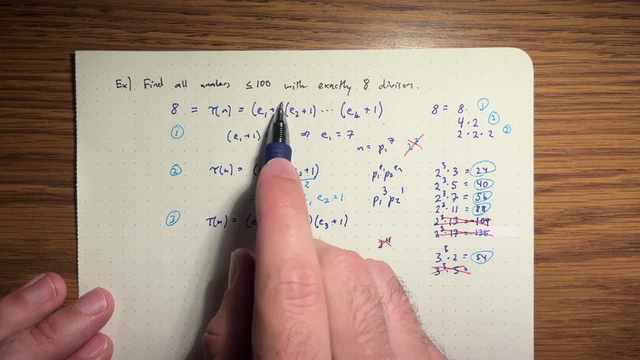 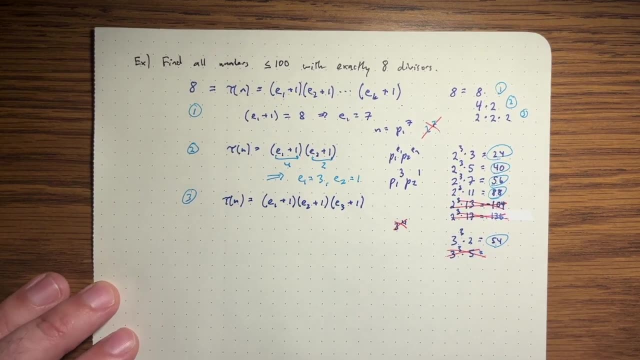 And I can. But then I would just get these factors of 1.. And if one of these equals 1, the EI would correspond to it would just be 0. So it's not really giving me anything in the factorization. So in this case, we want this to be 2, this to be 2, this to be 2.. 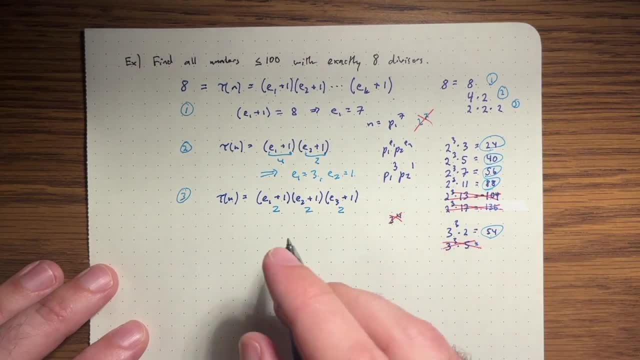 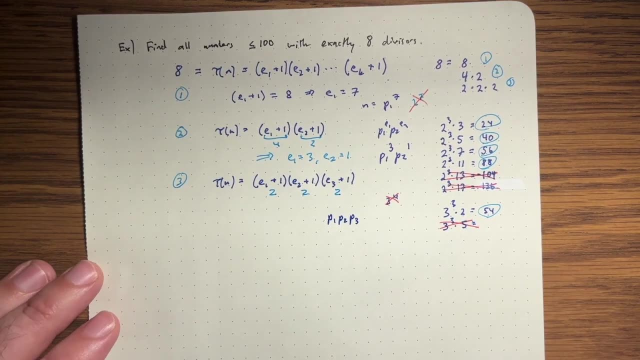 So that means we just have all the EIs equal to 1.. And we're going to look for factorizations of this form: P1, P2, P3.. It's all the first power. OK, Let's try to find some of those. 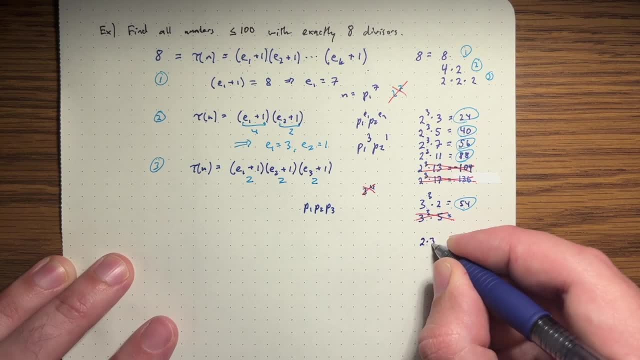 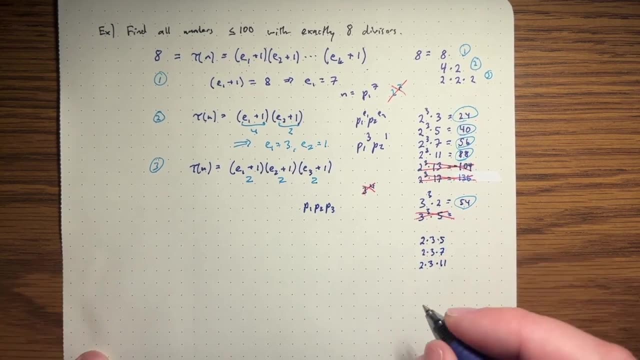 So come over here again. So we have 2 times 3 times 5.. That works 2 times 3 times 7.. 2 times 3.. I'm keeping the first two the same and just seeing how high I can go with the third one. 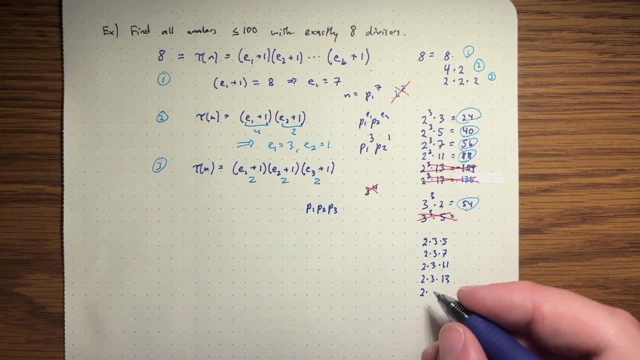 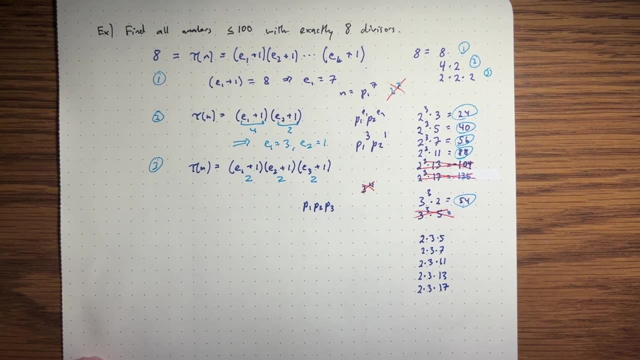 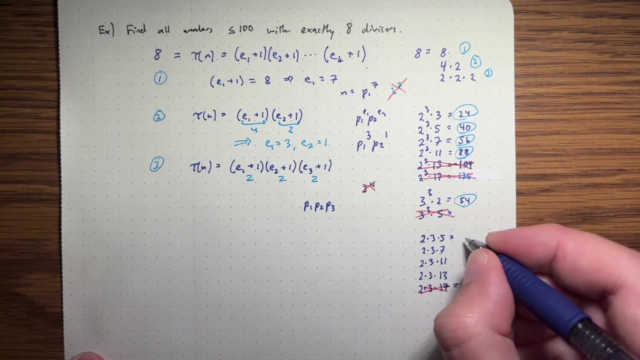 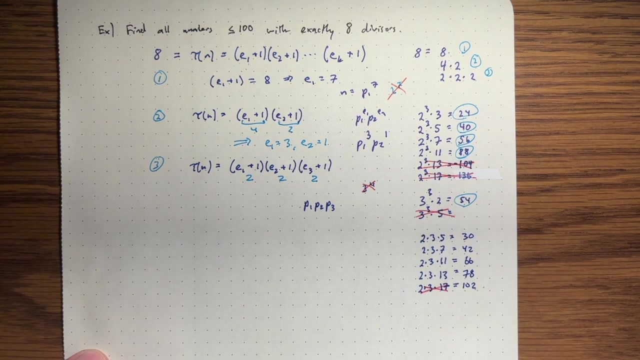 2 times 3 times 13.. 2 times 3 times 17.. That one should already be over 100.. That looks like it should be 102.. So we can certainly take all of these. So this is 30,, 42,, 66,, 78.. 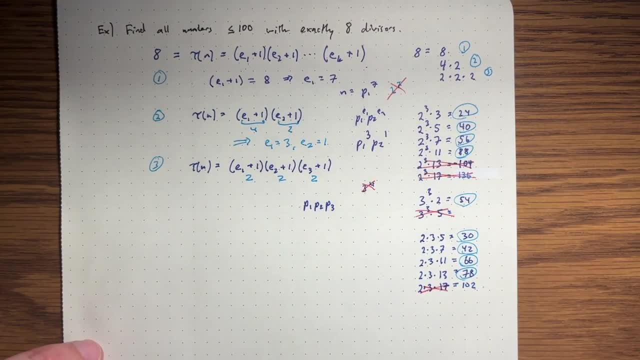 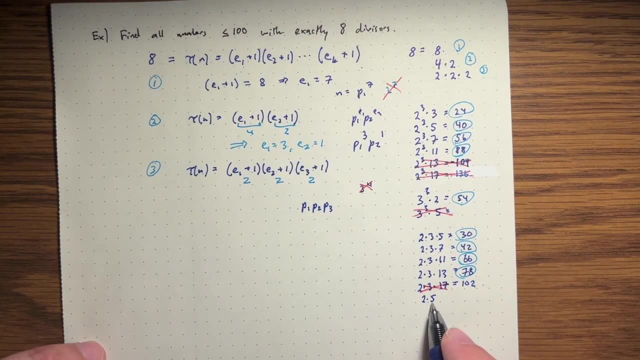 We've produced four more numbers with exactly eight divisors. OK, So we've gone as high as we can here. Let's try varying the second prime instead. So we'll do 2 times 5.. I can't do times 5 because that's a different factorization. 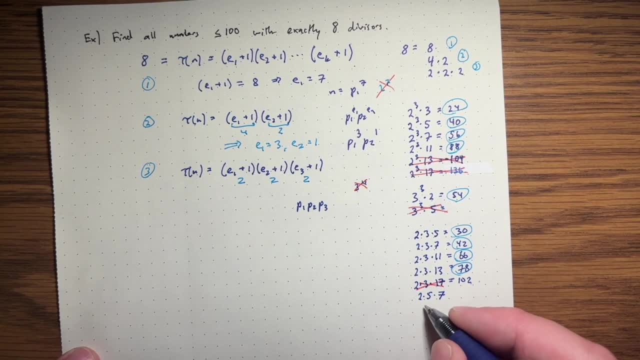 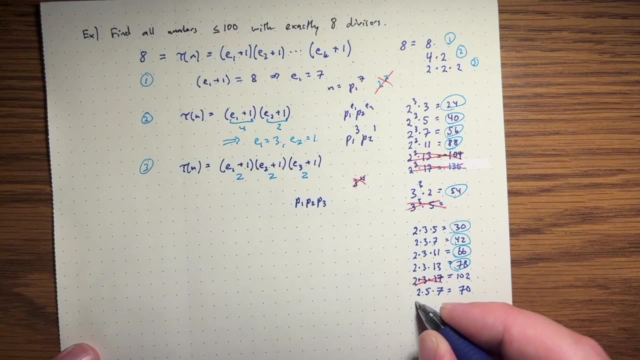 2 times 5 times 7.. I'm allowed to do that. And 2 times 5 times 11, but that's already too high, So it's going to be 70. And then I can do 2 times 7 times something higher than 7, but it's already going to be too high. 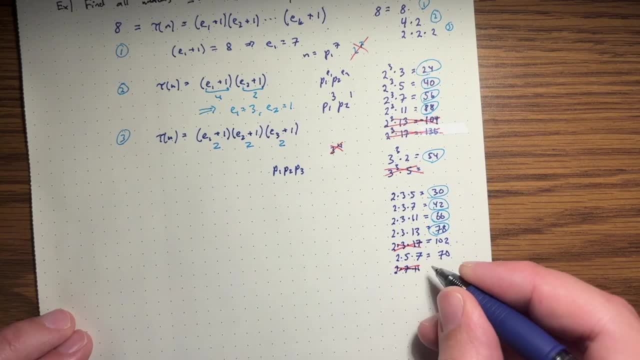 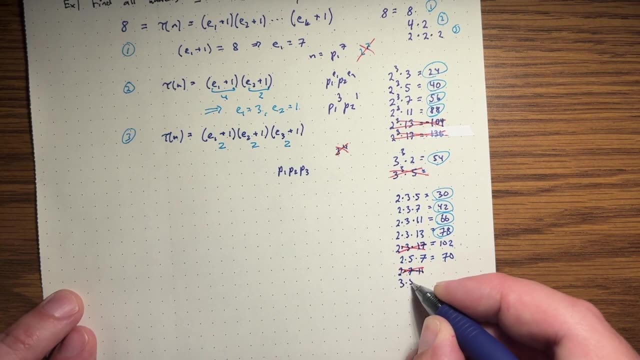 I'm only looking for ones less than or equal to 100.. Well, what else can I do? There's not much. I suppose I can start with the third, So I can do 3 times 5 times 7. Just taking small primes as I can. 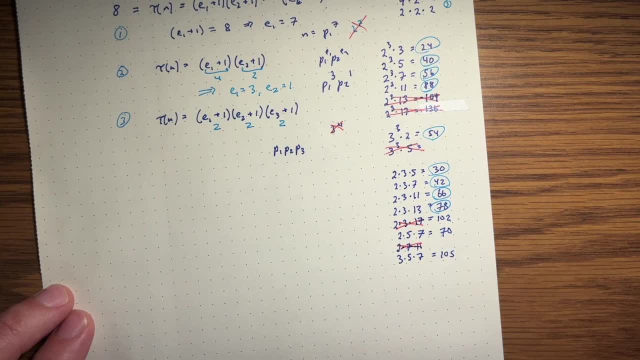 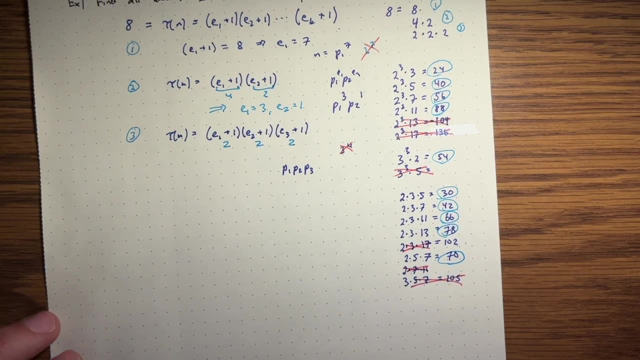 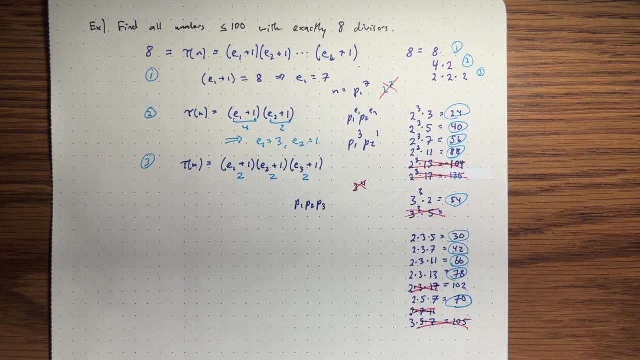 And this one's already over 100.. So I think we're done. I think we've found all of the numbers less than 100 with exactly eight divisors. There's these ones here. So Bill agreed that's a pretty efficient way to generate these. 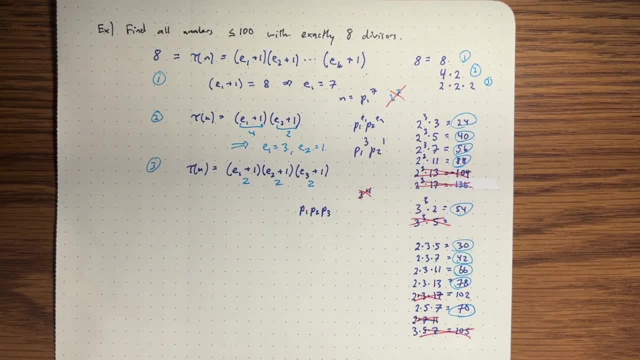 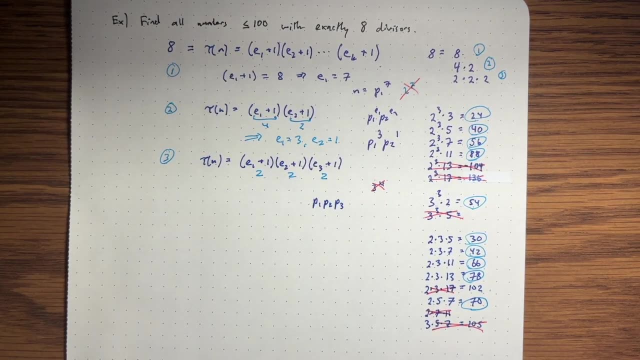 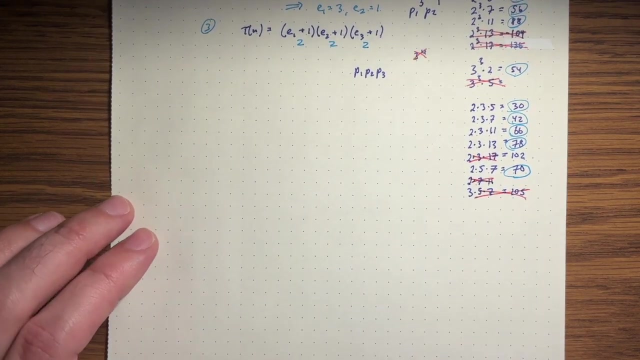 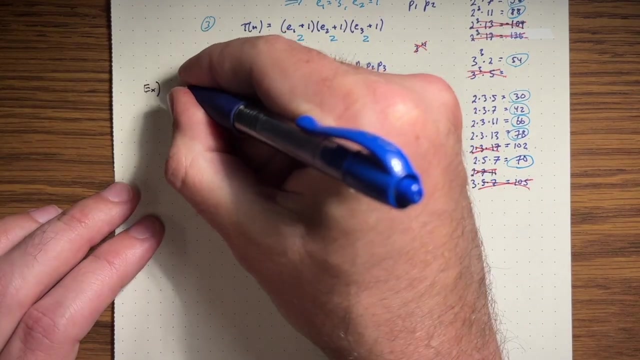 Take advantage of the fact that we have a product equal to this, And this is telling us sort of the shapes of the factorizations we need to consider. OK, Well, let's move on to our next multiplicative function. So this will be our next arithmetic function. 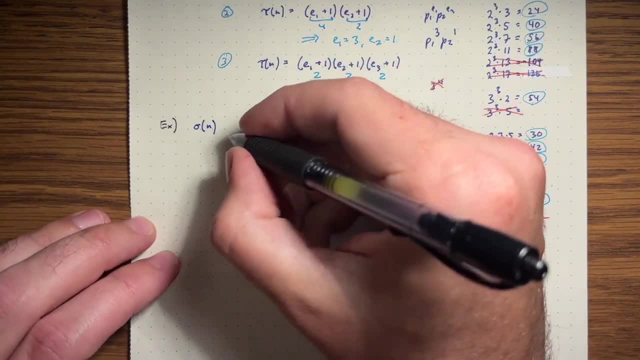 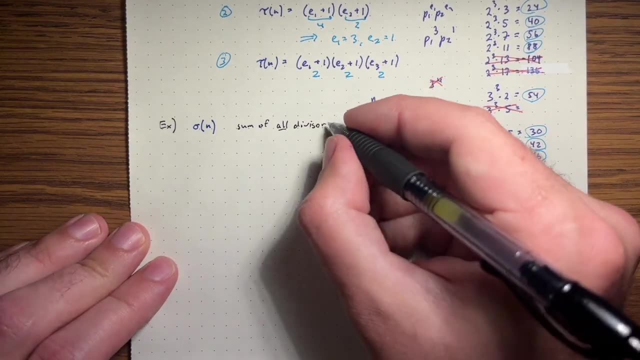 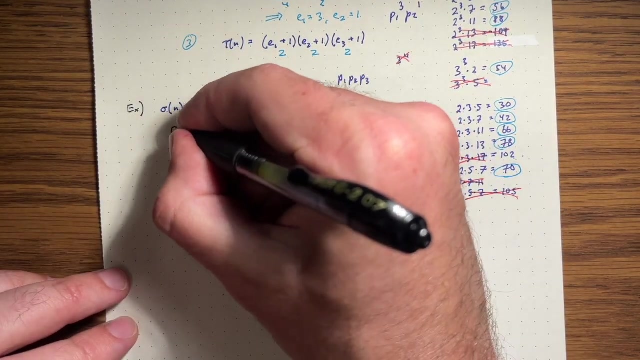 It turns out to be multiplicative as well. This one is called sigma of n. This is the sum of divisors, Sum of all divisors, All the positive ones at least. So sum of all divisors of n. Let's do an example. 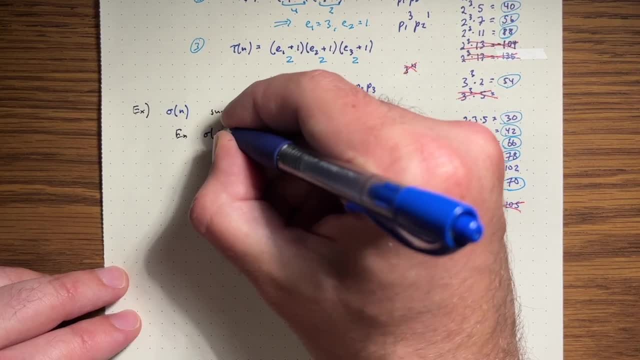 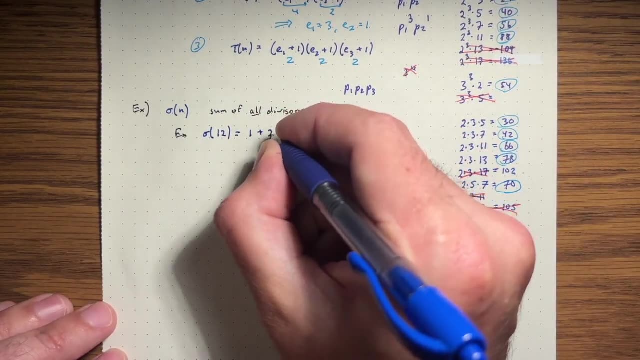 So sigma of 12.. You're going to think sigma means S for sum. That's how I remember that. So you're not counting them, You're taking a sum And add up all the divisors of 12, including 12 itself. 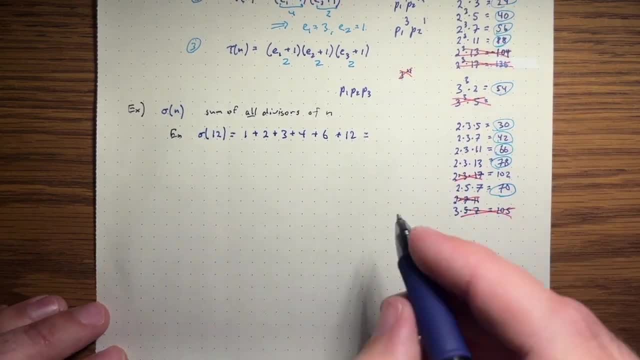 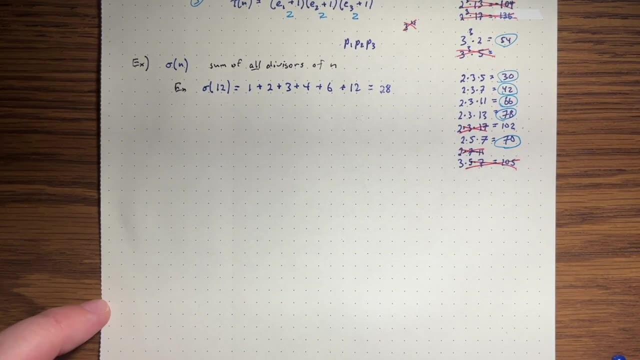 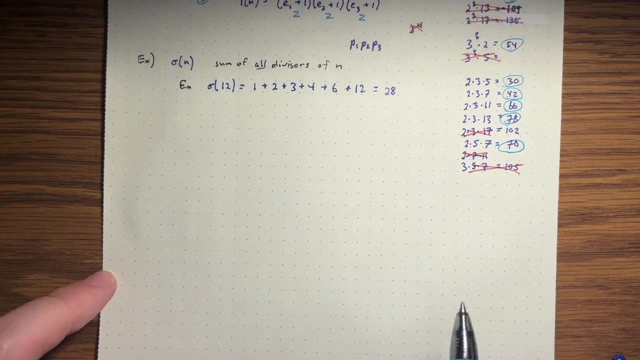 So I don't want just the proper ones, I want all of them. 16 plus 12 is 28.. So sigma of 12 is 28.. Let's think about how we can maybe calculate this in general, Because it would be nice if there were a formula, just like we had for tau. 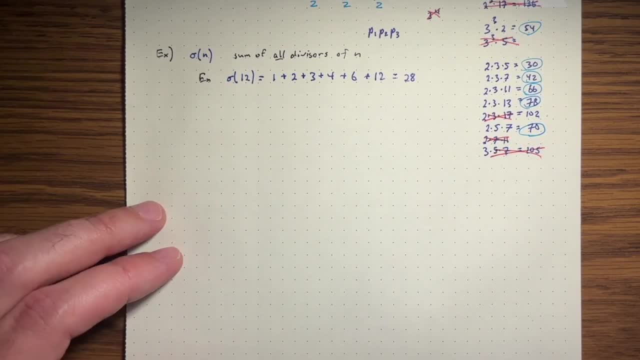 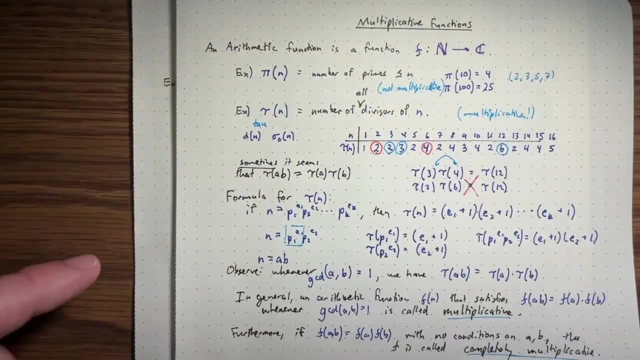 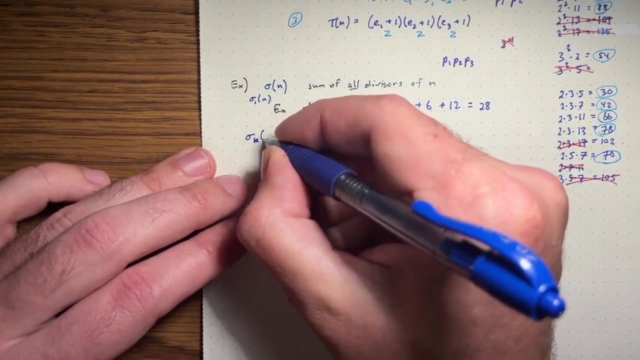 Before we do that, I just want to mention some notations. So this one is sometimes also called sigma 1 of n. So I said before that tau is sometimes called sigma 0. So what's the meaning of that? So we define sigma k of n to be the sum over all the divisors. 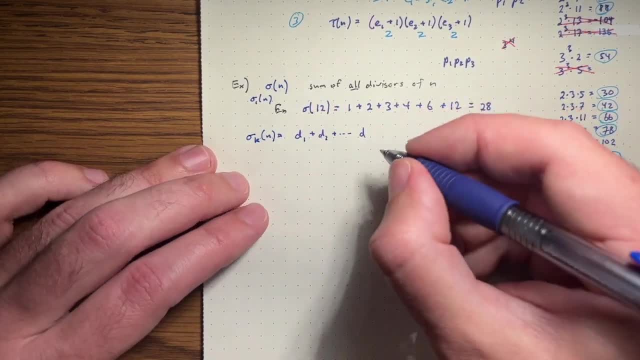 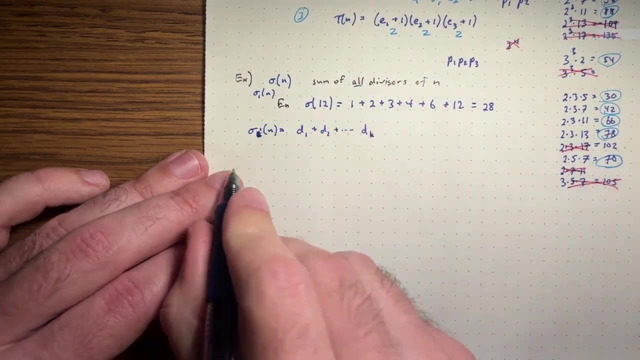 So I'll just denote those d1, d2.. Let's call it sigma i of n, because I usually use k to indicate the number there. So sigma i of n is the sum of all the divisors, but each one you're raising to the i-th power. 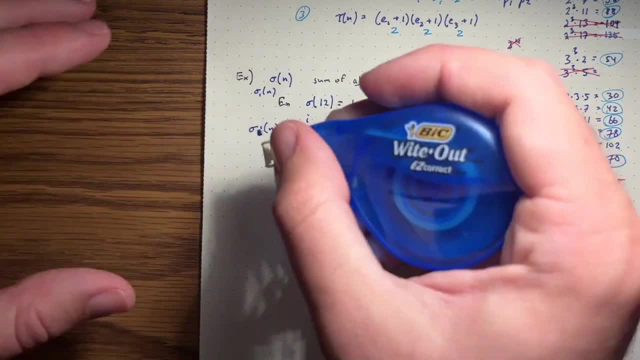 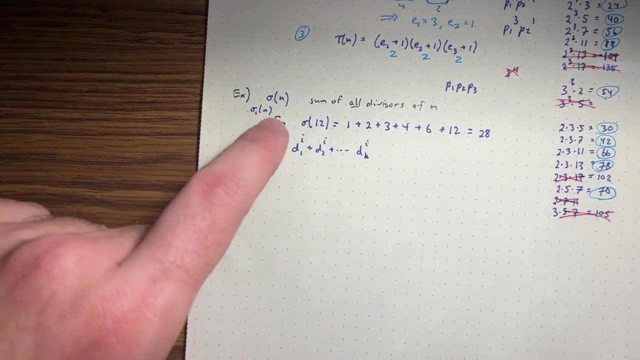 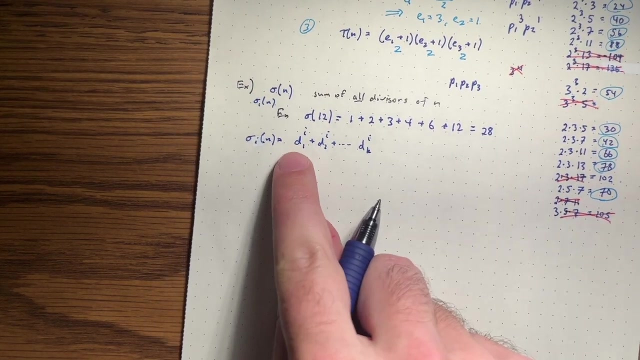 This turns out to be a useful thing that we might want to look at. So if you take i to be 1, you just get the sum sigma. If you take i to be 0, you get just a 1 for each divisor. 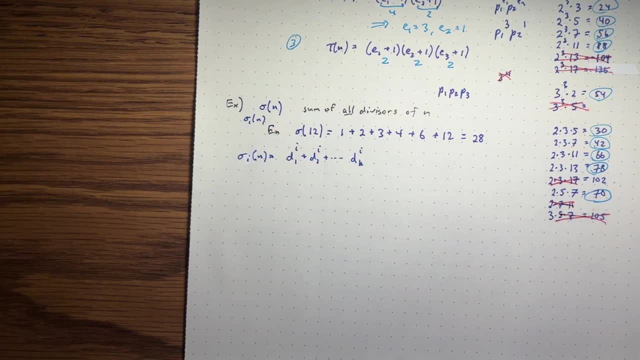 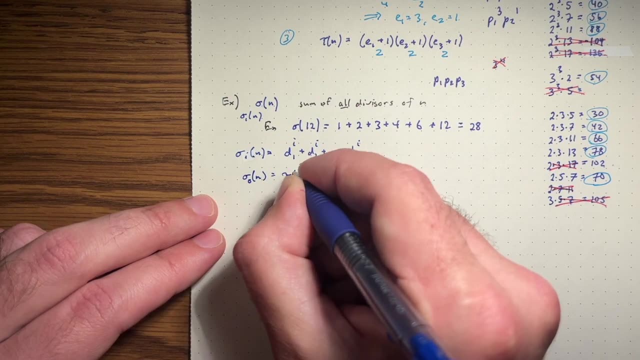 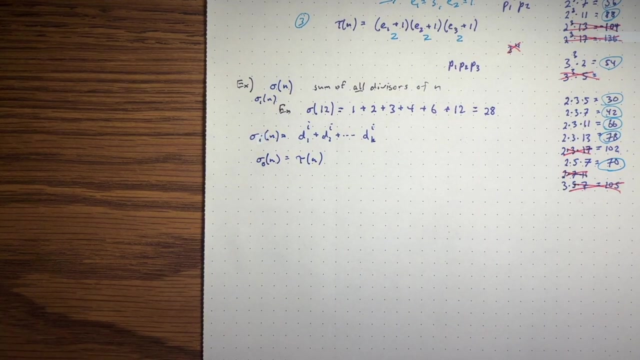 So essentially you're counting and then you're adding them all up, adding up all these ones. So this one is just sigma 0 of n, is just tau. Sigma 2 of n would be sums of the squares, of the divisors, etc. 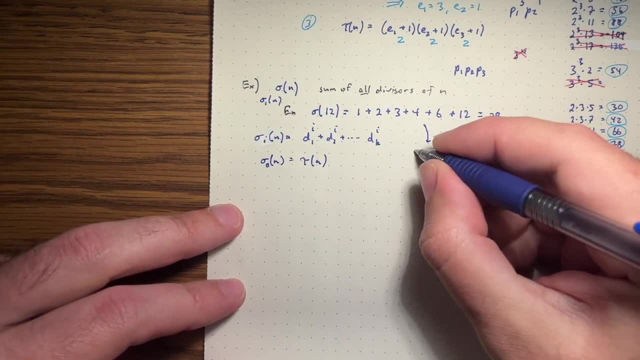 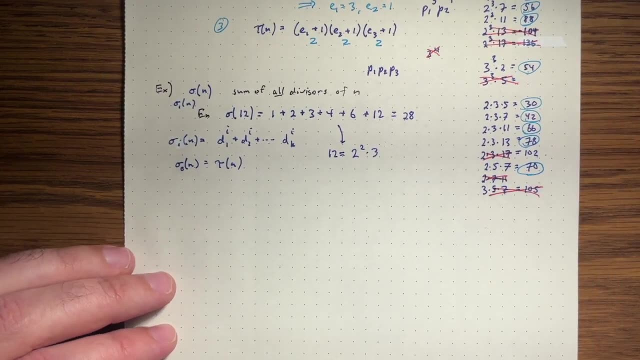 Okay. well, let's look at 12 again. So 12 is its prime. factorization looks like this: 2 squared times 3.. And we can see all the divisors from here. We can pick a 2 to the 0,, 2 to the 1,, 2 to the 2.. 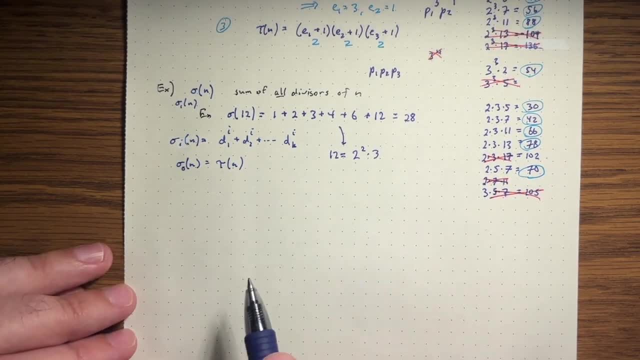 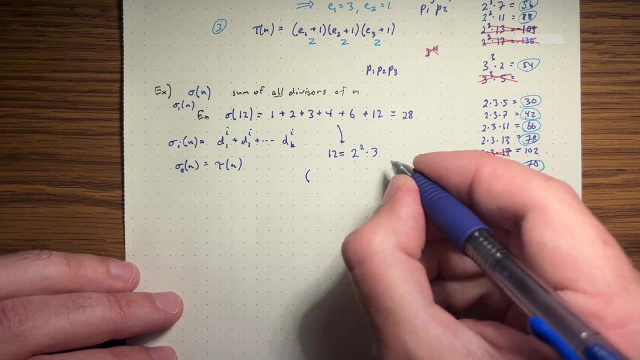 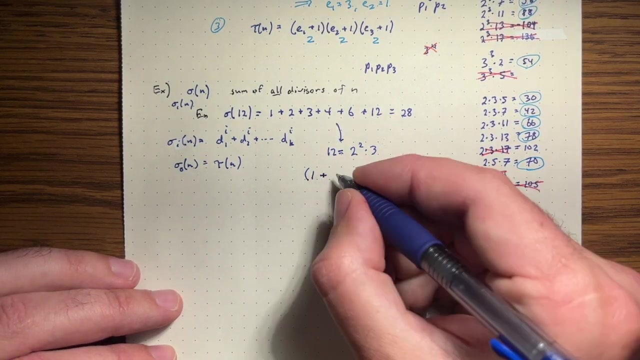 We can pick a 3 to the 0 or 3 to the 1.. Those all give us divisors. I know a nifty way that I can actually get all those terms, So all the divisors, in a sum, And the way to do that is. so I'm going to take 1.. 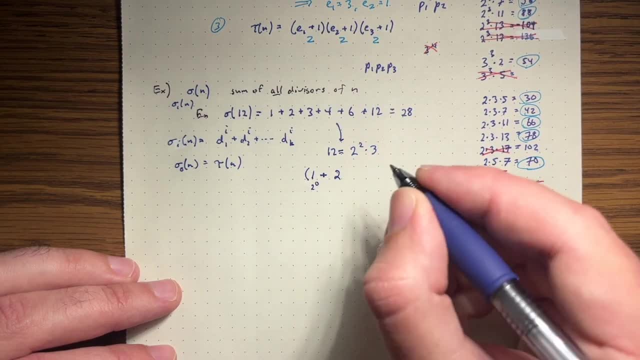 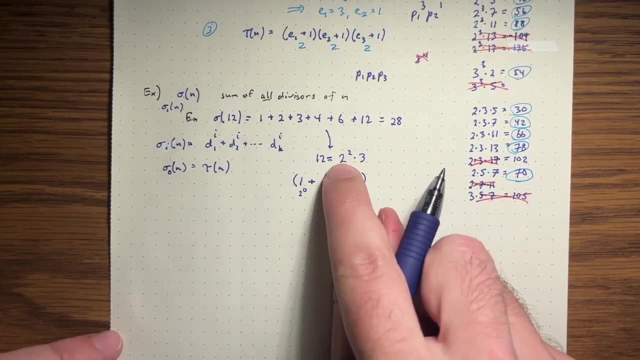 I'm going to take which is like 2 to the 0.. I'm going to take 2 to the 1,, 2 to the 2.. If I just have that sum alone, this would be the sum of the divisors of 2 squared. 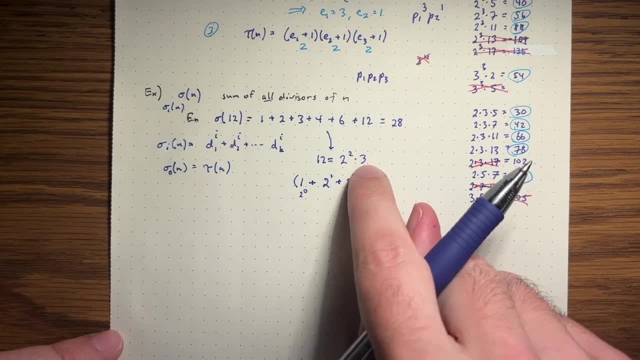 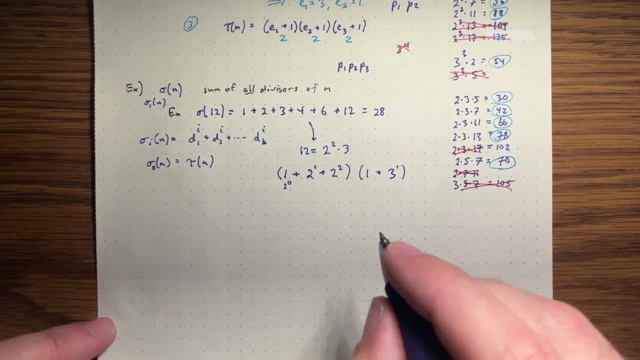 But I'm also allowed to take Divisors of 3. Divisors of 3 look like 1 and 3. So 1 plus 3. 3 to the 1, if you like. Look what happens if I multiply these together. 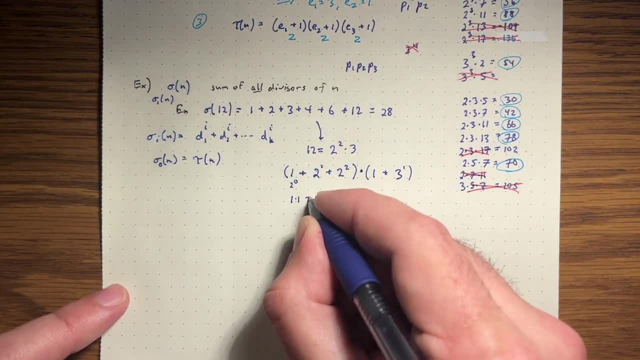 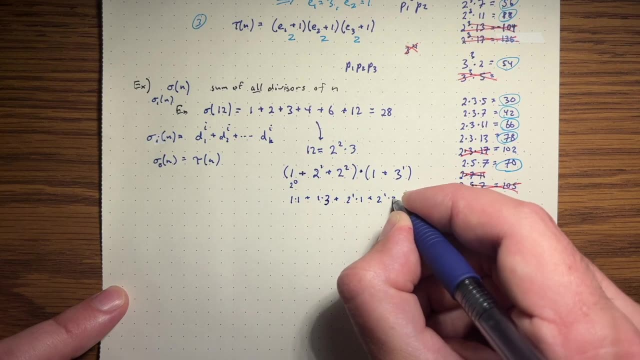 I get 1 times 1.. 1 times 3.. Plus 2 to the 1 times 1.. Plus 2 to the 1 times 3.. It's sort of generating all possible combinations of these and adding them up. 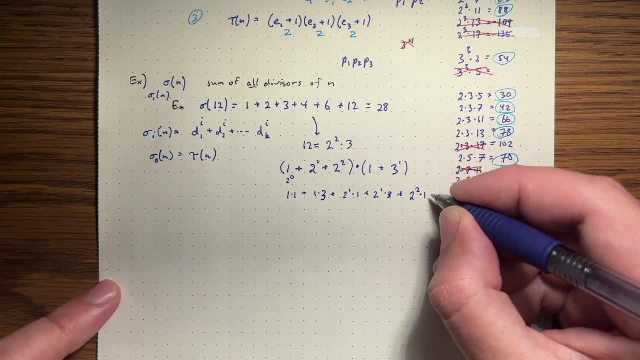 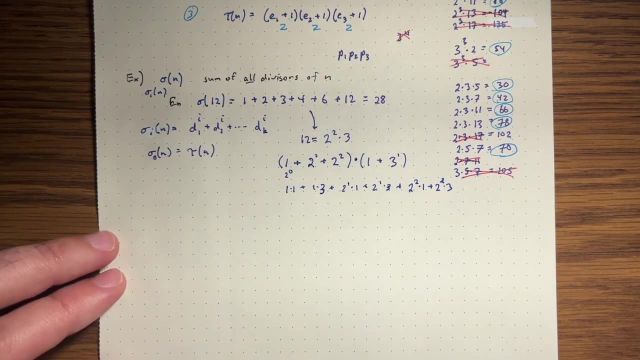 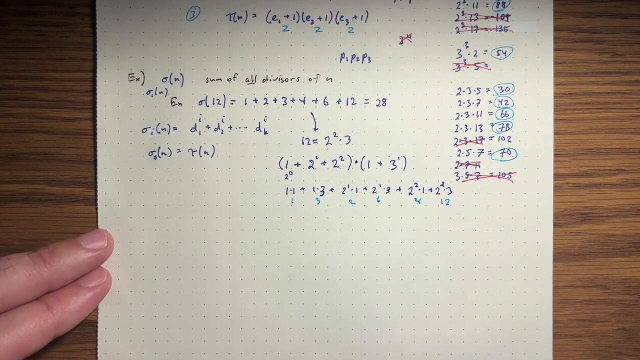 So this is exactly what I want to do: 2 squared times 3.. These are exactly all the divisors of 12.. So what is this? 1,, 3,, 2,, 6,, 4,, 12.. 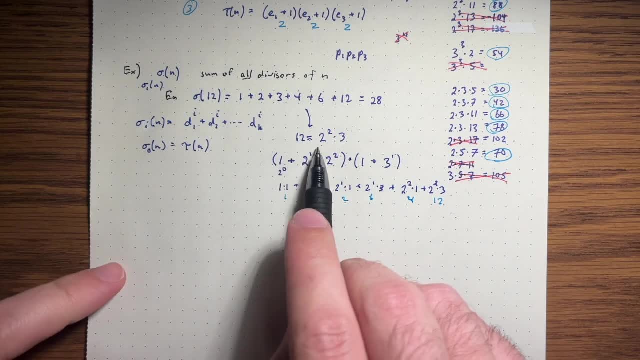 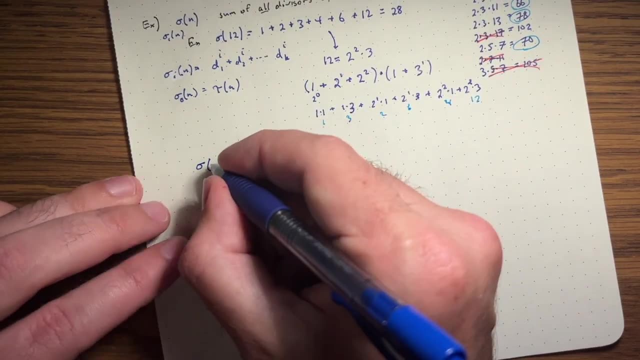 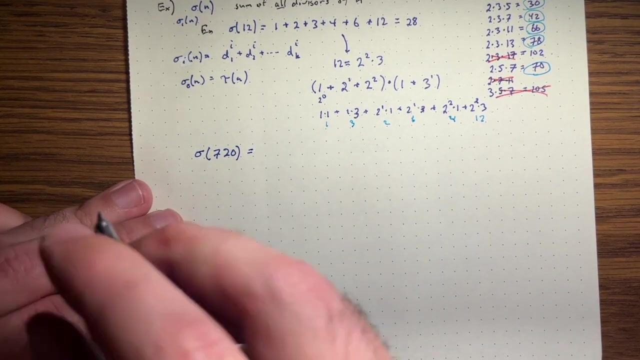 And so this is what you can do in general, essentially. So you write your numbers of prime factorization. Let's do another example, just to show before I write down a general formula. So let's do sigma of 720.. What did we decide? that 720 was? 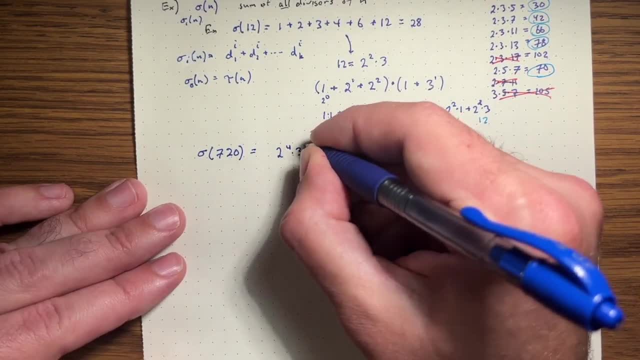 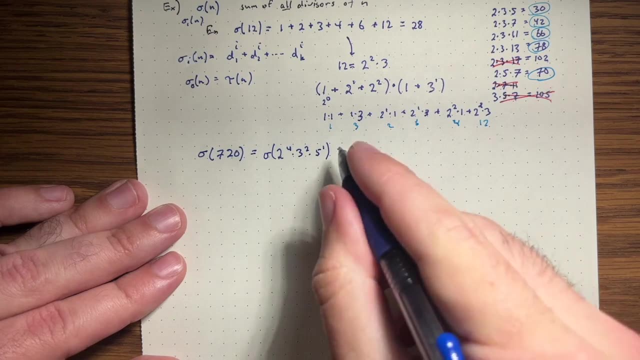 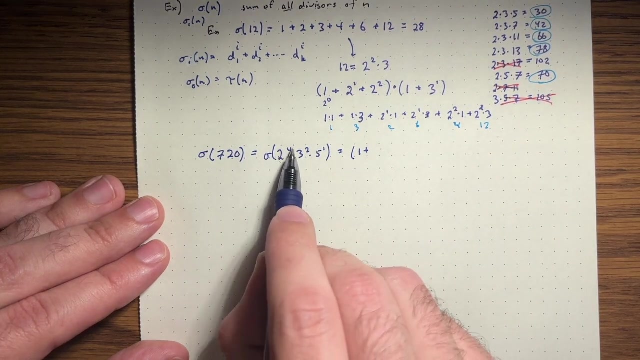 So 720 was 2 to the 4 times 3, squared times 5 to the 1.. Okay, We're going to use our trick again. So our trick is: you write out all the possible divisors you can take from here. 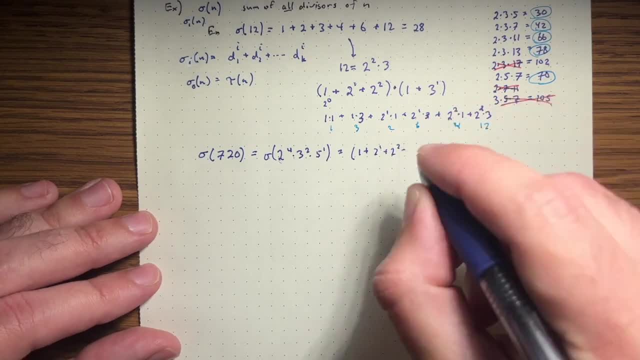 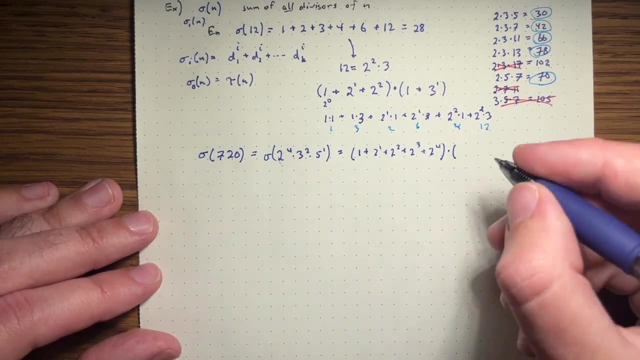 From the 2.. So you do 2 to the 1,, 2 to the 2.. I'm writing them as a sum: 2 to the 3.. 2 to the 4.. I'm going to multiply that by the sum of all the divisors from the 3.. 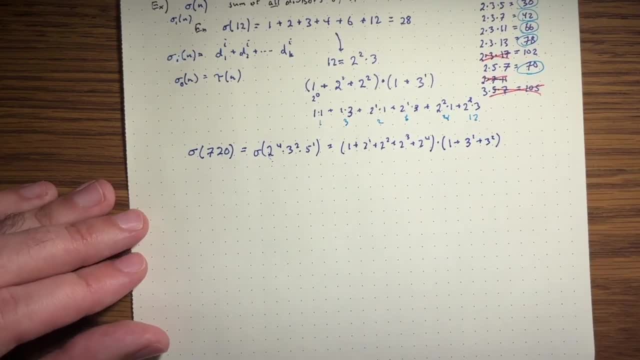 So I can do 3 to the 1,, 3 to the 2.. And you see why I'm doing this is because when you multiply these out, you're going to get 5 terms there, 3 terms there, I'm going to get 15 terms. 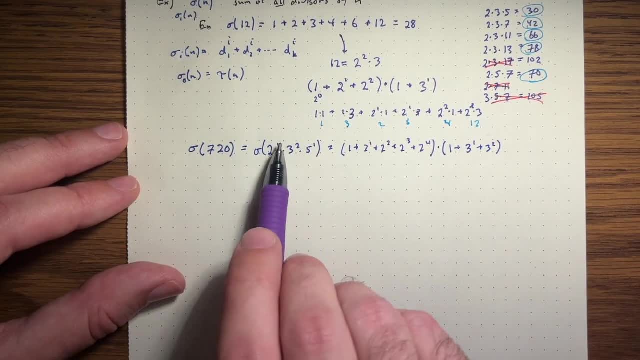 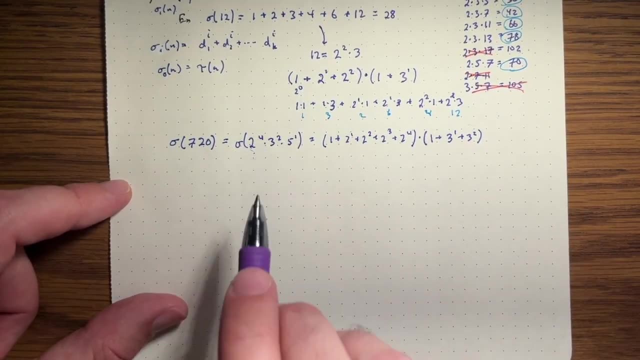 Each one of them is going to sort of choose a combination of these exponents. So I will just get a sum over all the divisors of these first two, And then I can multiply this by 1 plus 5 to the 1.. 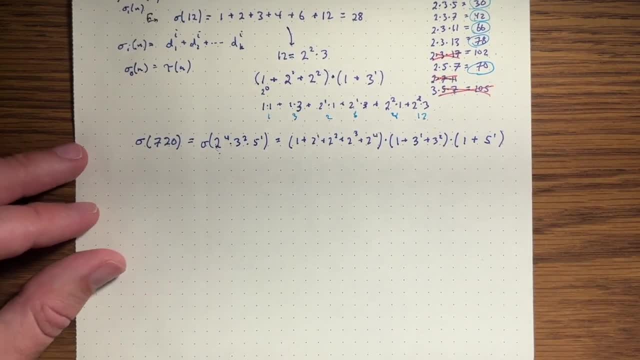 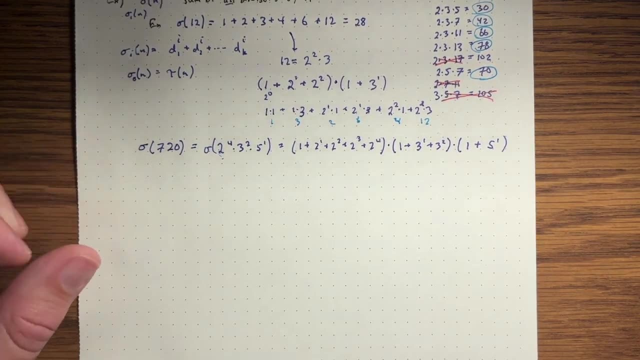 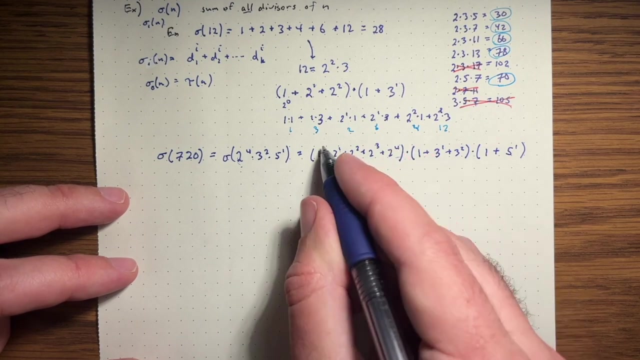 That's all I'm allowed to take for the 5.. And so this product, whatever it is, is the sum of all the divisors of 720.. Now I mean, we can figure this out. So what is this? This is a geometric series, actually. 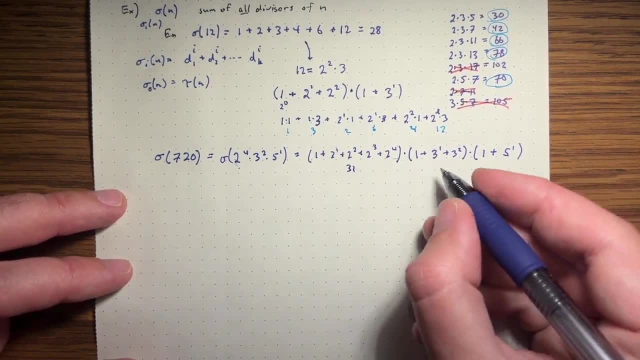 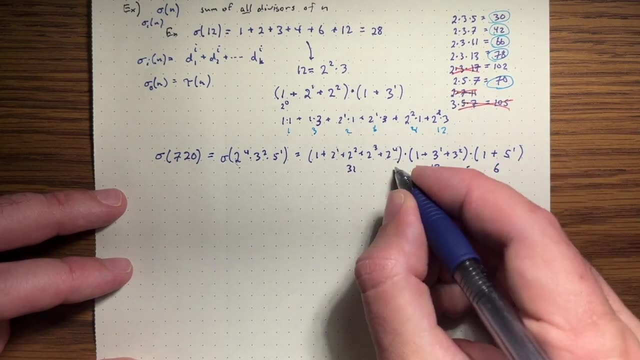 So this should be: 2 to the 5 minus 1 is 31.. This term here is 1 plus 3 plus 9 is 13.. This term here is 6.. So it's 31 times 13 times 6, whatever that is. 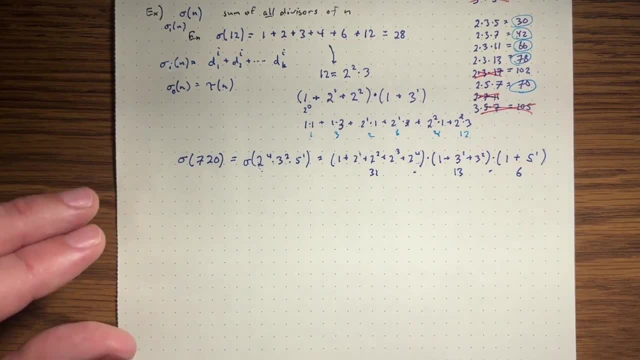 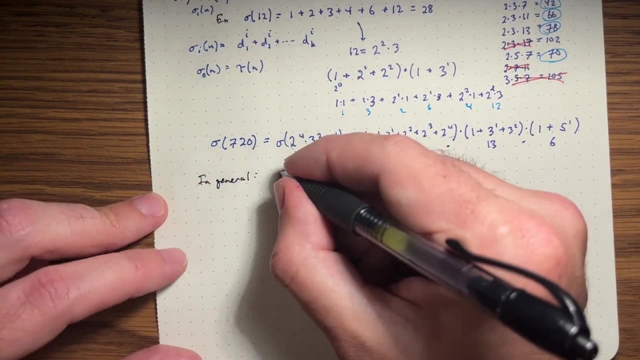 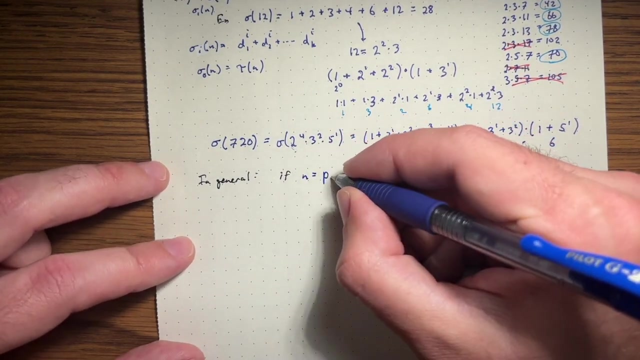 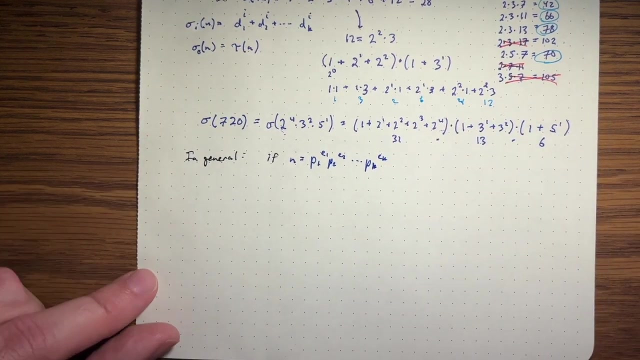 That's the sum of all the divisors of 720.. So in general, it turns out we're going to have a formula for this just like we did for tau. So if n equals p1 e to the 1, p2 e to the 2,, et cetera, pk e to the k. 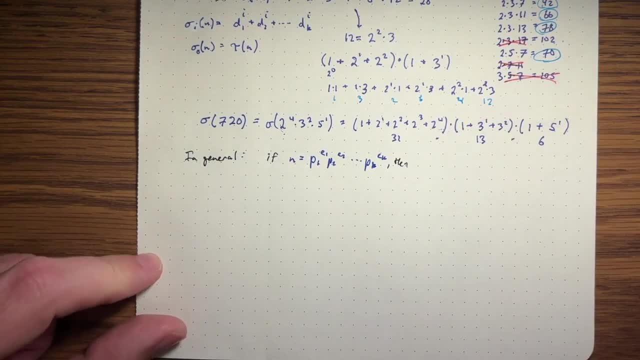 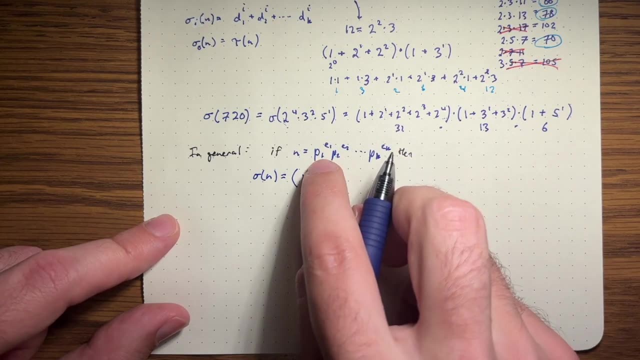 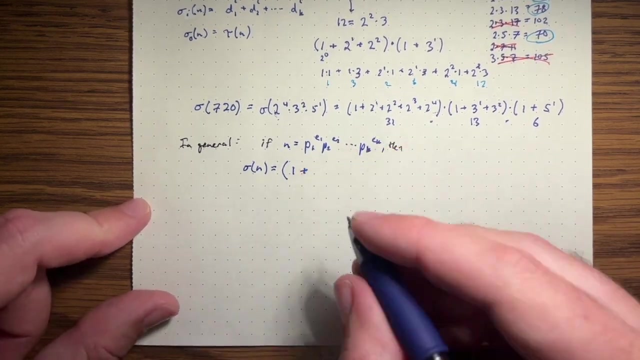 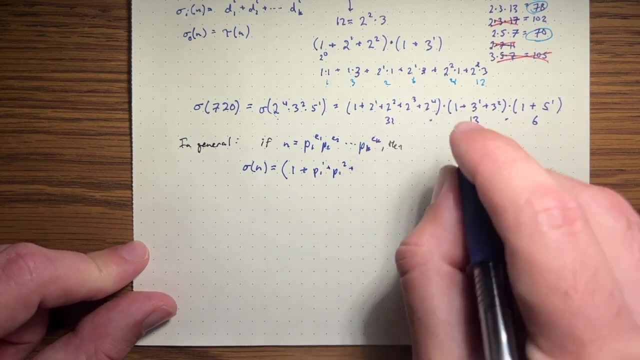 then sigma of n is, we'll do 1.. So we're choosing all the divisors of this p1.. And then for each of these choices we can multiply by all the divisors of everything else. So 1 plus p1 to the 1 plus p1 to the 2 plus. I'm just kind of copying this here: dot dot, dot. 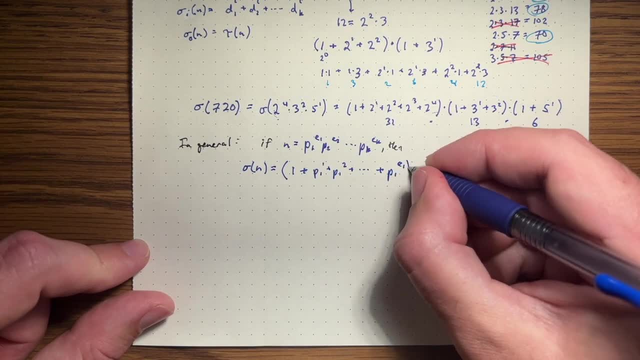 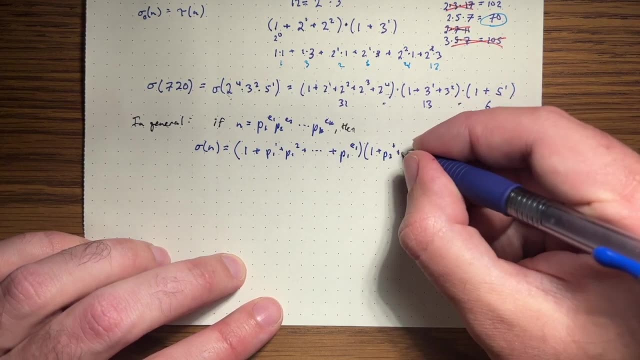 plus p1 to the e1. So we go all the way up to whatever that exponent is. We do the same for the next one: p2 to the 1 plus p2 to the 2, all the way up to p2 to the e2.. 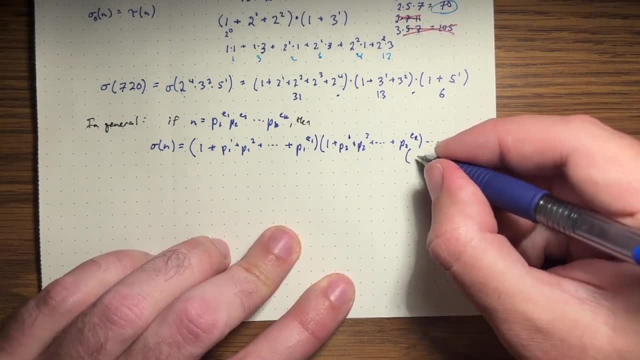 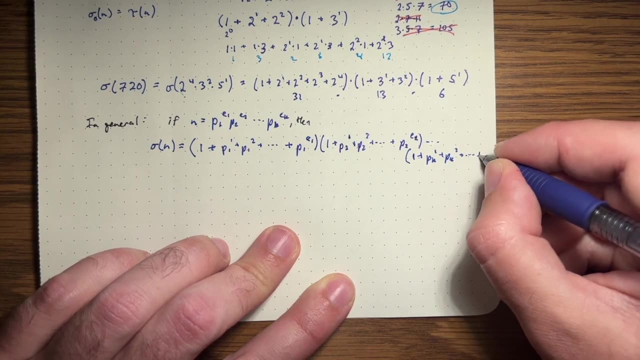 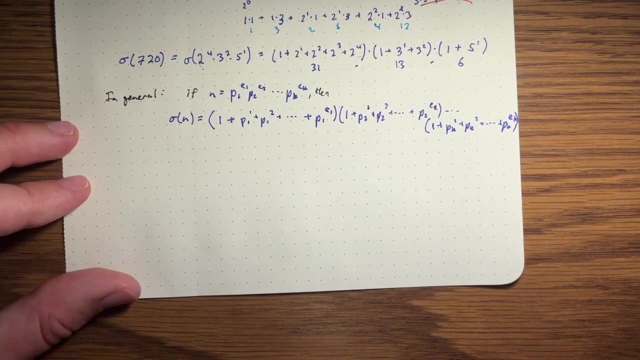 And you keep going until we get to this last bit. So pk to the 1 plus pk to the 2, plus dot dot, dot plus pk to the ek. Okay, There's also another way you can write this. So these are geometric series. 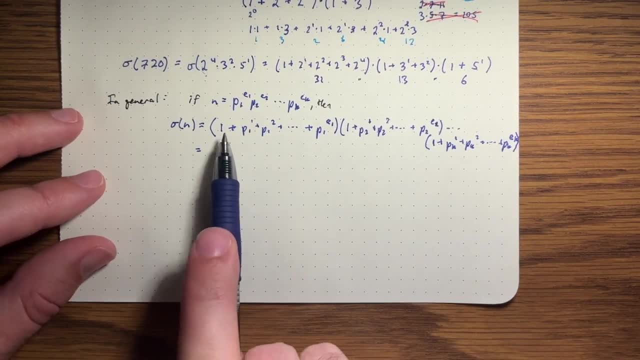 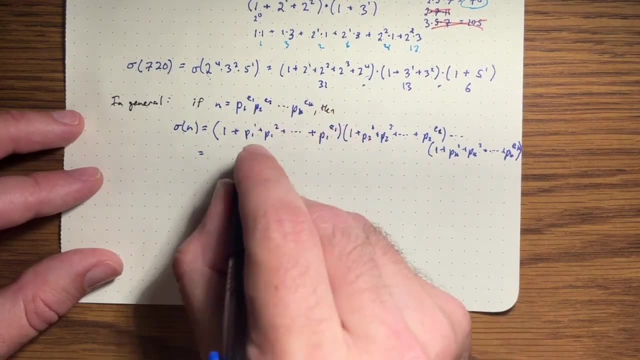 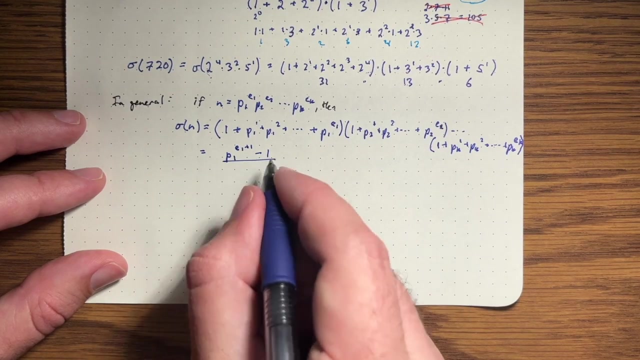 And you can recall maybe from an earlier lecture that we had to use a formula for this kind of thing. We're taking powers of a single number. So this sum here, this first bit, is going to be p1 to the e1 plus 1 minus 1, like that, over p1 minus 1.. 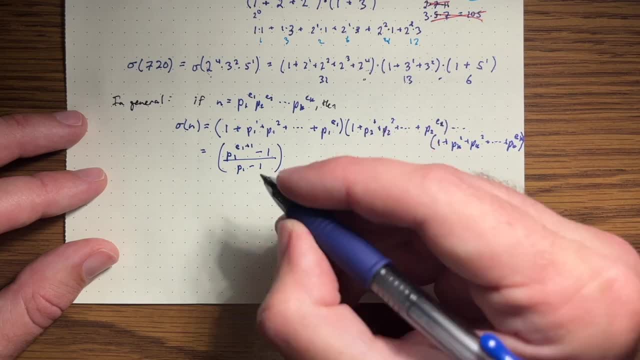 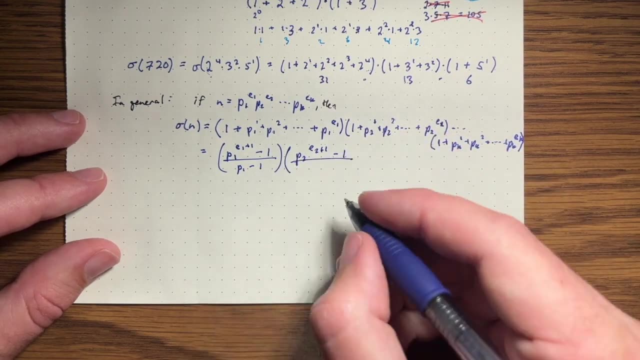 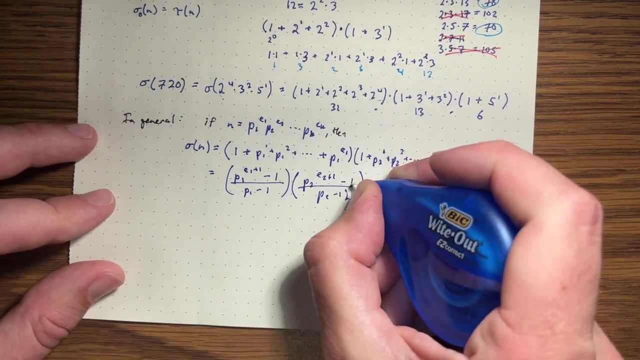 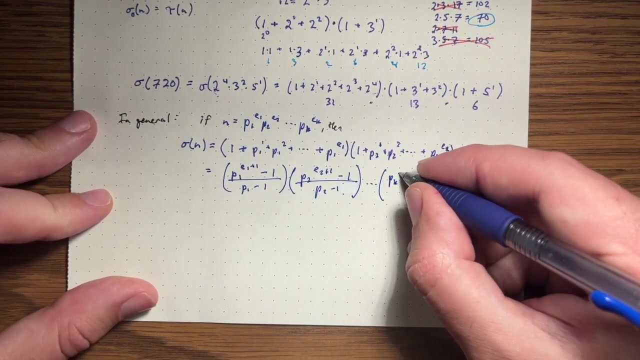 Okay, And that will be times p2 to the e2 plus 1 minus 1 over p2 minus 1.. And you keep going Go all the way up to pk to the ek plus 1 minus 1 over pk minus 1.. 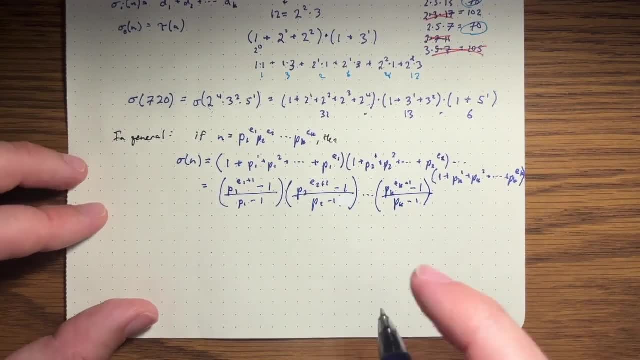 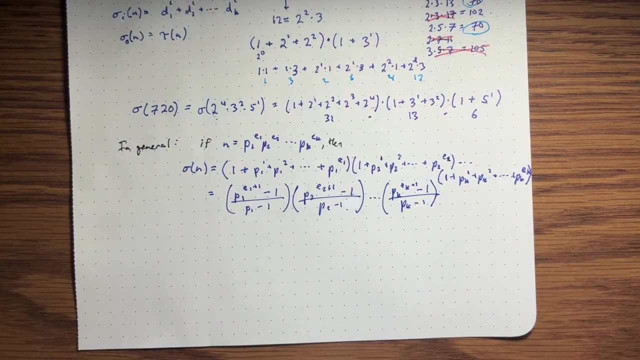 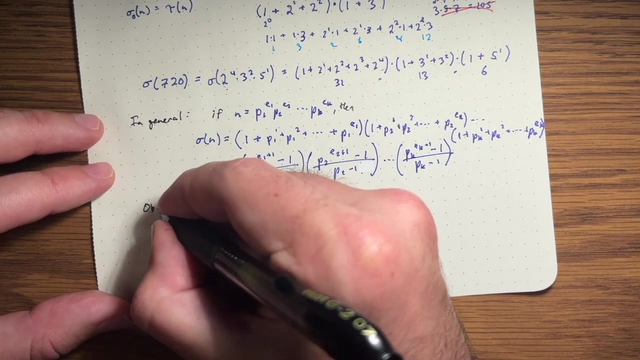 Okay, So I'm just using the formula for geometric series. Sometimes it's actually more useful to just think about it as these larger sums, But you can use either formula. And so another observation. So observe that this sigma of n is multiplicative. 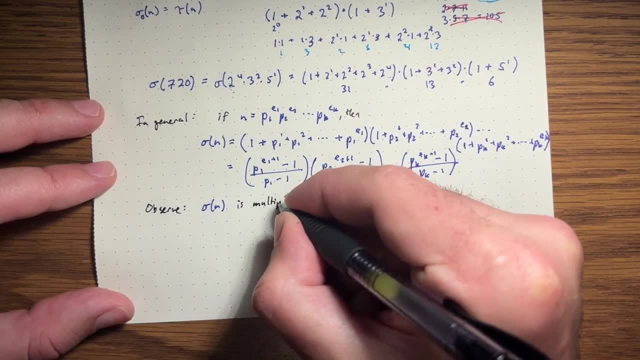 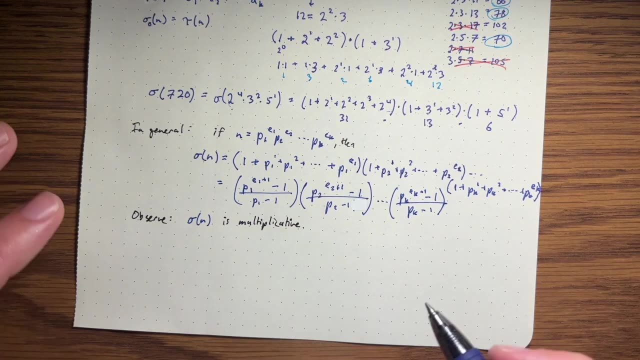 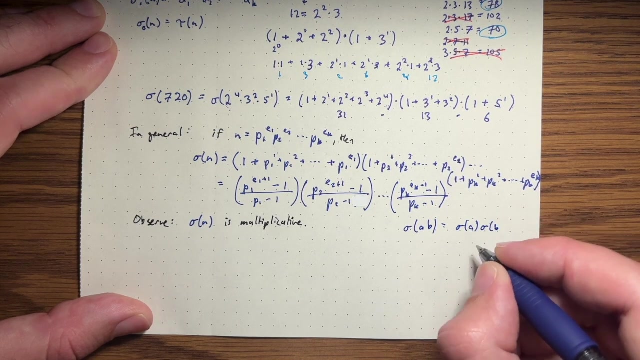 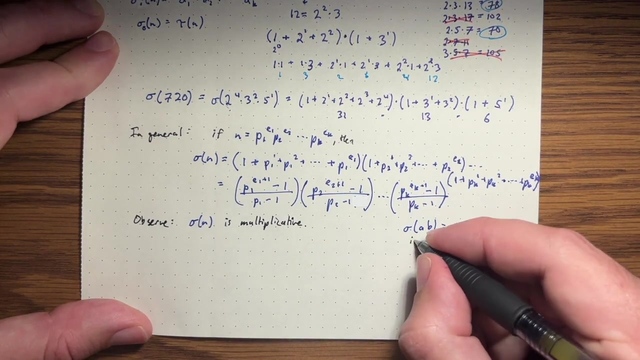 What does multiplicative mean again? So, multiplicative, It means that when you have a product ab, sigma of ab is equal to sigma of a times sigma of b, provided a and b are relatively prime. So this is if a and b are relatively prime. 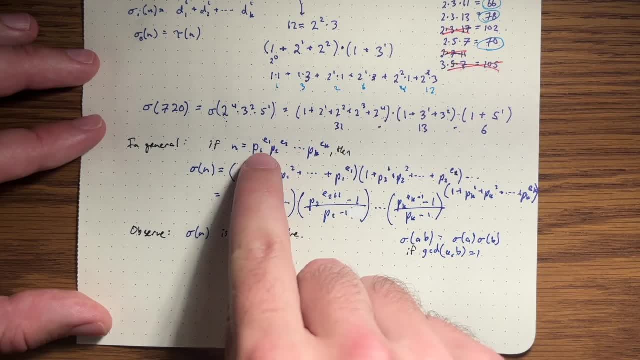 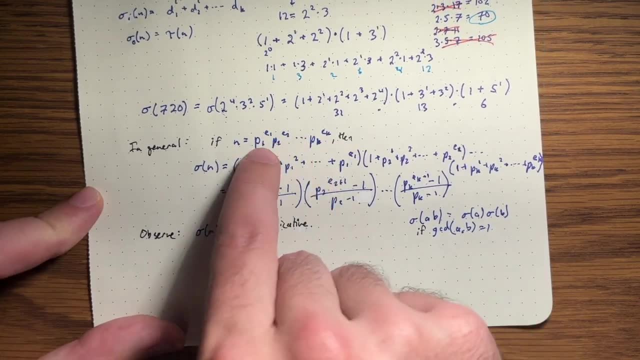 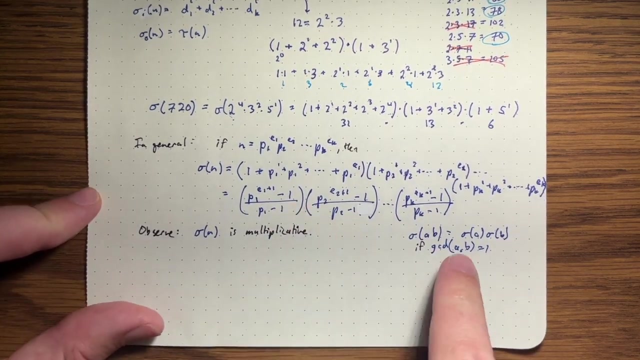 But essentially that's coming just from how we derived the formula, Because it's a product over these different primes. So if you have a relatively prime product equaling n, you're sort of splitting this formula into two parts And then ultimately multiplying them together, which is what we're doing here in the formula anyway. 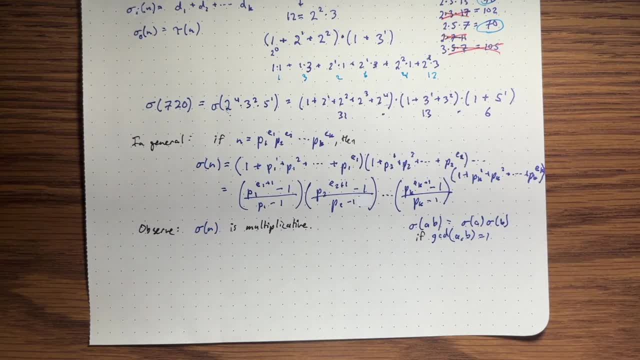 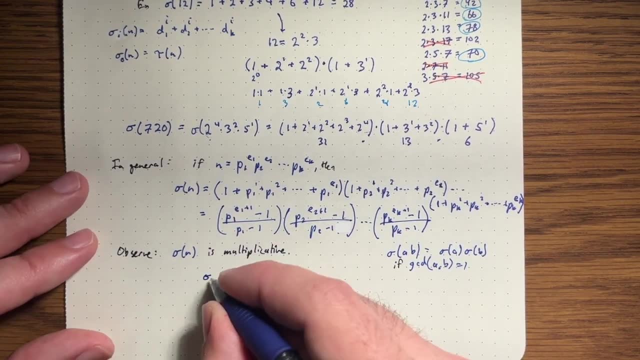 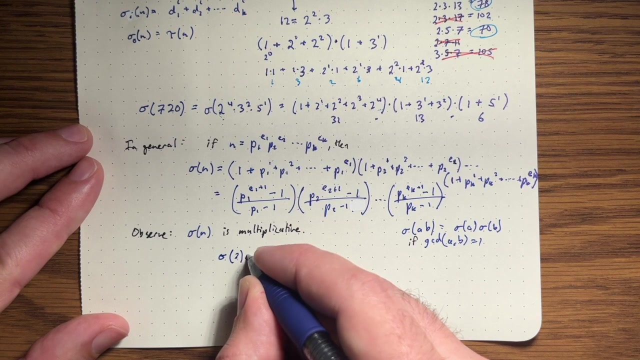 So this is a multiplicative function. Is it completely multiplicative? So is it completely multiplicative? It's multiplicative, but it turns out it's not completely multiplicative. So essentially, you can just find that with a small example. So let's take two things that are not relatively prime. 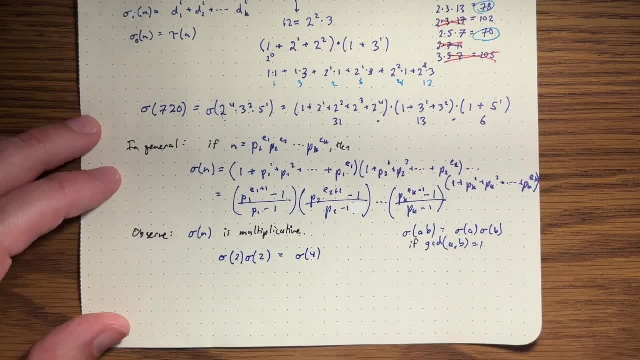 So 2 times 2 is 4.. Is it true that sigma of 4 is sigma of 2 times sigma of 2?? Well, sigma of 4, what is that? That's the sum of divisors of 4.. 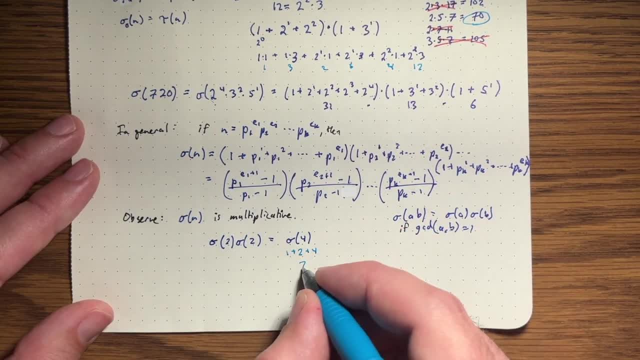 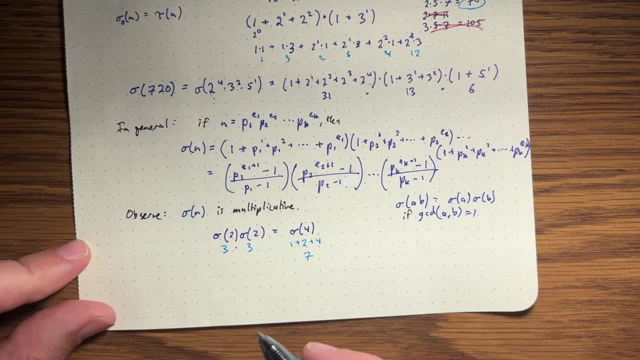 So that's 1 plus 2 plus 4, which is 7.. Sigma of 2 is 3, right, It's the sum of divisors of 2, which is 1 plus 2.. So 3 times 3.. 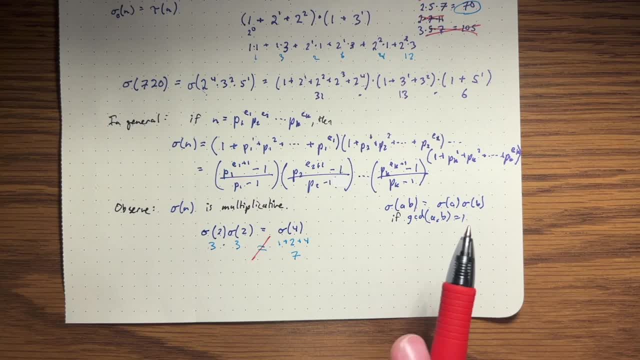 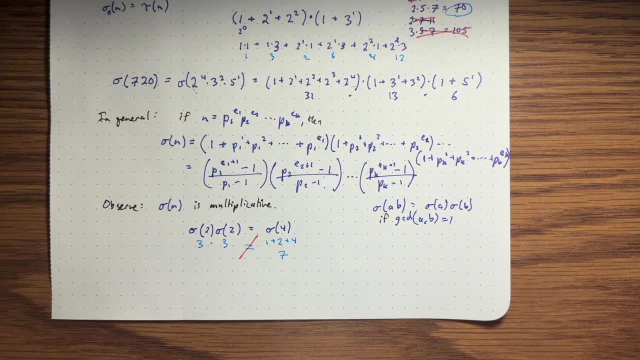 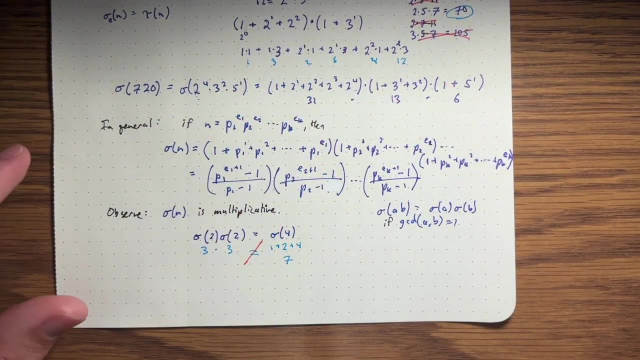 3 times 3, not equal to 7.. So, yeah, again, this formula only works if your two numbers here are relatively prime, Because we need to be able to get all the divisors from this kind of multiplication. That's why it works to partition it apart like this: 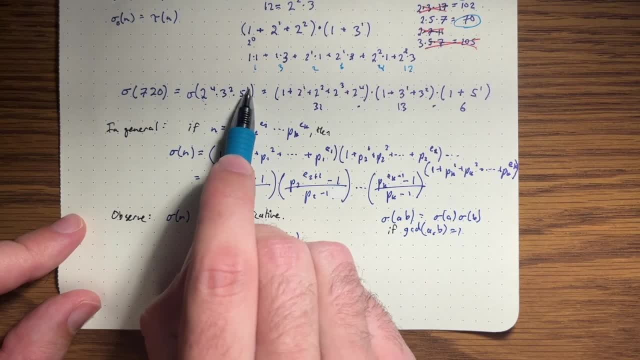 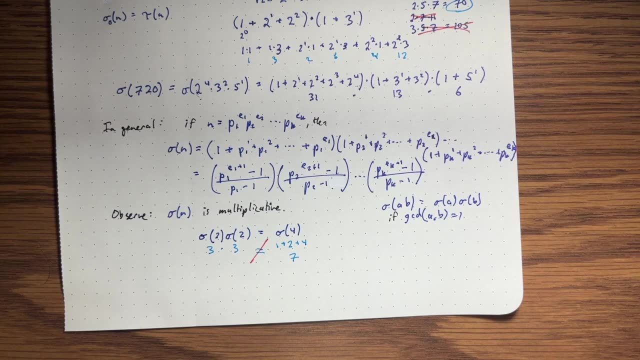 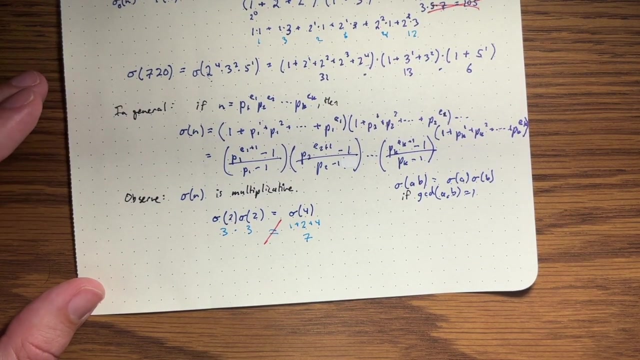 Because all the divisors of this number come from making choices of these separate exponents. Okay, great, So here's, by the way. so this is what we're going to be doing in the next lecture: We're going to be talking about perfect numbers. 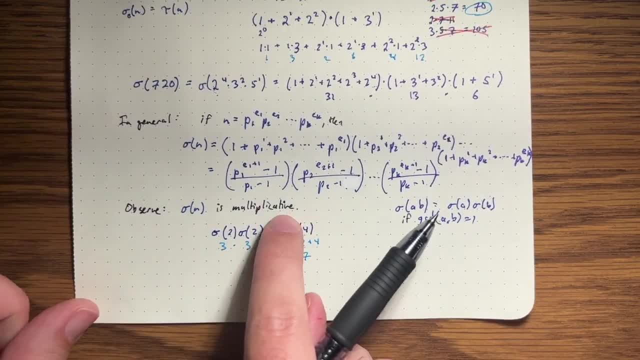 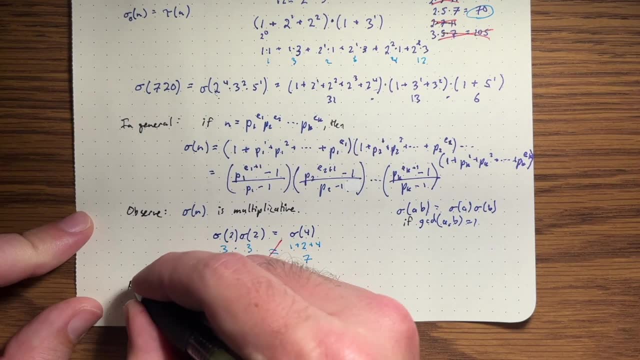 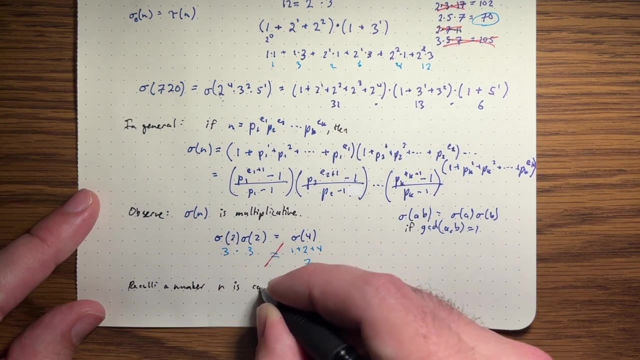 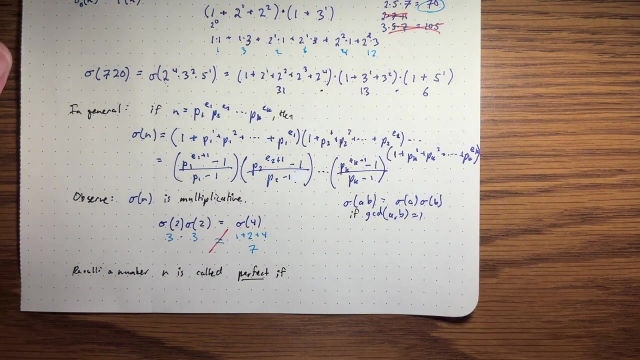 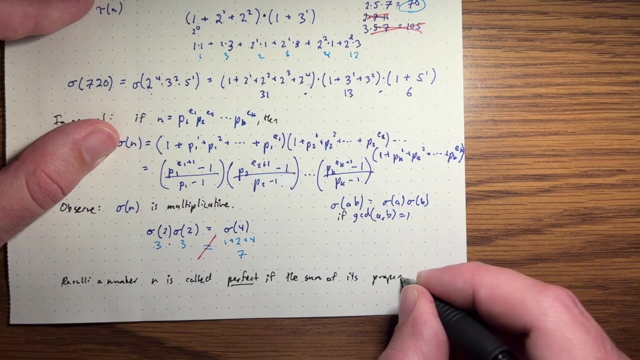 And essentially using this property, and basically this property alone, to classify all, even perfect numbers. But let's just recall, so, just to remind you. So a number n is called Perfect if the sum of its proper divisors, So if the sum of its proper divisors is n itself. 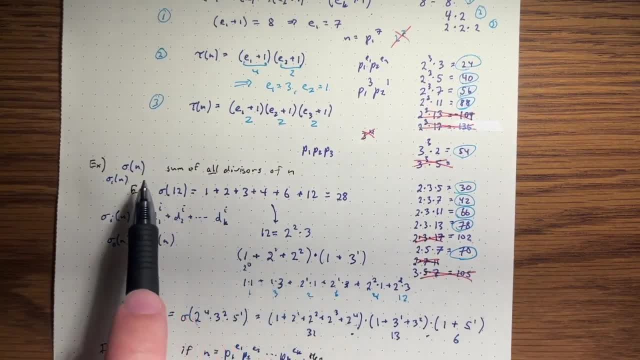 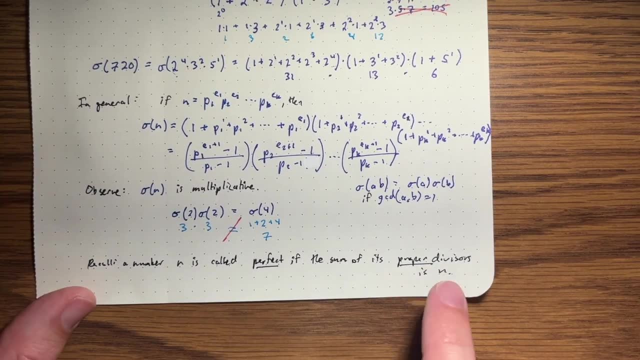 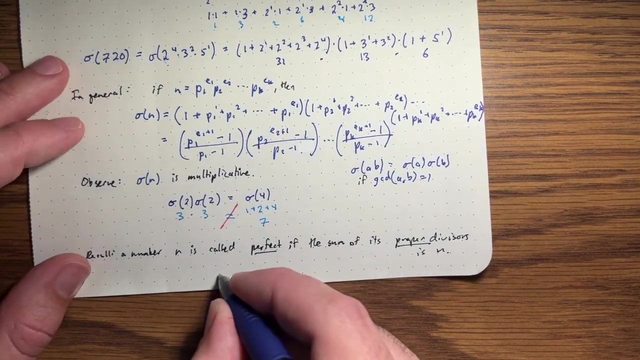 But this is proper divisors. Sigma is talking about all divisors, So It looks like we can't really write this concept in terms of sigma, But you really can, because So the sum of the proper divisors is n. Let's write the proper divisors. 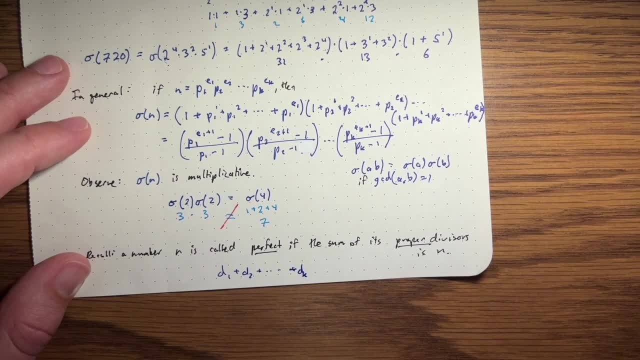 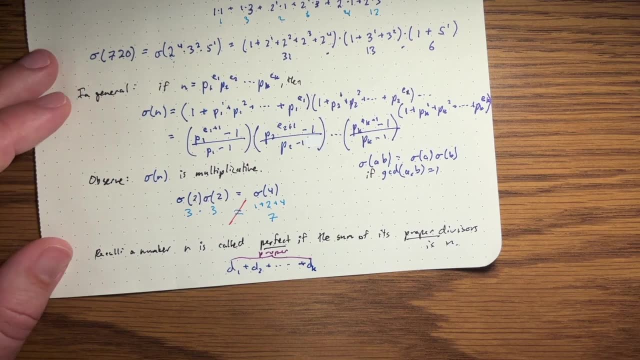 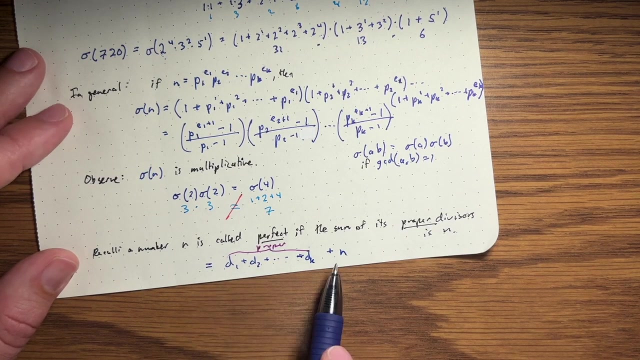 d2 up to whatever dk. So if these are the proper divisors Of n, Well, what are we missing out? We're just missing n itself. So if we add n itself, This is going to equal: Well, this bit here is already n. 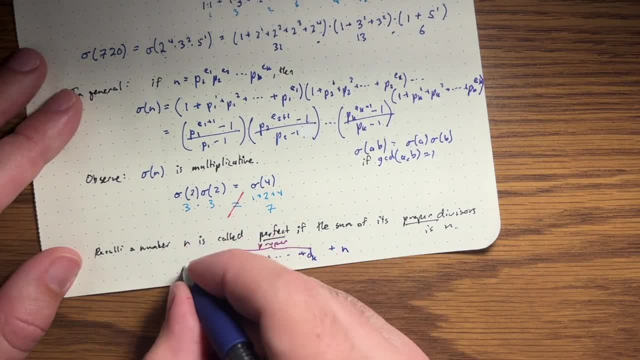 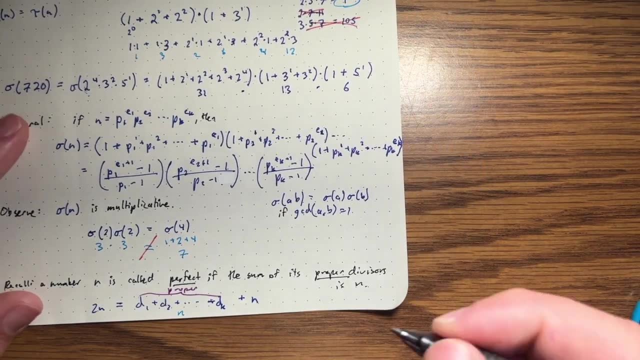 We add n itself, We get all the divisors. We get n plus n, That's 2n. So the sum of all the divisors Is 2n, for a perfect number. So in other words, There's just a. 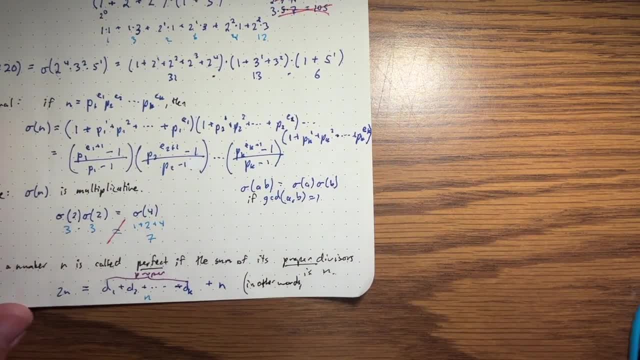 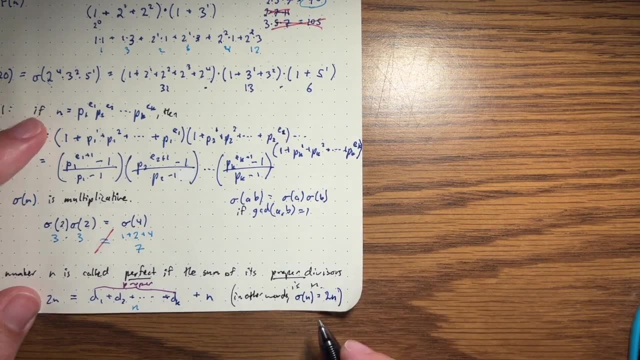 Rephrasing this in terms of our new function, sigma. So the number is called perfect if Sigma of n equals 2n- Not equals n, but equals 2n, Because we want the number itself When we're talking about sigma. 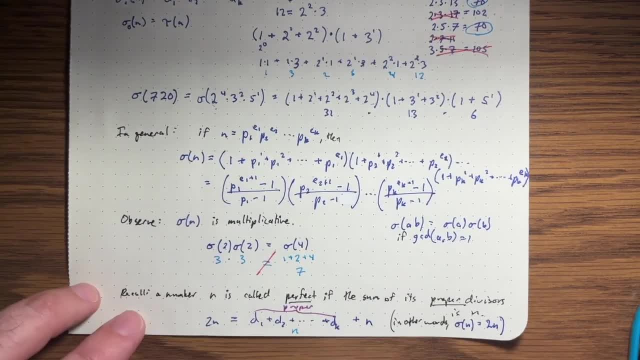 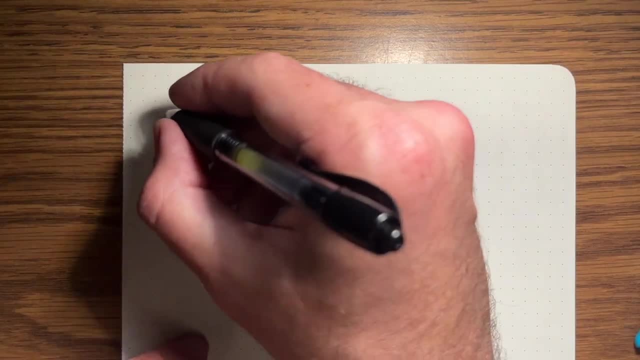 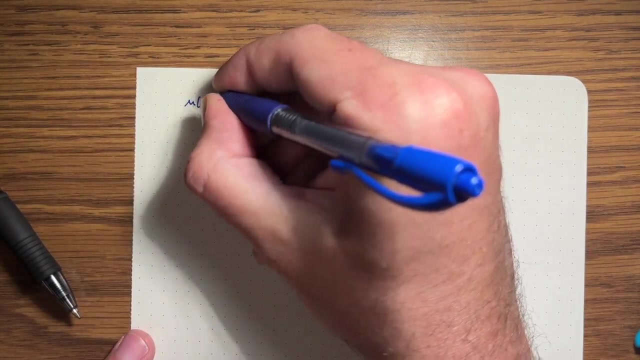 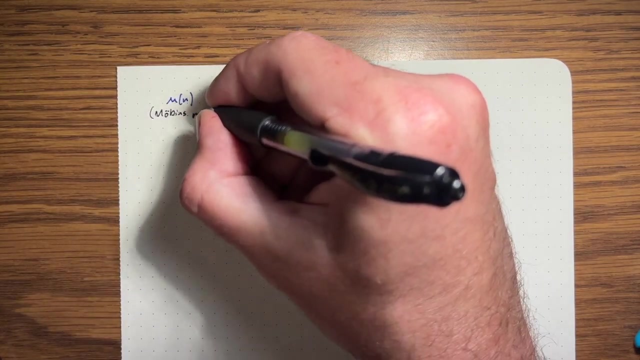 Because it becomes all divisors. Okay, so I'd quickly just like to introduce One final arithmetic function, And it's called the Mobius mu function. So this is Mu of n, This is the Mobius Mu function. 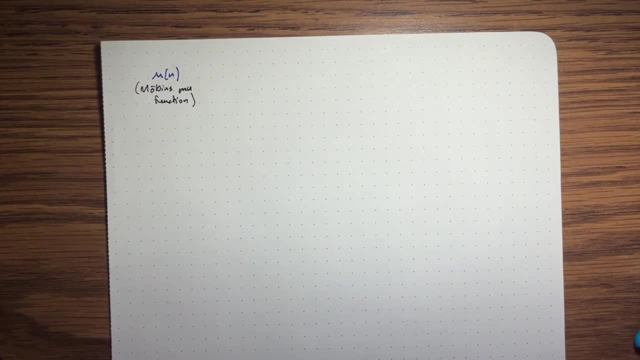 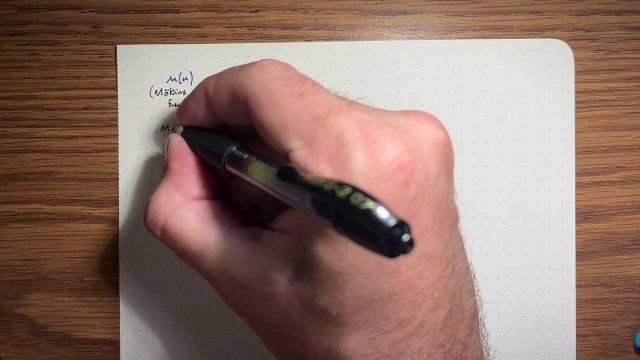 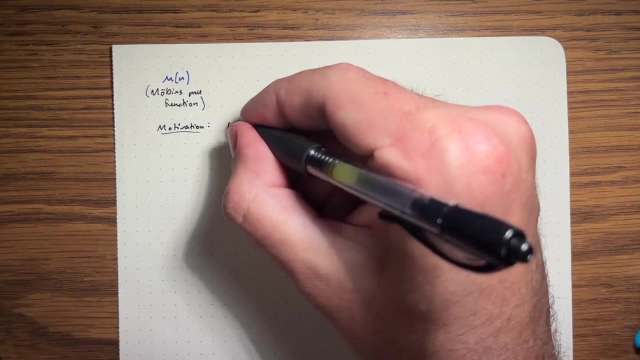 And It has a bit of a weird definition. So I'd actually like to motivate it first Before I define it. So motivation: There's one possible motivation for this function. Let's try to just count primes. So let's count. 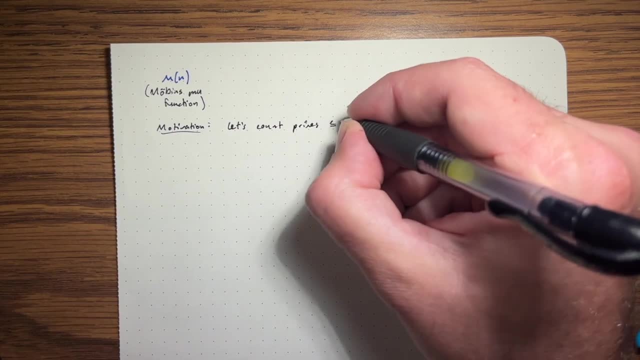 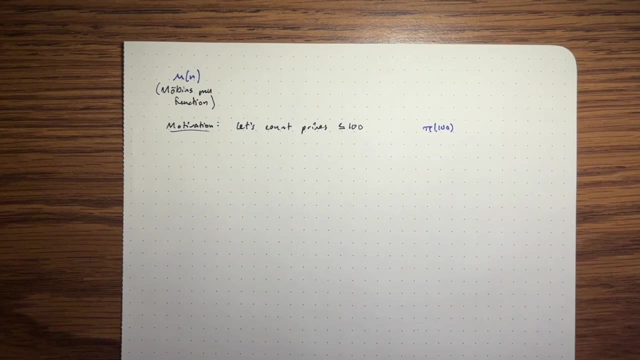 Primes Less than or equal to 100.. So, in other words, We want to find pi of 100.. Remember, pi is the prime counting function. We said earlier, it is equal to 25.. But what if we didn't know that? 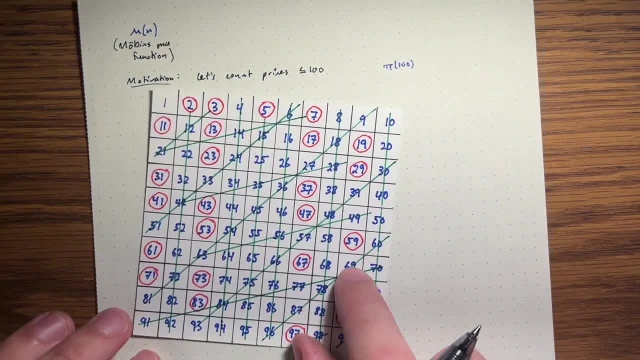 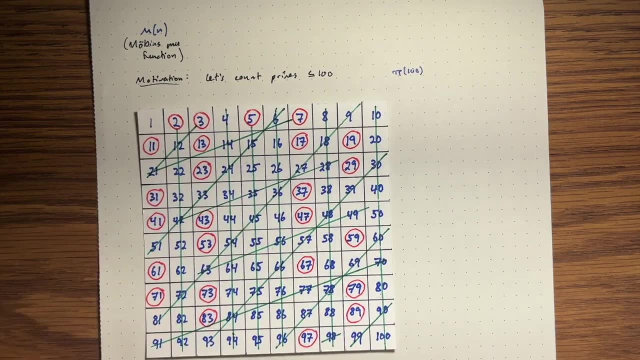 We want a strategy for counting primes. Let's go back to our Civ of Eratosthenes. Well, let's just try to write out the same idea that we did here. So What do we do in a Civ? We took all multiples of 2 and got rid of those. 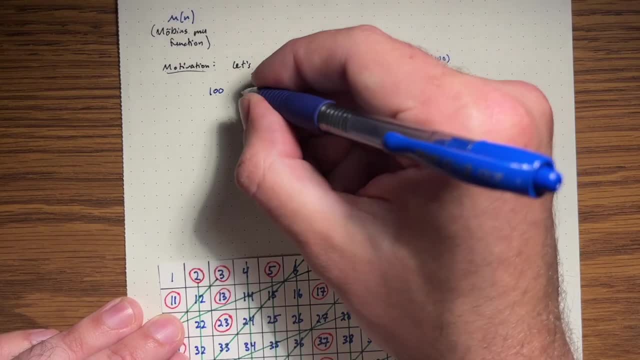 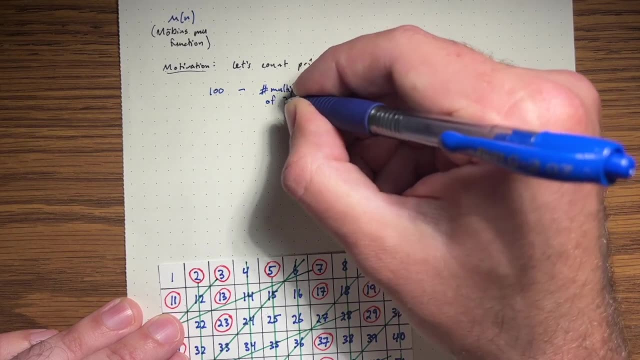 So let's say we're starting with 100 numbers And we're going to subtract off all the multiples of 2.. So how many multiples of 2 do we have Multiples of 2.. Okay, which I guess will be 100 over 2.. 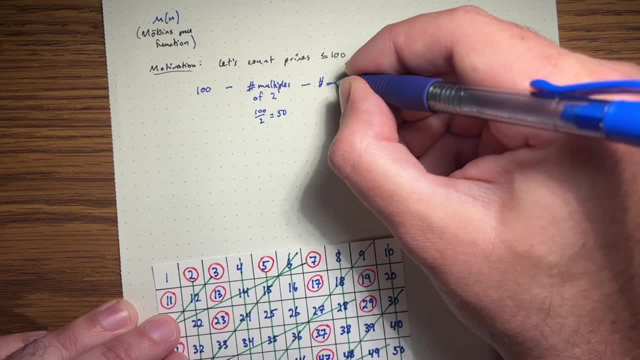 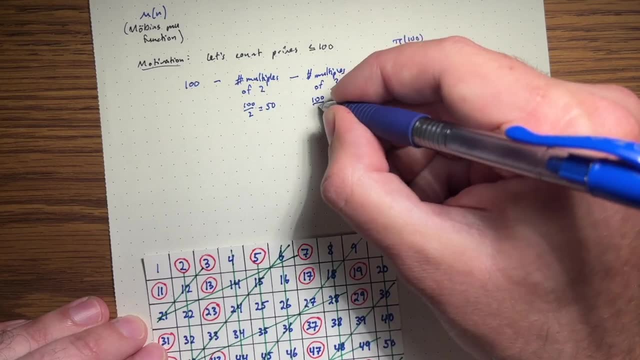 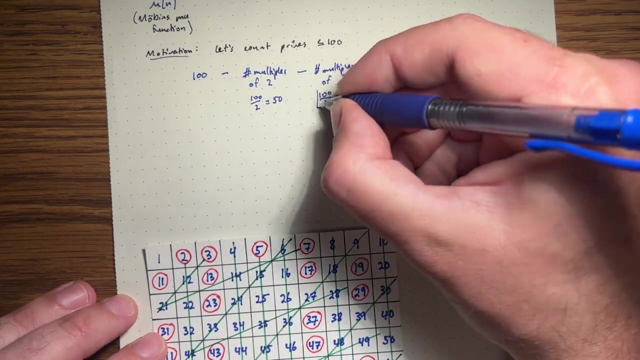 And then we subtract off the number of multiples of 3.. How many of those are there? I don't want to say 100 over 3, because that's not an integer, But The quotient is what you get when you divide 100 by 3, if you ignore the remainder. 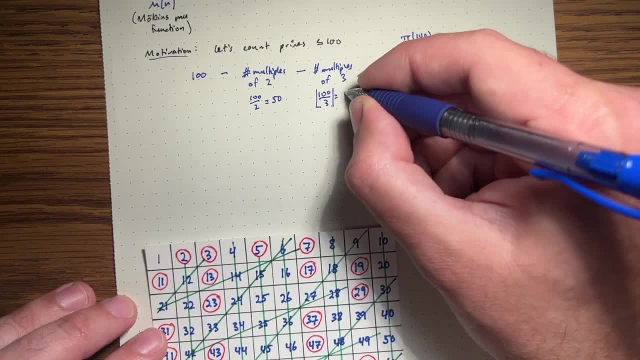 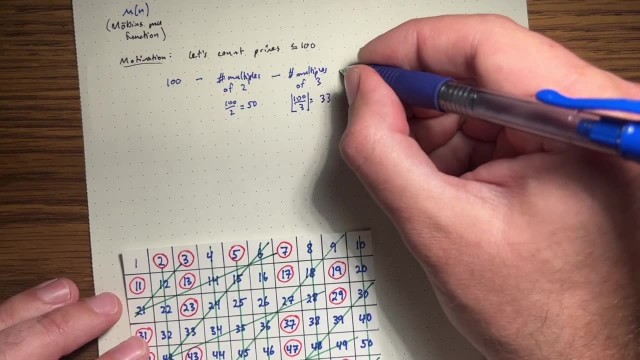 So I'm going to put this as a sign, Which means: take the floor of what you get. So it's 33.3. repeating, There are 33 multiples of 3.. We don't need to do anything with the multiples of 4.. 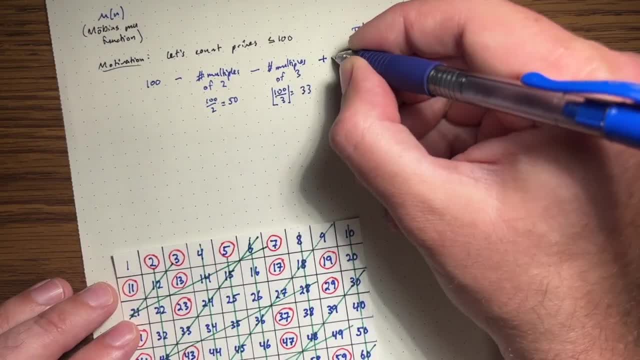 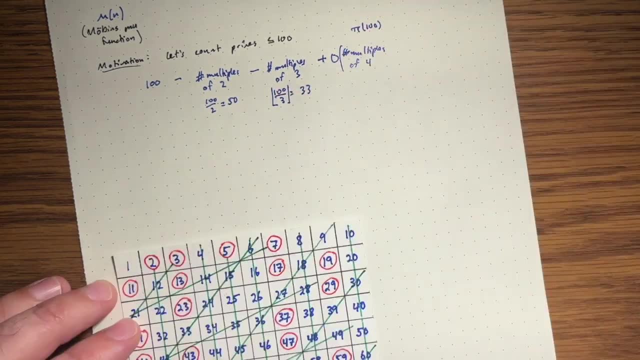 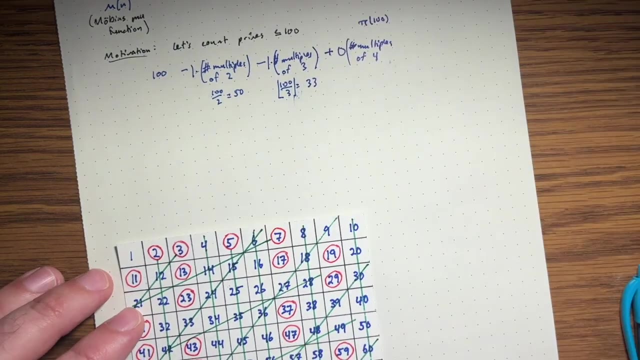 So I'm just going to write- I'm going to write- plus 0 times the number of multiples of 4.. I'm actually going to write this as minus 1 times, Writing this in kind of a funny way. Okay, what do we need to do next? 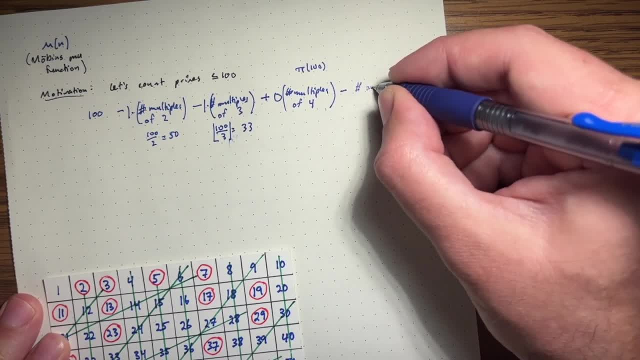 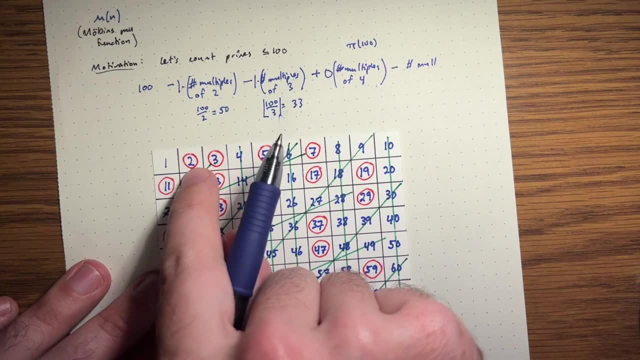 We need to subtract off the number of multiples of 5.. Let's just recall really quick: Why don't we need to cross out the multiples of 4? Those are sort of entirely subsumed by 2.. We already crossed out all the multiples of 2.. 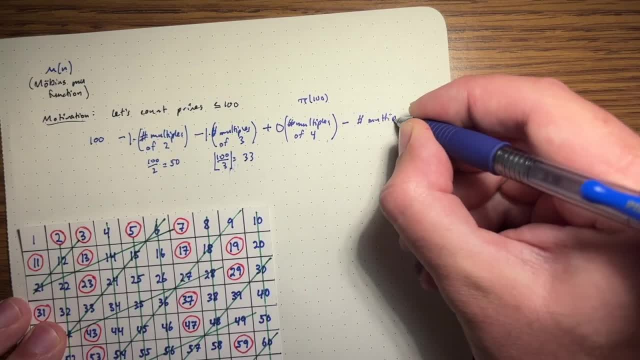 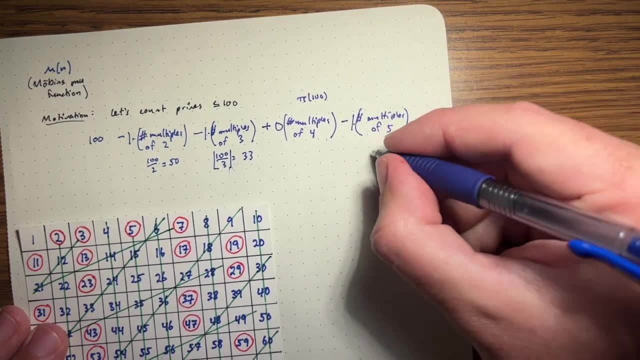 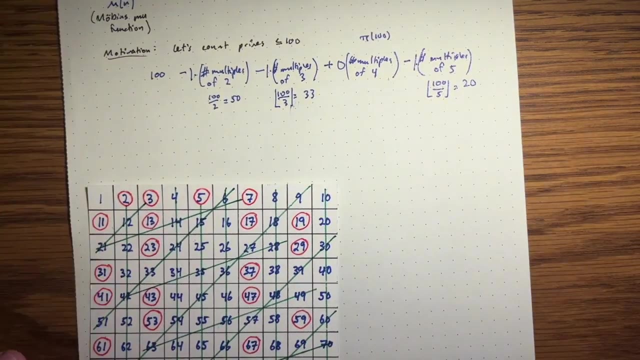 And 4 is just 2 squared. Let's cross out all the multiples of 5 next. So if we want to count, we need to do 100 over 5.. I don't need a floor function there, I'm just putting it just to be safe. 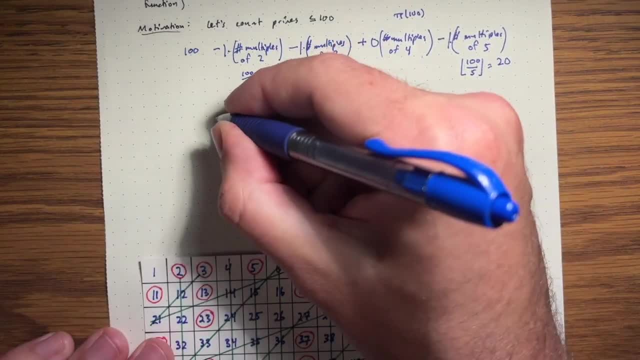 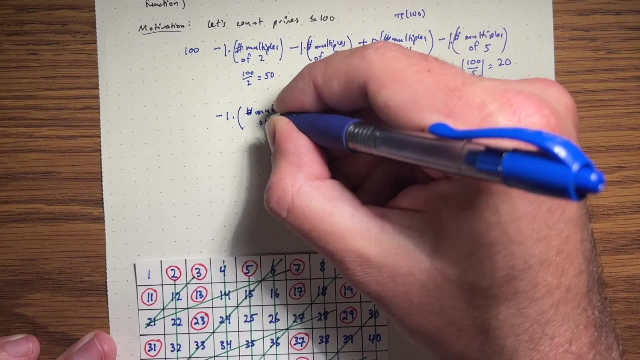 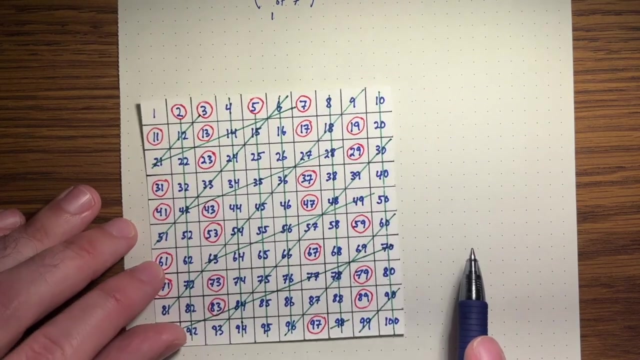 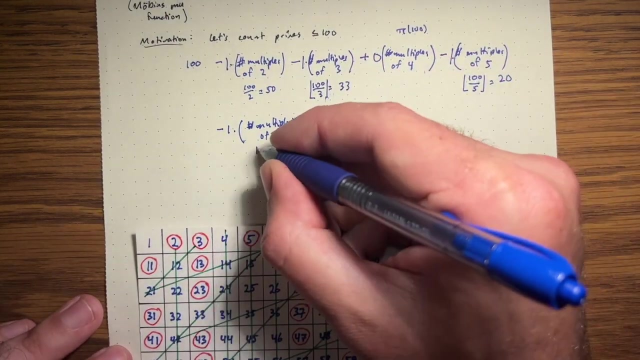 Okay, And we also need to subtract out the multiples of 7.. Whatever, that is Etc And actually after that we're done, Because we only need to check primes up to the square root of 100.. So if something is divisible by 11, it would be 11 times something that we already checked. 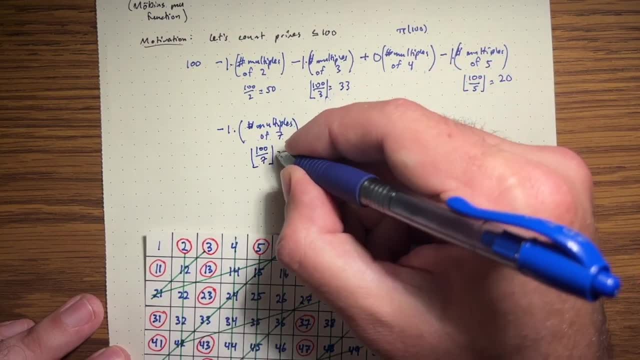 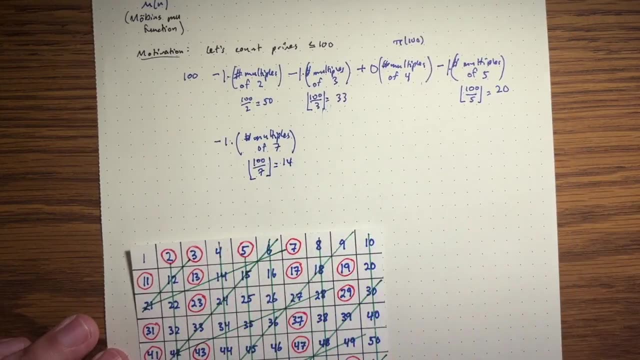 However, this gives you the wrong answer. if you calculate it, What is this, by the way? 14?? This will give you the wrong answer. See, if we subtract these out, these already are adding up to something bigger than 100.. 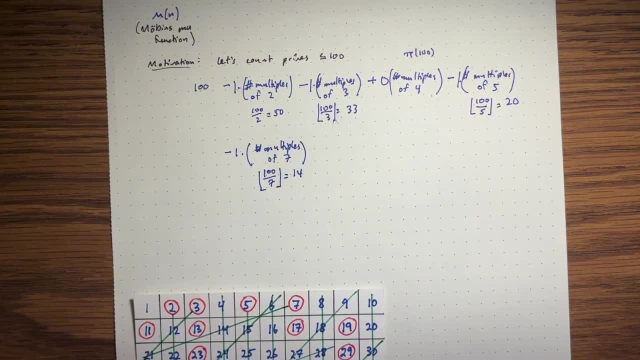 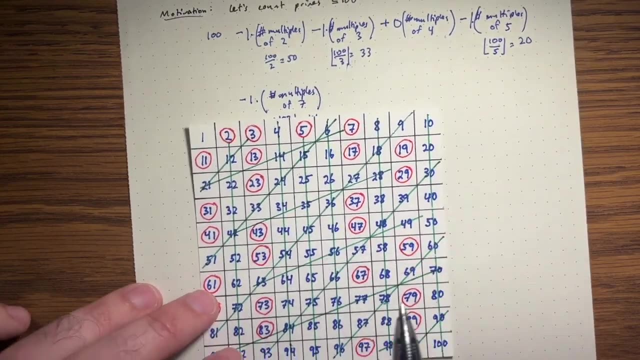 So we're going to get a negative number, which doesn't make any sense. So the problem here is actually In our picture. it was fine, actually, Because we just cared about the primes, But when we're counting them with an equation like this, 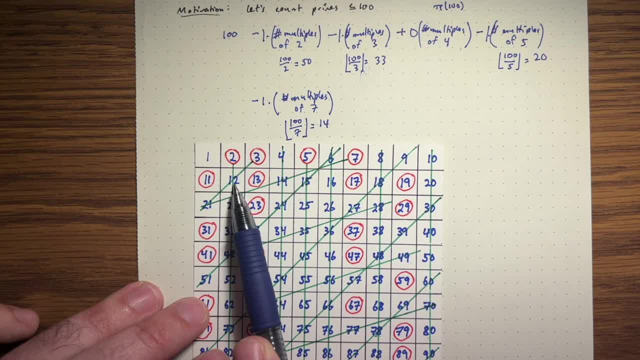 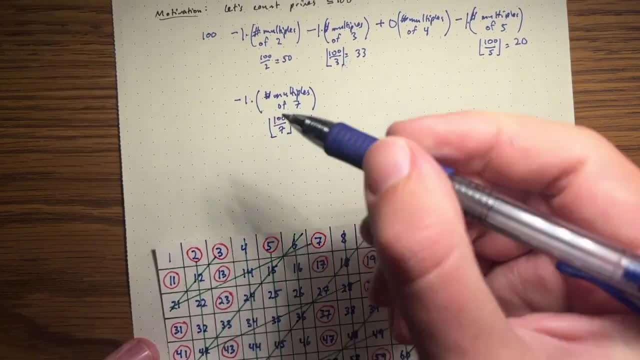 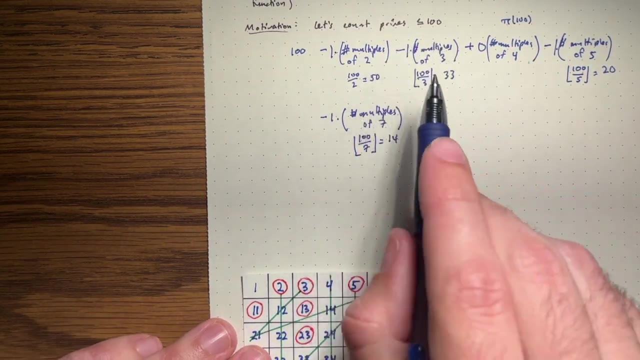 we have to take into account that some numbers we actually crossed out more than once, Like this 12 here, this 6 here, In fact any multiple of 6.. See 6 is 2 times 3.. So We crossed all multiples of 6 out twice. 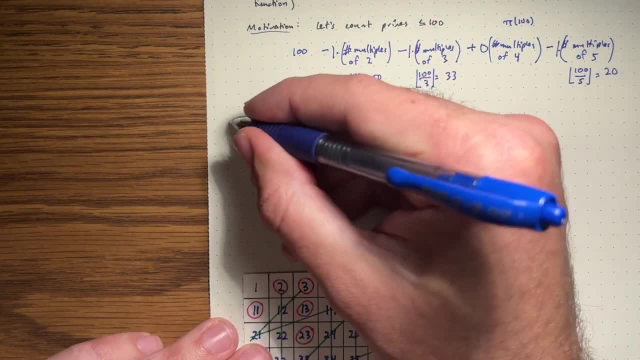 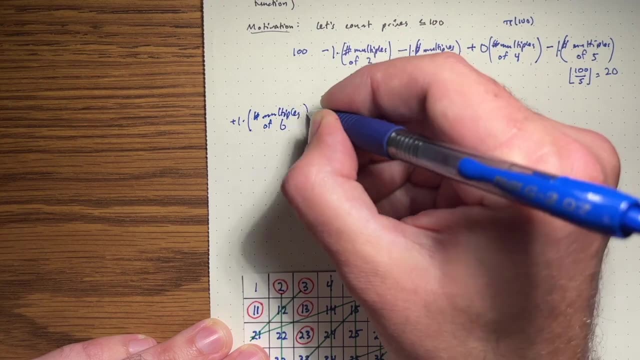 We didn't want to do that, So why don't we add them back in? So I'm going to add back in the multiples of 6.. Multiples of 6. Or 2 times 3.. I guess I'm going to do plus whatever that is. 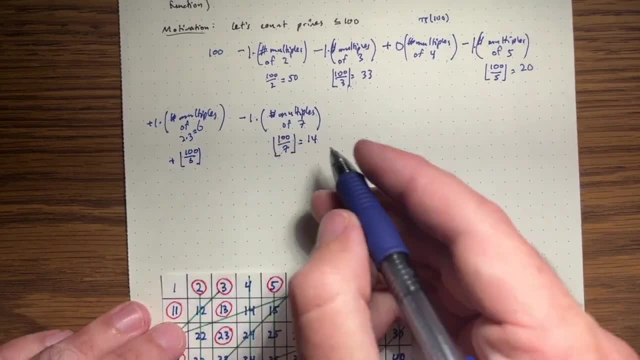 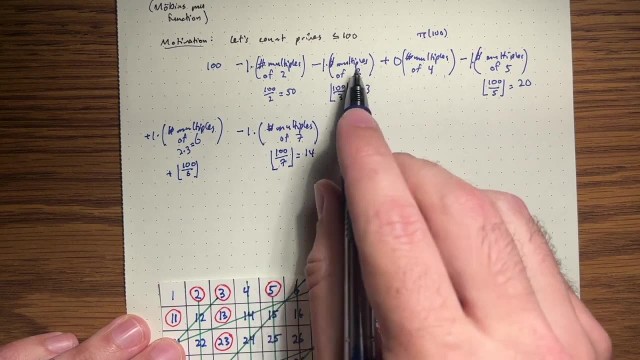 100 over 6.. Multiples of 8: we don't care about because 8 is just the power of 2.. Multiples of 9. Those are entirely just dealt with here. But multiples of 10. See: 10 is 2 times 5.. 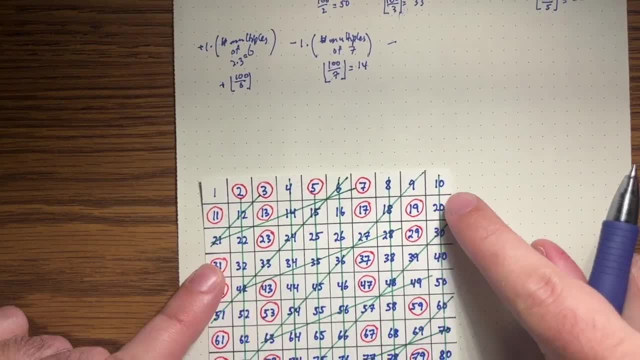 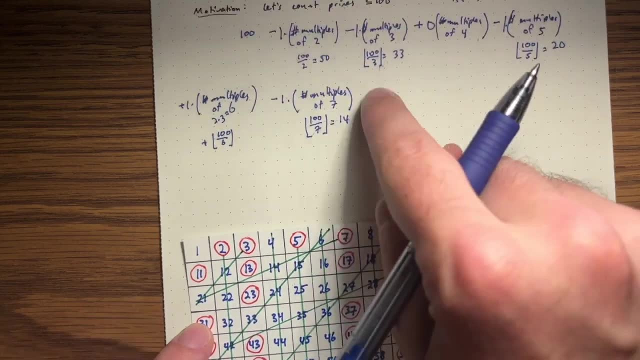 And we have a similar problem with the multiples of 10.. I mean, you can't see it here, but technically I went over this line twice, So I crossed out the multiples of 5.. But they were already crossed out when I crossed out the multiples of 2.. 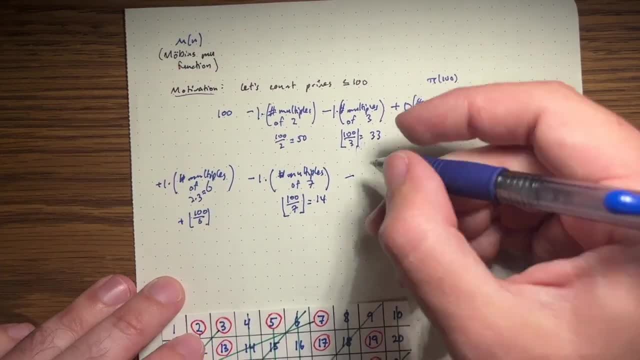 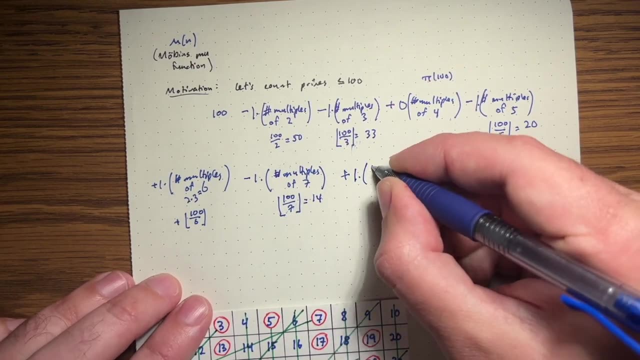 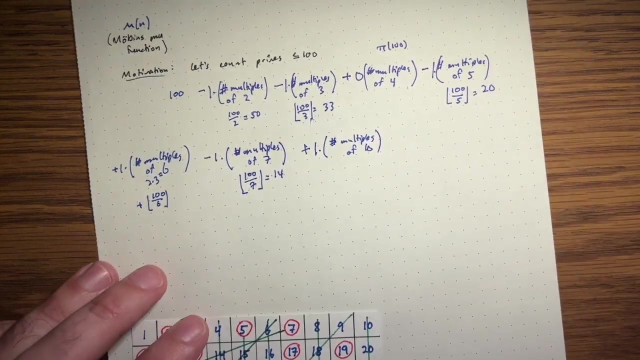 And here in my equation they're actually counted for here and here. So I need to. Let's see, I subtracted them twice, I only wanted to subtract them once. So I need to add them back in And you see, we're getting some kind of weird sum here. 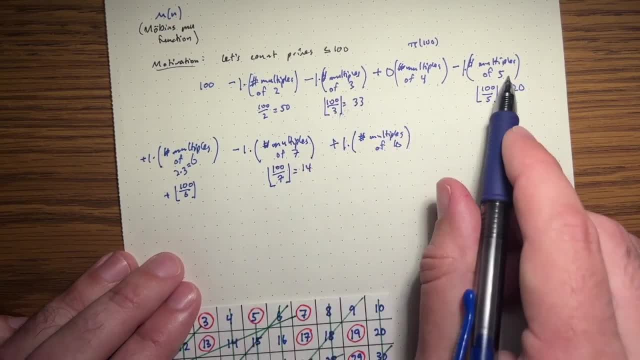 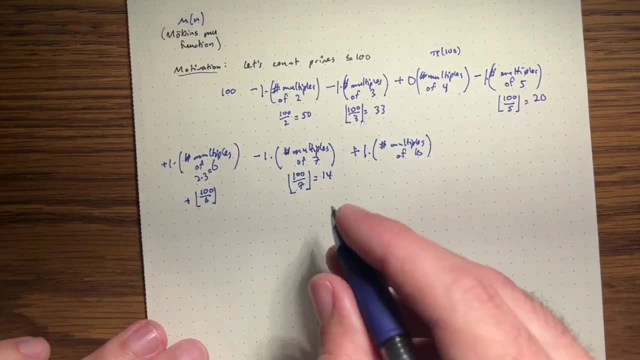 And then you have to keep doing this. So 3 times 5.. So we crossed out the multiples of 15 too many times. We need to add them back in. So this is looking kind of mysterious, Like what coefficients we have here. 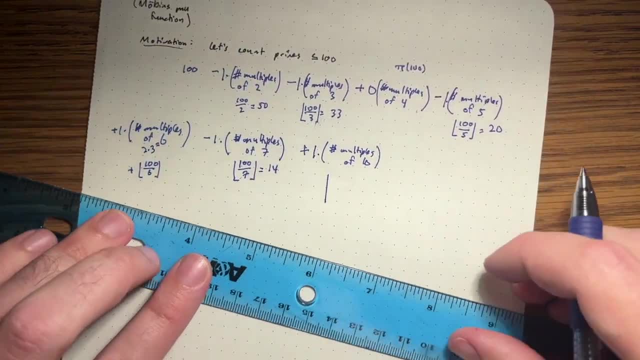 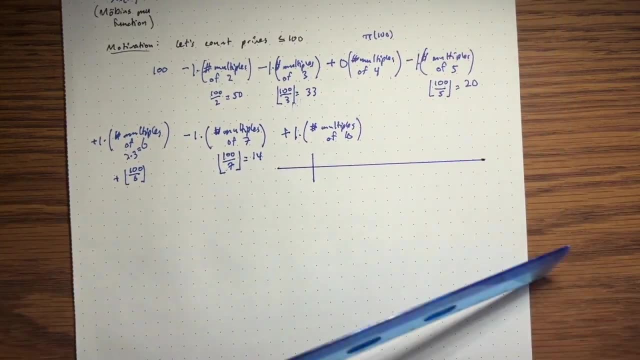 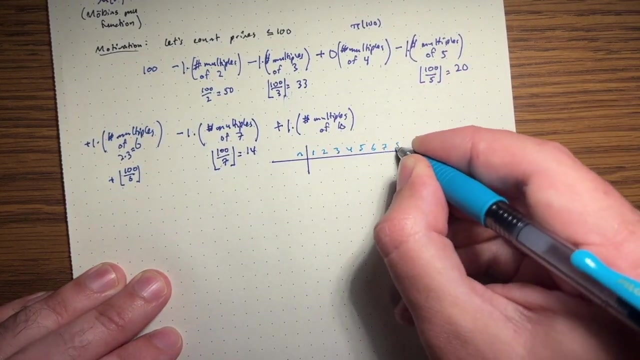 But I'm just going to write down the coefficients that we're getting here. So, in other words, when I'm dealing with multiples of d for some divisor, Let's call it n. So n would be 1, 2, 3,, 4,, 5,, 6,, 7,, 8,, 9,, 10.. 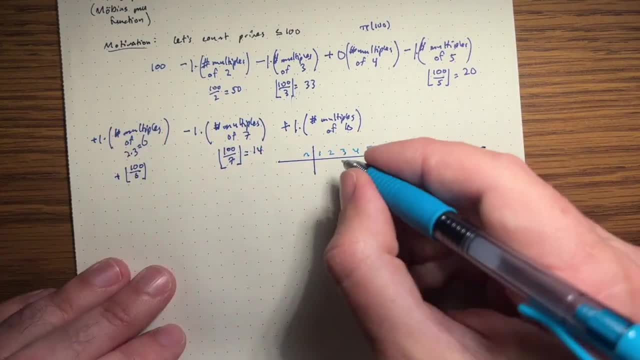 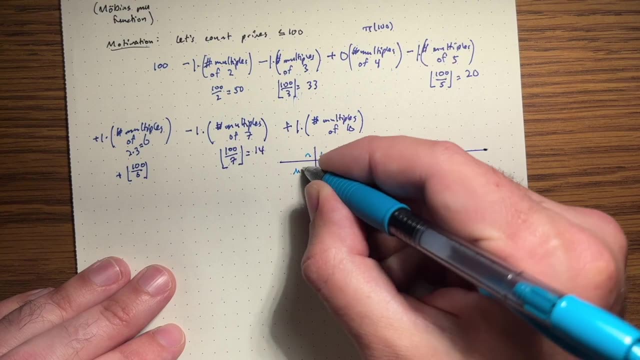 I'm not going to write this whole number, I just care about the coefficient. So I guess this we can think of as 1 times 100.. So my coefficient is 1.. I'm going to call that coefficient mu of n, by the way. 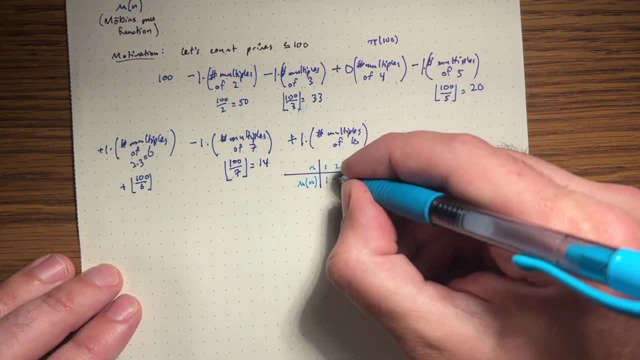 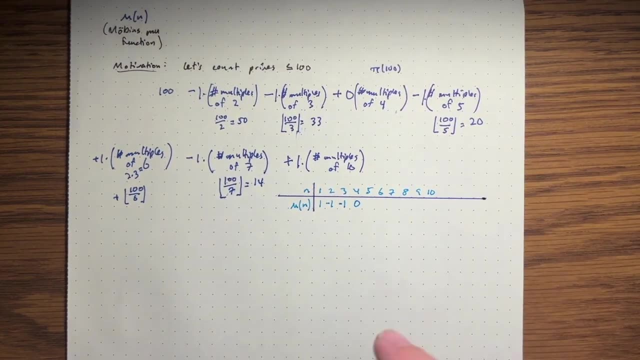 When n is 2.. So we need to subtract out the multiples of 2.. So I have a minus 1.. I have a minus 1 on this term. I have a 0 on this term because it wasn't giving us anything new. 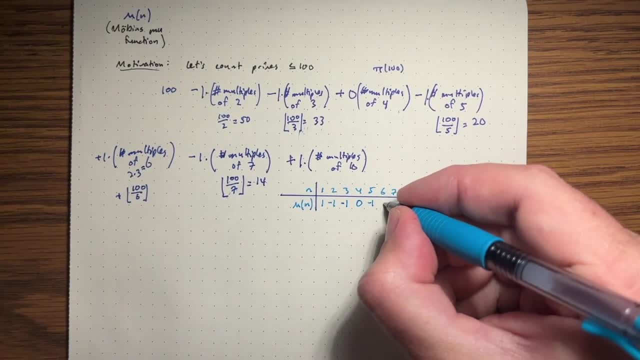 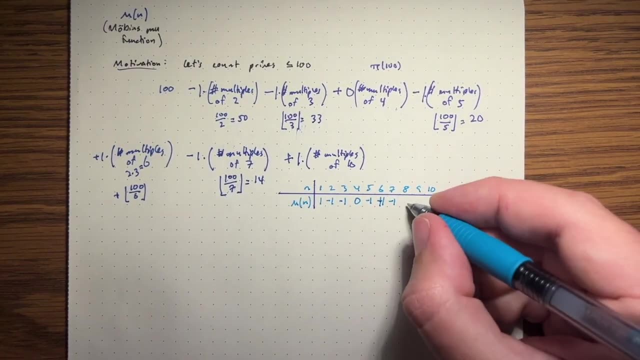 I have a minus 1 here. I have a plus 1 on the 6.. So this is plus 1.. With a 7, I have a minus 1.. The 8 and the 9: we decided wasn't giving us anything new. 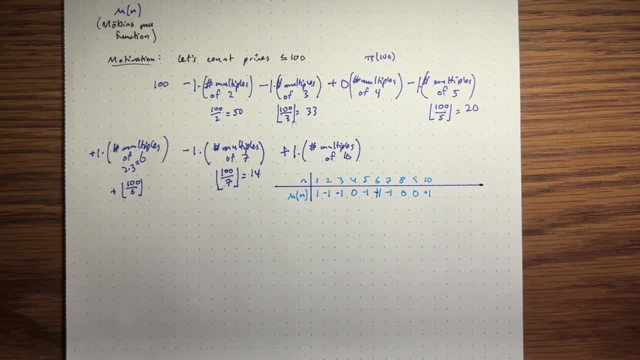 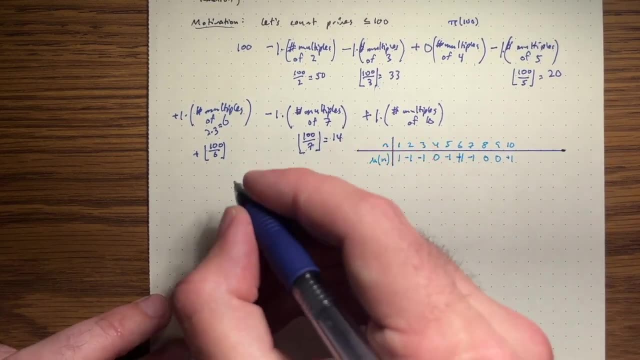 With a 10, I have a plus 1.. And you can kind of keep going with this. For example, if we're doing something kind of funny here, we subtracted off the multiples of 2,, the multiples of 3,. 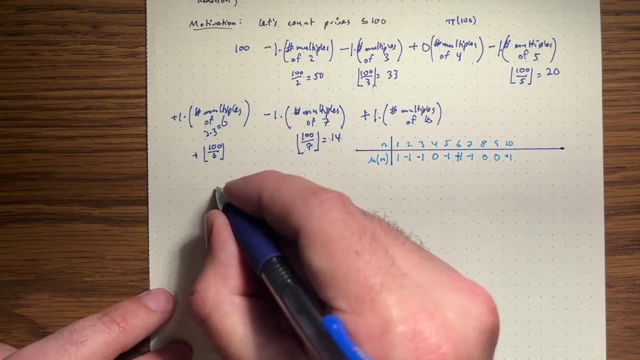 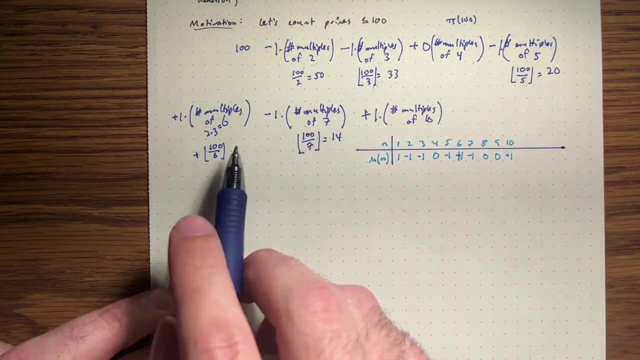 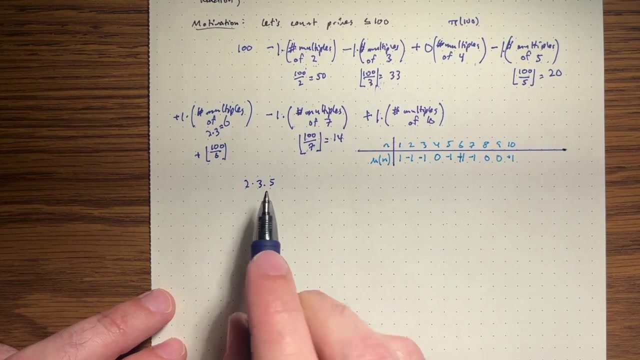 the multiples of 5.. We added back in all the multiples of 2 times 3,, all the multiples of 2 times 5, and all the multiples of 3 times 5.. But what about the multiples of 2 times 3 times 5?? 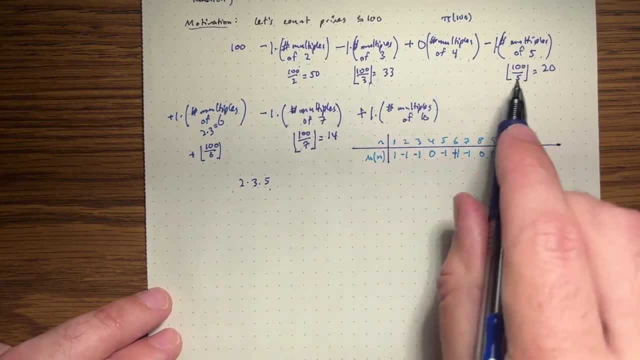 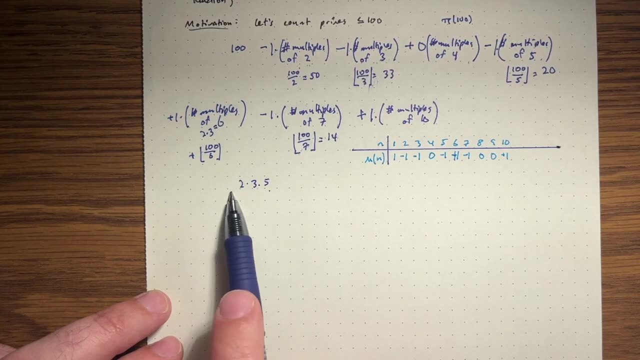 So we subtracted these off 3 times. We're adding them back in 3 times Here here and we have the term for 15.. But we want to get rid of those, So I need to subtract these out an additional time. 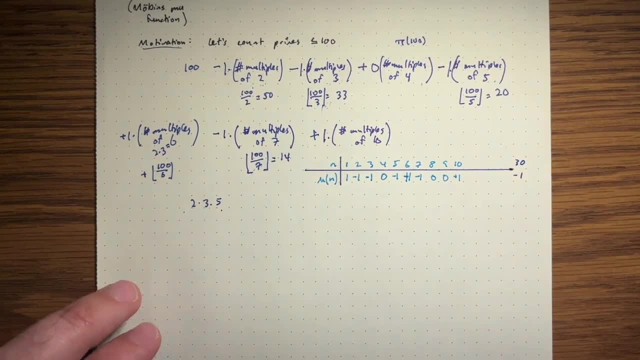 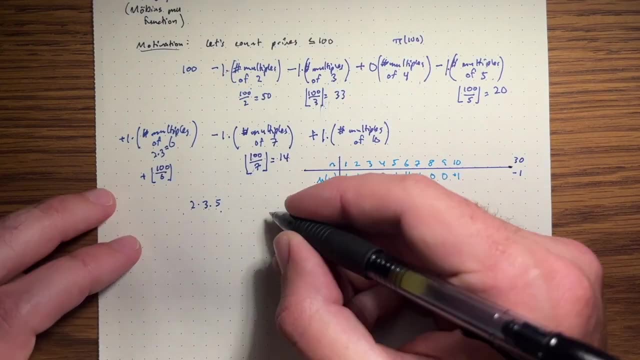 So if I go all the way up to 30, we're going to have a minus 1.. And essentially what we're doing here is this is a constant. you might have seen before. This is called the principle of inclusion-exclusion- Inclusion-exclusion. 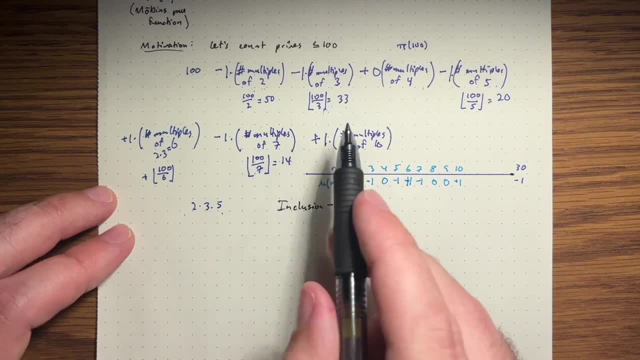 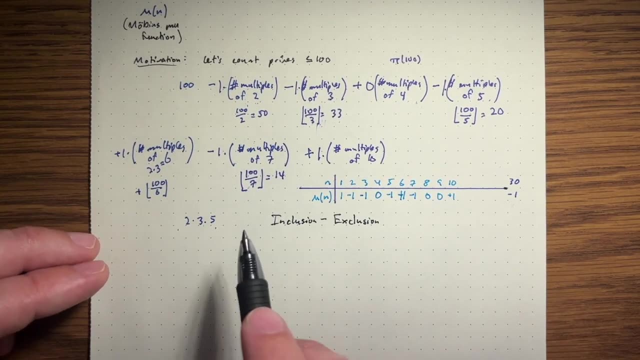 It's where you realize you're sort of double-counting certain things and then you try to add them back in. But then you add too many things back in and you need to take things back out again. But that's the idea. 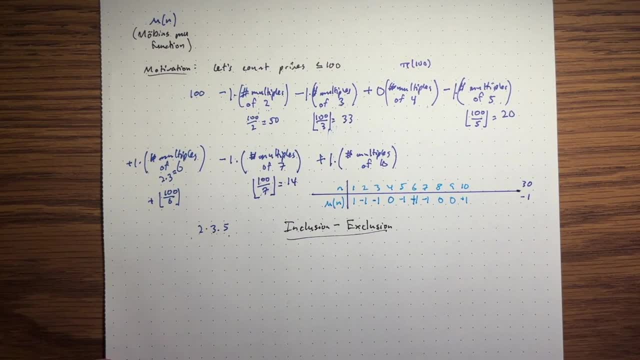 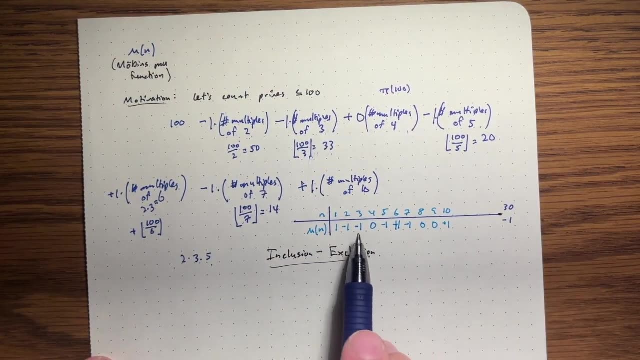 We can in theory write a sum like this, but we have to be very careful about it And it turns out these coefficients here are. they form a very interesting multiplicative function, even called the Mobius mu function. And to really define this, 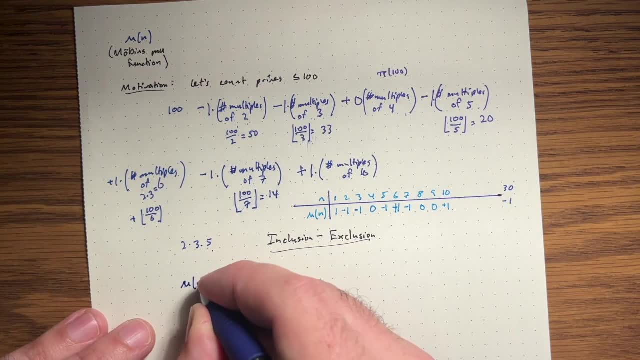 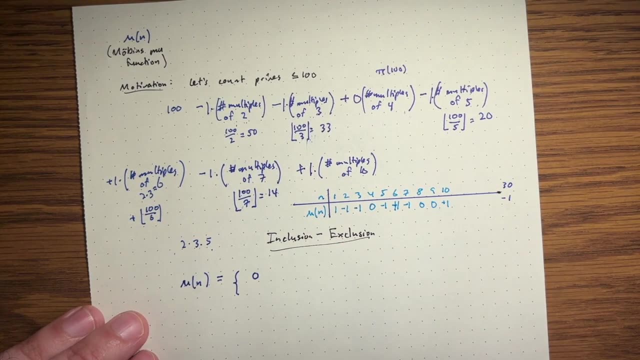 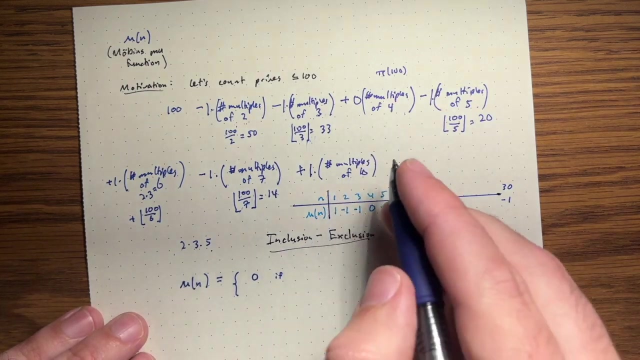 so now I'm going to define this, but the definition might make a little more sense now that we saw where it came from. So first of all I'm going to say it's 0 if we don't really get anything new. So we have a square here. 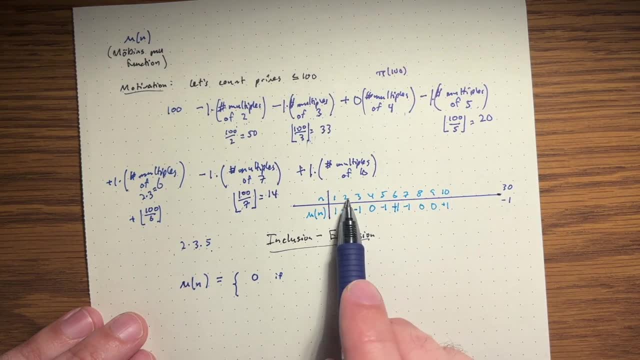 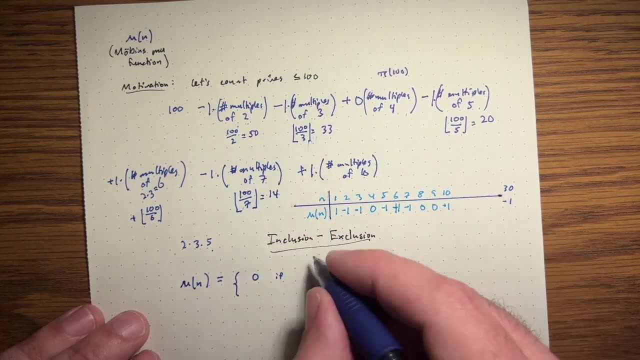 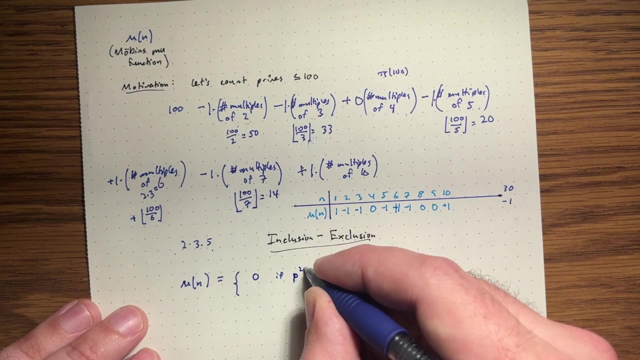 we have a third power of the 8. Essentially, the condition you want is you want you want to ignore the multiple if your number is not square for you, if it's divisible by some square, so if some square divides n, and in fact you can even say it's the square of a prime. 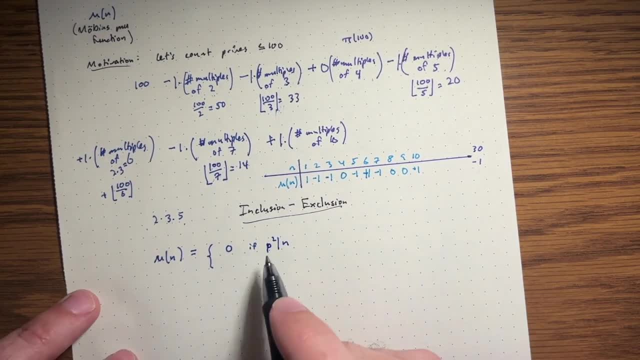 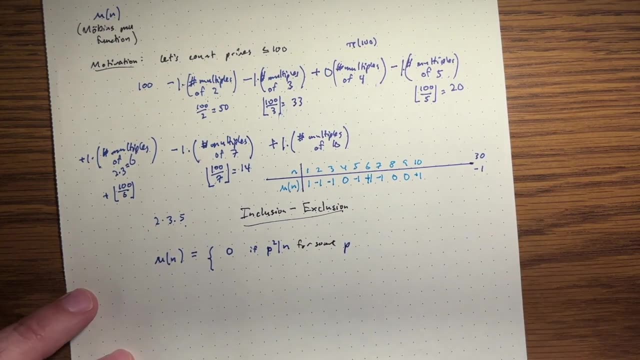 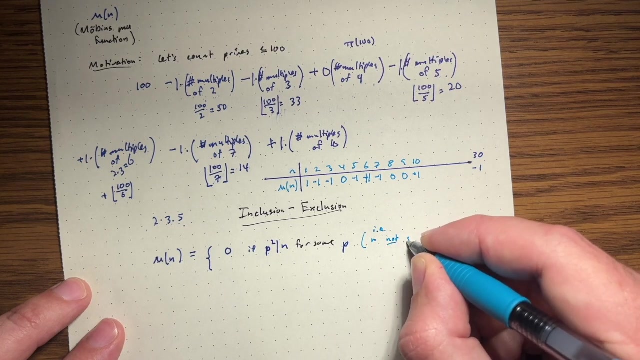 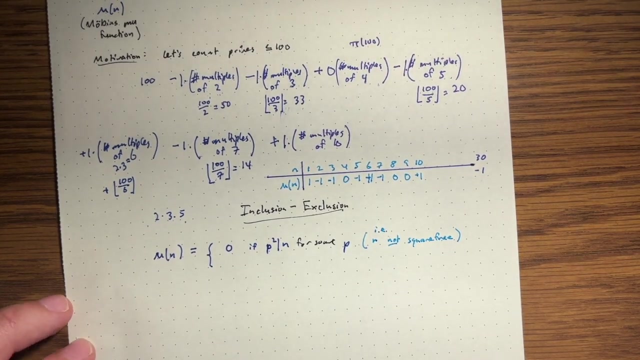 because if a square divides n, then take one of its prime factors. So if p divides n, for some p, in other words a sort of mathematical term- would be. so ie, n is not square for you square free. square free means that no square divides your number. 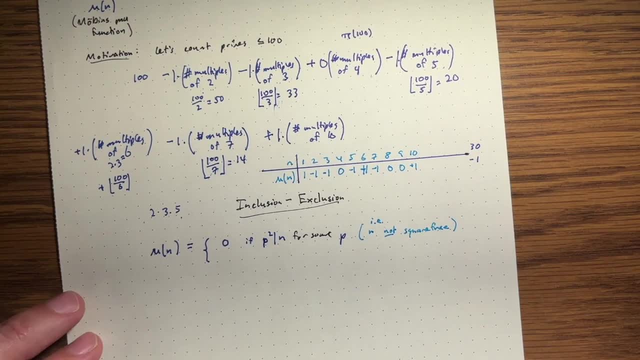 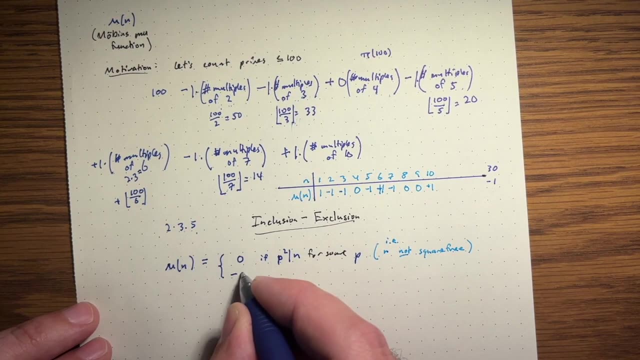 Yeah, 0 if there's any square whatsoever that divides your number, except for 1.. But yeah, 1 is not prime. And then this is the part of the formula that's going to look weird: it's going to be a negative 1 to some power here. 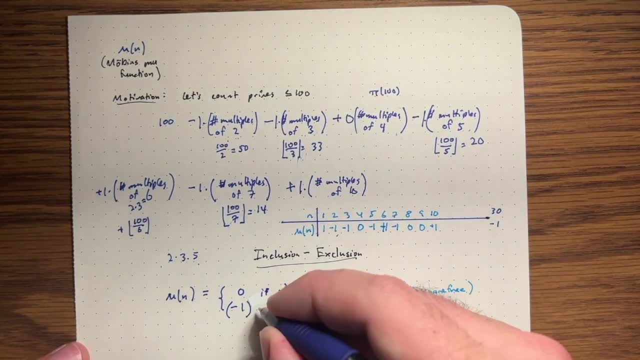 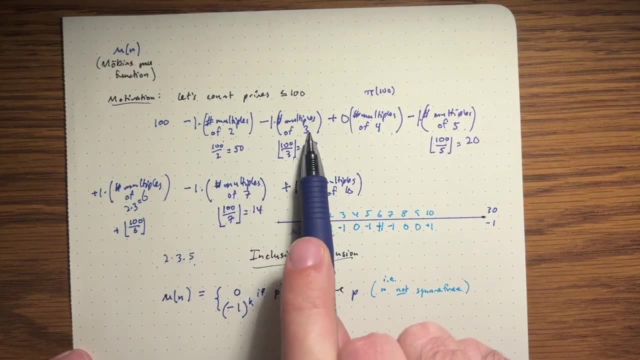 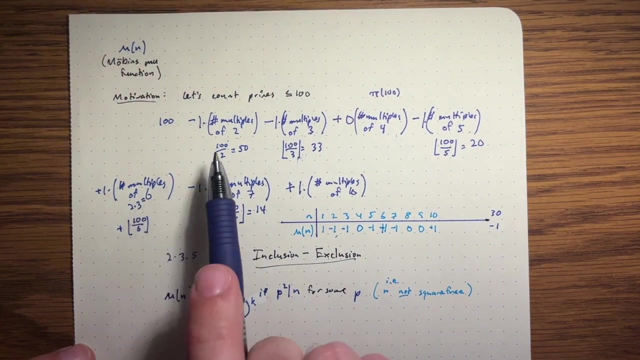 Okay. so what is this power going to be? It's going to be okay, so essentially it's going to be the number of primes in my factorization. So here, 6 was 2 times 3, so that case was already covered by the cases for 2 and 3,. 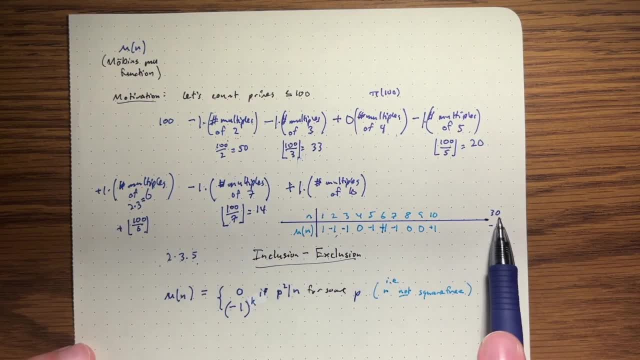 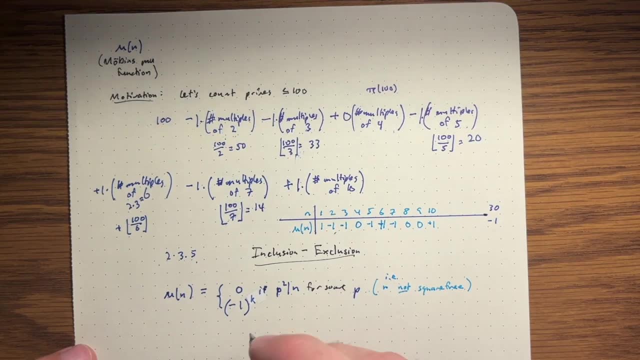 so we want to flip the sign, But then for 30, we wanted to do a minus 1 again, because that's 2 times 3 times 5.. And it turns out you want to continue this pattern. So if yeah, this will be in the case where n.